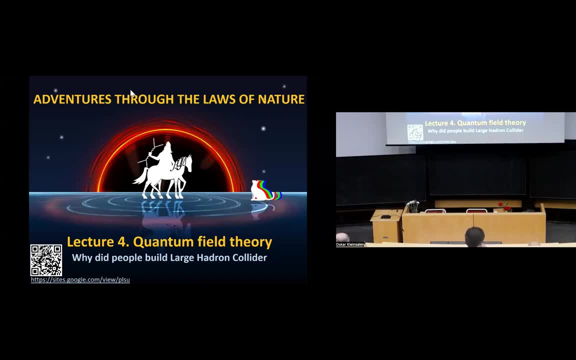 Welcome everybody. So today we continue our series of lectures, Adventures through the Laws of Nature. We have Dmytro Volin that will speak about quantum field theory. Hello everyone, You can hear me well Good, Today we finally go beyond what is usually discussed on forums about quantum mechanics and do a little bit closer to modern times. 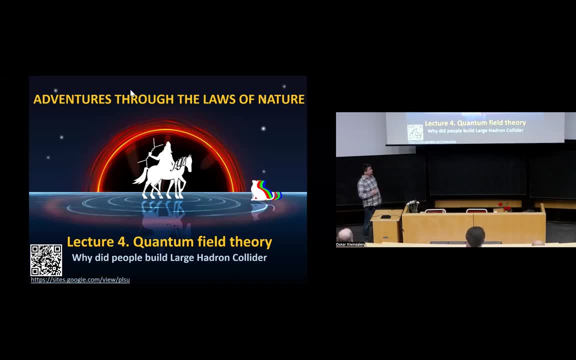 But yet we still have to go to the past first. We start by asking Google what is the biggest machine built by humans? And Google actually tells us, will tell us- I checked it- that Wal Guinness said it is LHC, Large Hadron Euclidean. 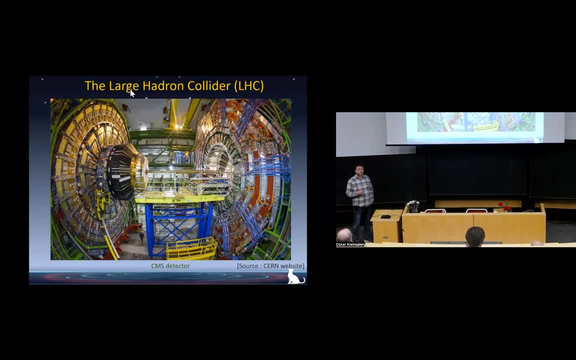 And I kind of can agree with this completely, because it's really a very huge machine. Here you can see some part of it. it's quite a small part of it actually. This is a CMS detector, one of the several detectors that we found. 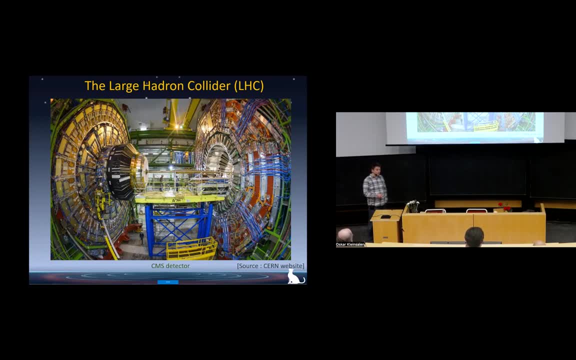 It's a Large Hadron Euclidean And here you can see a human. So most of this actually, if I understand correctly, are detectors that will detect different particles and metallic stuff Like here are some electronic equipment which collect data And there are some wires which will bring data to the computer. 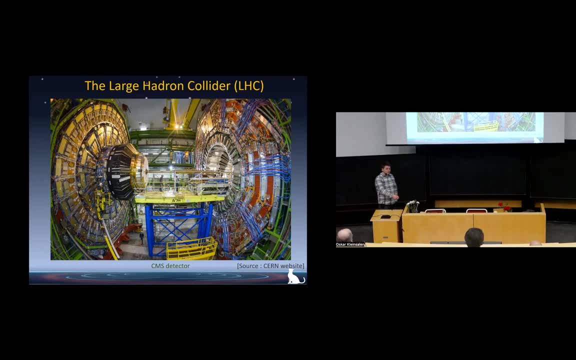 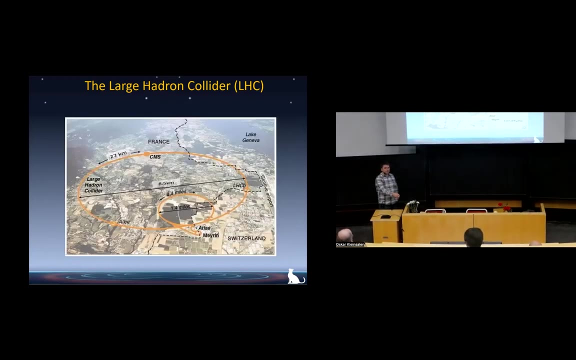 Roughly it's like this, But it's just a detector which will detect what's happening In this small tube. here, if you can see, The real thing is accelerator itself And it's much bigger. So our detector, which we discussed, was here. 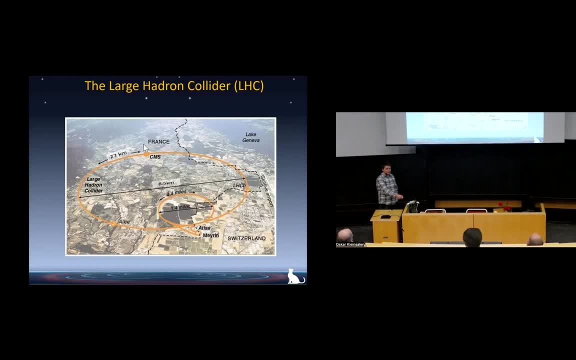 It's a big building inside of which you have the detector, And the machine itself is 27 kilometers in circumference. It actually doesn't fit in well. It's partially in France, Most of it, And some part of it is in Switzerland. 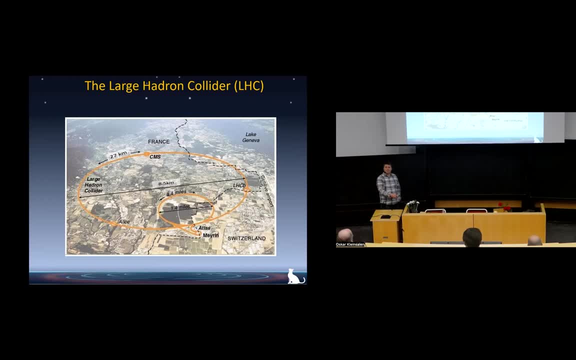 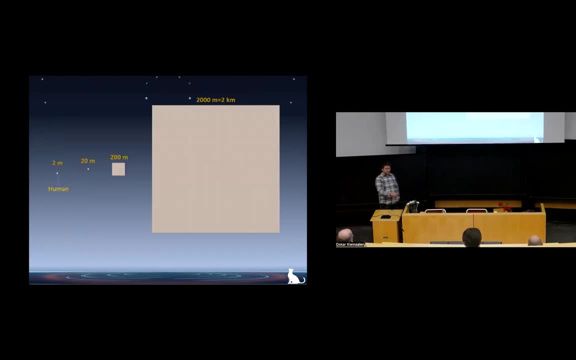 It's situated close to the Geneva city And in diameter it's 8.5 kilometers. In the very first lecture we were discussing scales And I remind you that this pixel here actually is a little bit less than a pixel in the size of a human. 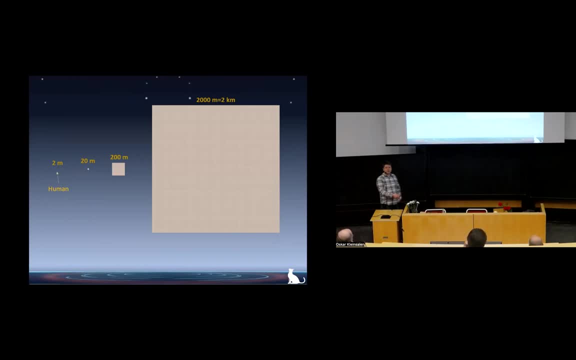 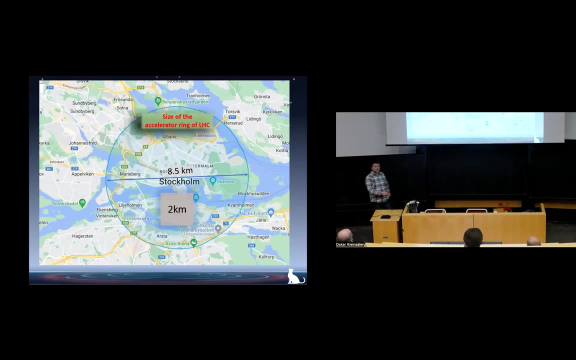 And then if it's the size of a human, this will be the size of 2 kilometers wide. Now, if you make 2 kilometers wide on the real map, It will be the size of Gamla Stan in Stockholm, And then up to scale, we put a big ring of accelerator LHC. 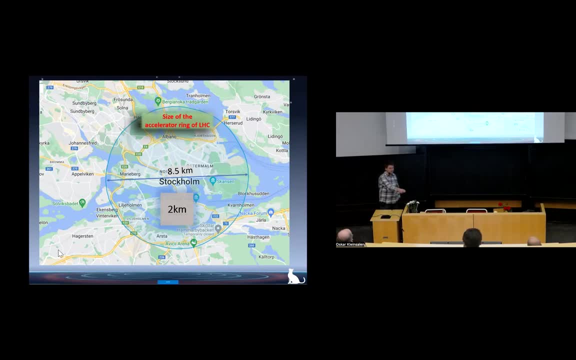 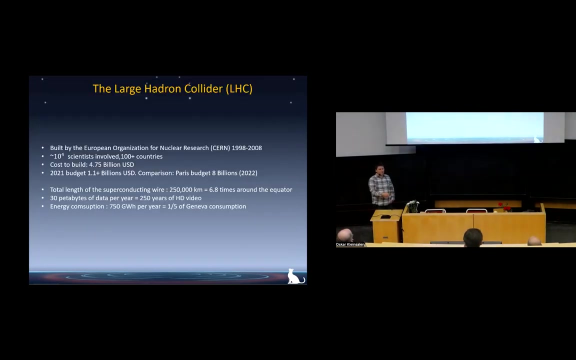 It will be roughly corresponding. It's actually interesting because it's quite well fits E20 highway, which goes around Stockholm. So this is how big the machine is. It took 10 years to build it. There are about 10,000 scientists working. 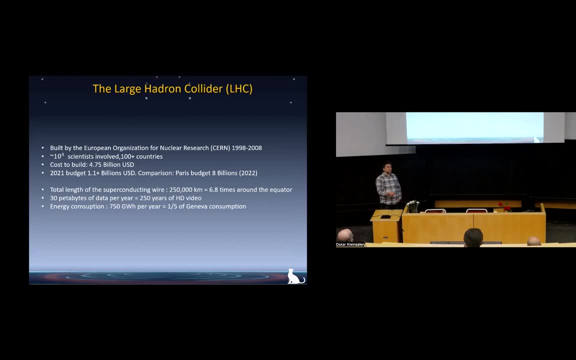 And more than 100 countries participate in contributing money for its operation. Its budget is almost 5 billion. Not budget but cost of construction was 5 billion American dollars roughly And every year budget is about 1 billion dollars. It can be compared to our budget of Paris which is 8 billion last year. 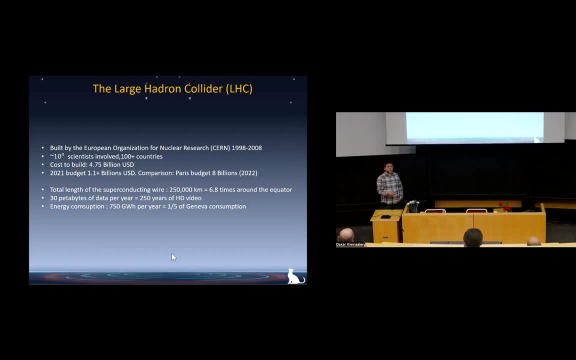 It has very many superconducting wires in it And actually it's 250,000 kilometers. Well, you can see it seven times around the equator. And this is not just wires, It's superconducting wires. I imagine nothing else was required that many wires. 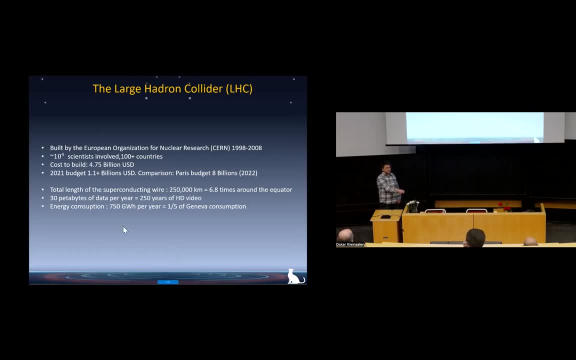 That's how many. you also see how many data It accumulates. It's 30 petabytes of data per year In reality, actually all the information, which is one petabyte per second. It's just too much to store. 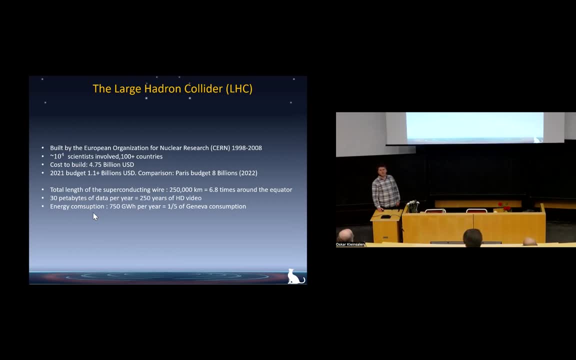 And they throw away most of it and keep on a little bit. Still. it's 30 petabytes per year And energy consumption is one-fifth of Geneva consumption And it's averaged over a year, But it's operating actually quite high. 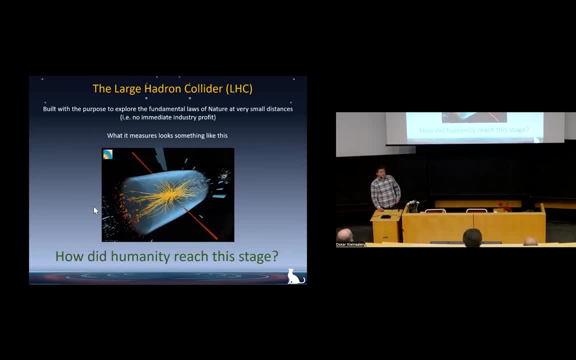 So this is how big it is And what it is for. To study these crazy pictures which nobody meaningfully understands what's going on, It requires analysis And finally, I want to notice that this machine was built for the sole purpose of natural exploration. 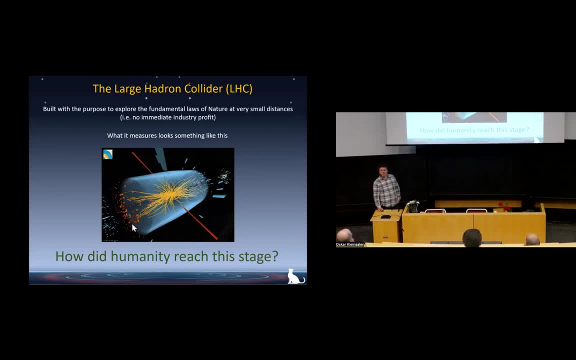 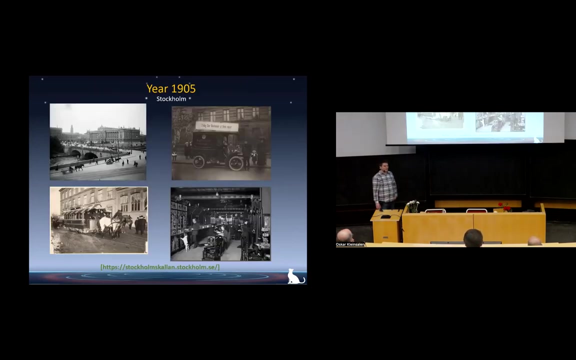 It has no immediate industrial application- Maybe in the future, But not now. So it's a huge thing And the question you should try to understand: how did humanity reach the stage of building such a monster? I decided to go back more than 100 years, to the year 1905.. 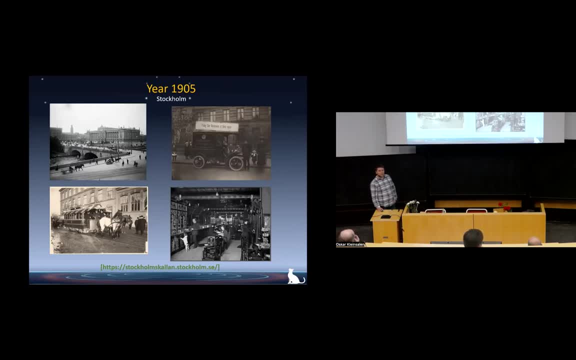 In the year 1905, I found several pictures of Stockholm. So I understand this is the royal palace And so there are some horses pulling carriages. You see actually here some rails. So first of all, the tramway was there. 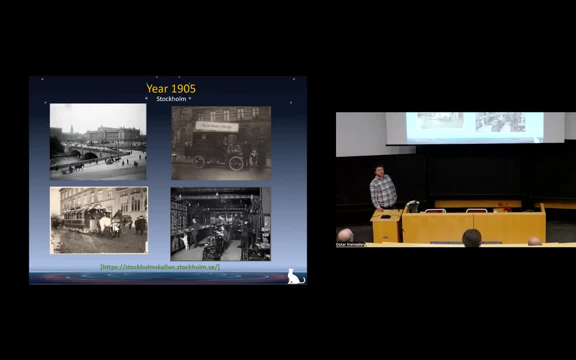 But in reality the tramway was pulled by horses, Although on the picture it was said that it's the last tramway pulled by horses. After that they actually changed and made it electric Or maybe steam power. I mean diesel power. 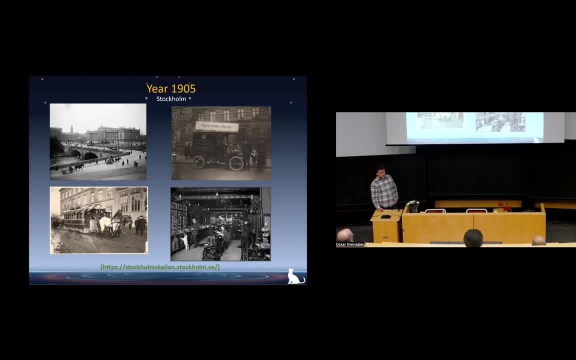 And there were already cars, And in restaurants people were wearing all these nice dresses, Not like we are today. It was much more elegant, But this already was a buffet. This was not like served food. So this is how life looked like more than 100 years ago. 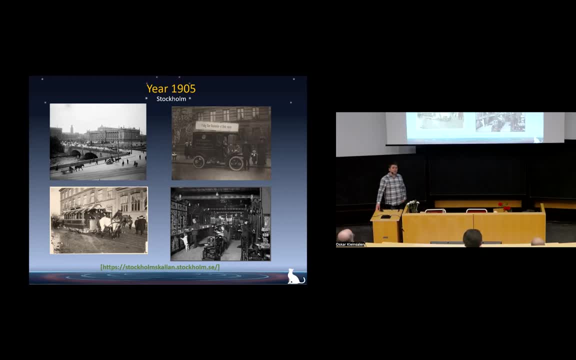 Starting to become a little bit familiar to the modern life, But still quite different. But also I want to notice that now it's about 50 years that industrial revolution has happened And this means that production by humanity changed completely How it's done. 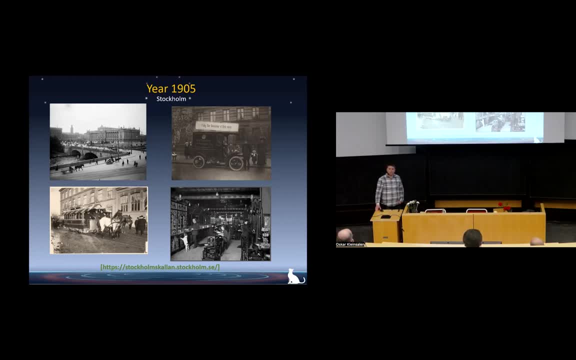 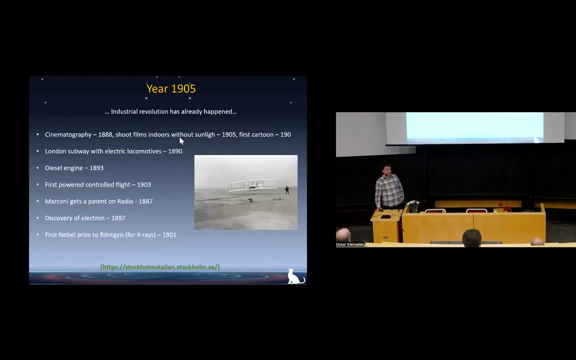 And scientists in particular, got access to completely new type of technologies And this led to many different discoveries. Let us see what happens prior to 1905.. A few years, like a maximum 20, 25 years before. So cinematography was discovered about 20 years before. 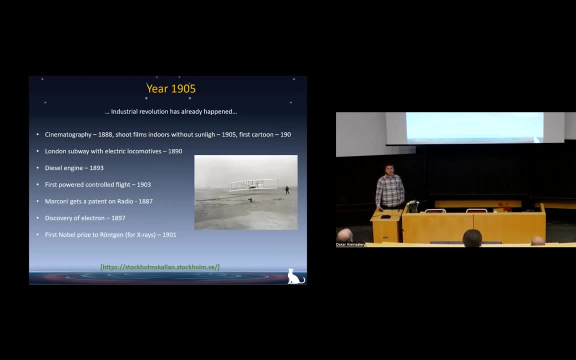 And 1905 was the year when they started to film inside the doors without the usage of sunlight. So they completely changed the level of exposure they required. This is 1906.. I don't know when it disappeared, But the first cartoon was made in 1906. 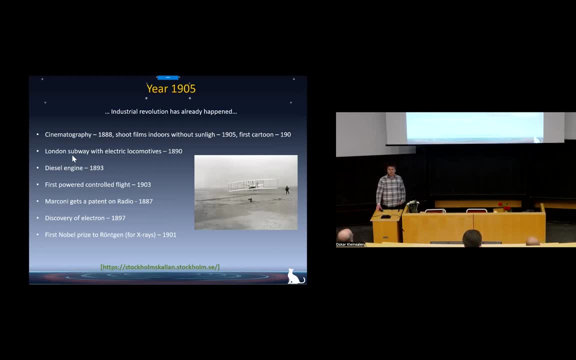 I'll show you horses. But in reality people already knew electricity very well And London some way started to operate electric locomotives in 1890.. 15 years before 1905.. Diesel engine, the one which is used in cars these days, started operating in 1893.. 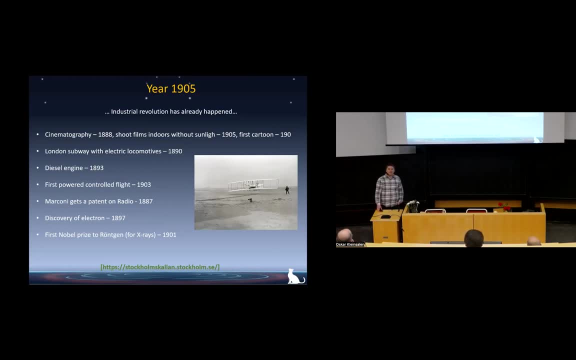 Brothers Wright launched first controlled powered heavier than air flight, And I want to notice that mathematics behind the fact that airplane can fly was known for more than 100 years. People just concluded that we do not have technology for designing powerful and enough and light enough engines. 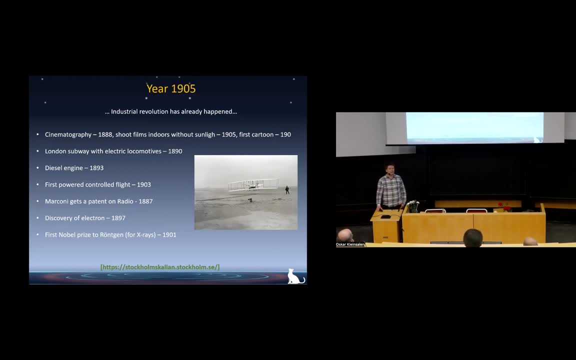 So we have to wait. And so the time came And special engine was designed. But anyway, Brothers Wright did not claim that they designed a good engine. What they did, they designed a good control system to control the flight. This was a real contribution to the flight. 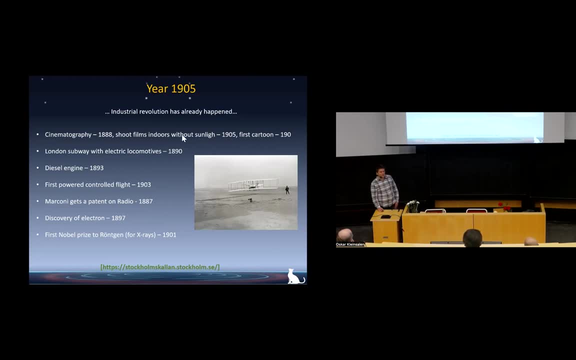 Anyway, this happened roughly the same time we're speaking about. We have a radio already patented. There are many radio styles before Marconi, But this is when it was become popular. In physics, electron was discovered not so long time ago. 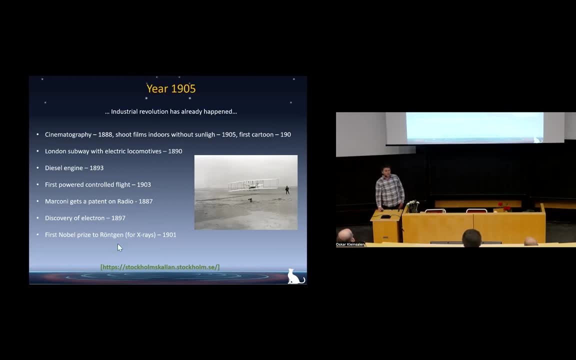 And Nobel Prize started running in 1901.. So actually Röntgen discovered X-rays in 1896. And 1901 is just the first Nobel Prize that was awarded. So this is roughly the year when New Epoch started And we have most of the discoveries that become more and more well designed in the future. 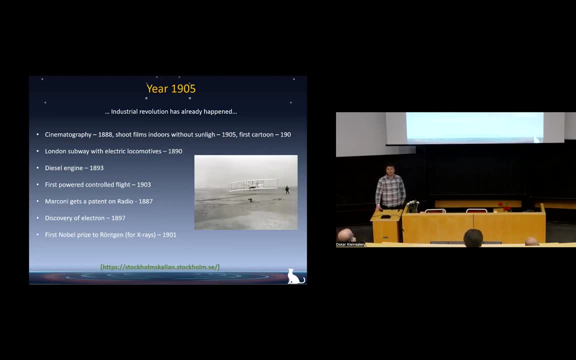 But the ideas and principles of action. If you look on the CRs, I could have chosen maybe last 20 years of the 19th century, But I chose the CR for a very specific reason: Because in this year it's called Miraculous Year. 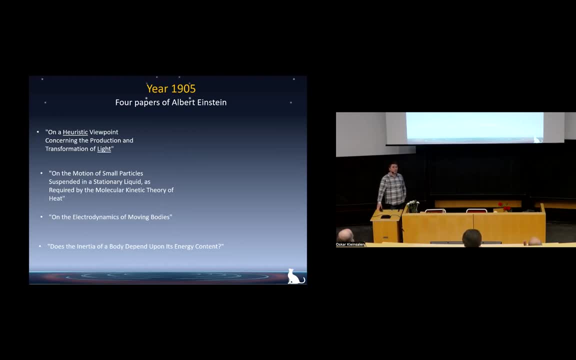 When Albert Einstein published not one but four papers- And let us make a quiz. So there are actually four formulas. When I was reviewing my slides- And I was reviewing my slides- I realized I actually made some mistakes. The square root is not here. 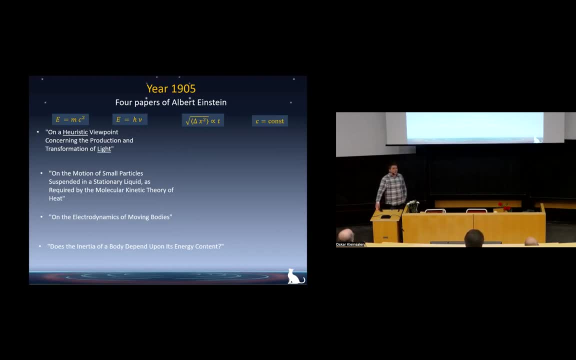 But otherwise it's okay. And so let's play a game. Can you tell which formula corresponds to which paper? So, first paper, it's called on the heuristic viewpoint concerning the production and transformation of light. Which formula goes there? This one: 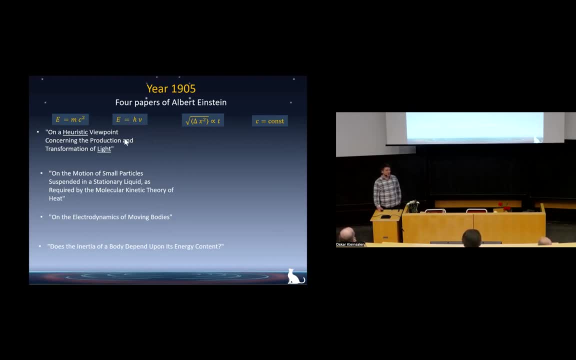 Yeah, So this is actually the paper for which Einstein was awarded the Nobel Prize. It's about explanation of photoelectric effect When he used Planck idea that energy is transferred in quant to proportional equal to Planck constant and frequency of light. So he actually goes here. 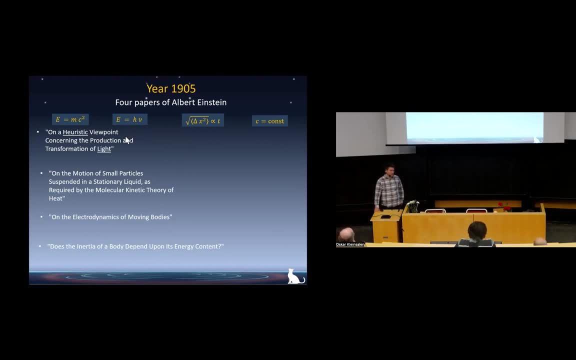 Let's go to the next one, On the motion of small particles suspended in a stationary liquid, as required by the molecular kinetics theory of heat. That's very complicated. title. The third one: Yes, So this is Brownian motion. So he could just write on Brownian motion and it will be clear. 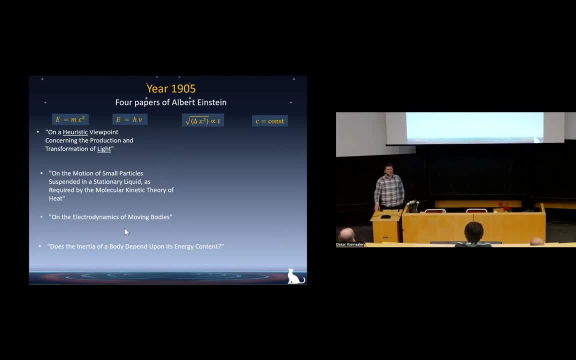 I don't know. I mean, didn't they have this course like efficient paper publication that we like have these days? And then the third one On the electro dynamics of moving bodies. Sasha did the lecture on special relativity last. So it's C equal to constant. 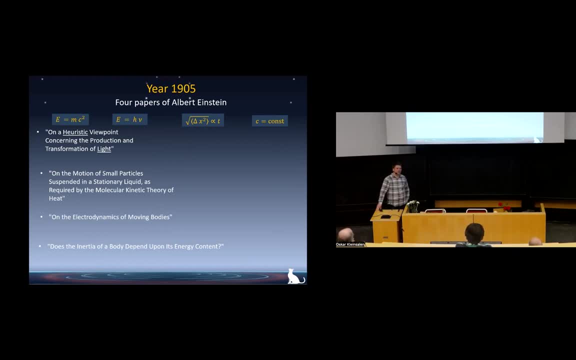 The paper, when I understand that C in constant is one of the laws of nature And it follows from Maxwell equations in particular. In this paper they also have additional velocities formula. I wanted to write it, But then I know it's kind of funny. 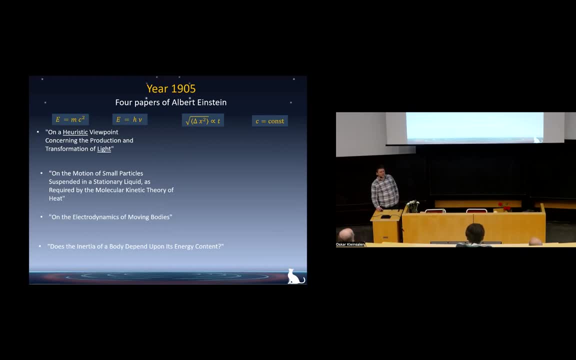 It's kind of too much, too long formula, So let's, let's pick it up. And finally, the last one: Does the inertia of the board depend upon its energy content? Well, this is famous equal MC square, But, as we learned last time, this photo was not written there. 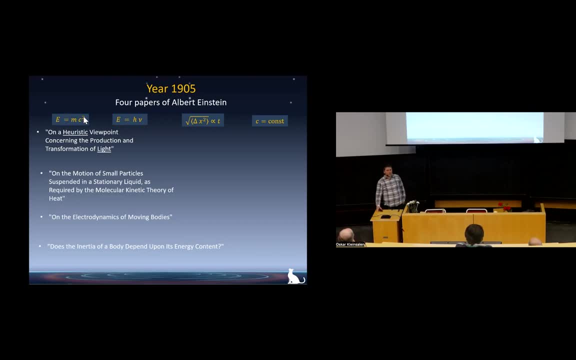 In reality it was equal Delta E, equal beta M, square Roughly. And and also, All this for formulas is very important, Very important formulas for modern science. But don't think that each 10 invented. There were quite a few papers before him. 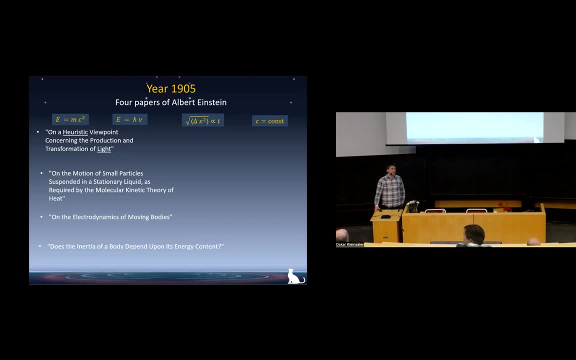 Which content a lot of very useful ideas, And we can debate whether he was actually the first to write. I didn't want to divide it today, But notice, I'm not very good at history of science, But I'm doing science myself. 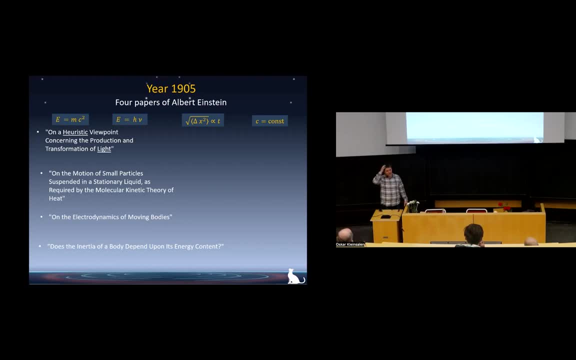 It's not like one person sits down things and discovers. Process is much more complex. It takes many years And a lot of people in community Contribute these different ideas And somehow it evolves. Eventually, face transition happens And suddenly we understand. 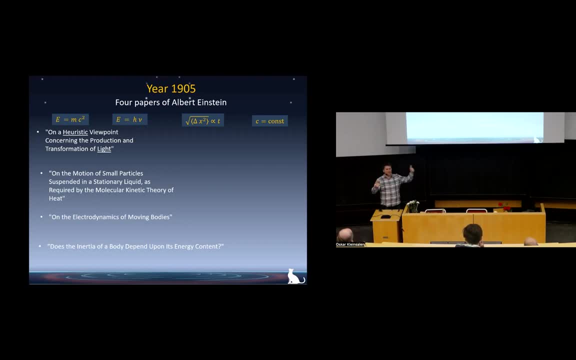 And the person who actually happened to be on this. Yeah, he gets the credit, But there are very many people around just before, just after Who contribute really important Knowledge And if you look at the papers around this year, All this ideas. 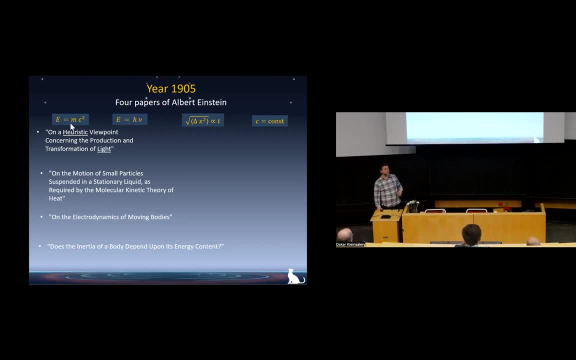 They're present in many papers. This forum like this: It's for the electromagnetic radiation, before And state Is it? Is it See people to constant false follow Related to Electromagnetism? And, for instance, you know what is this? 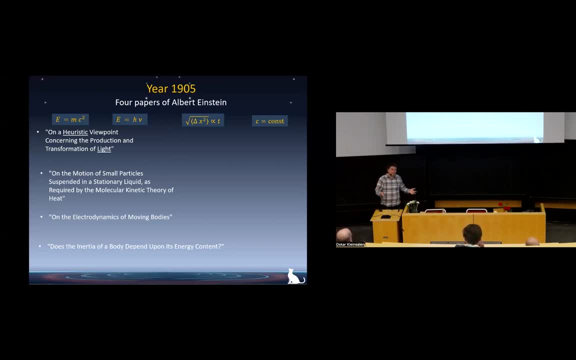 Something is called Lawrence construction, It's not called. It's called Lawrence For the reasons that Lawrence knew it before and stay, And so on This formula. I checked Wikipedia before. This formula appeared first time in the analysis of stock markets. 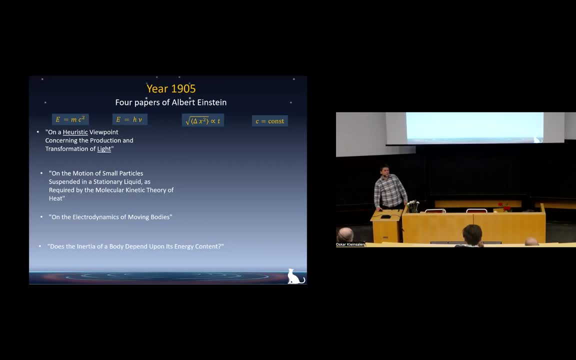 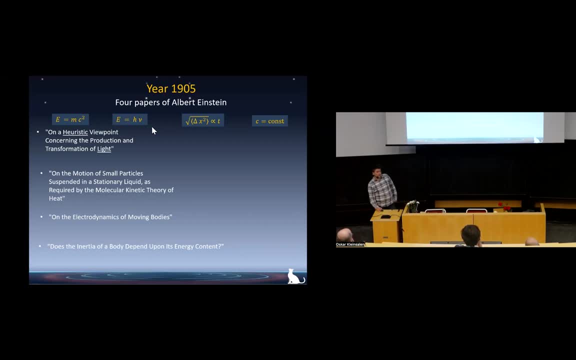 After good, correctly, Stock markets is another stochastic system. It's also that Right And this formula Formally usually Second paper. Except He did not say It's light, exchange of energy happens with this amount and instead say no, okay, exchange happened this amount. 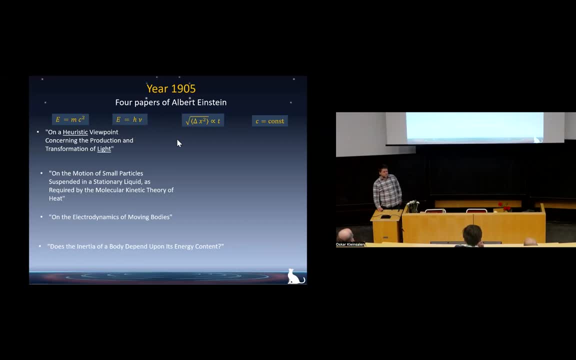 but also light, have this minimal amount. uh, all these formulas will happen to be important today. that's why i chose them this year, and papers of einstein, and i will start with brownian motion, as was i say in order. uh, because brownian motion? uh, it's about big particle moving in this way. 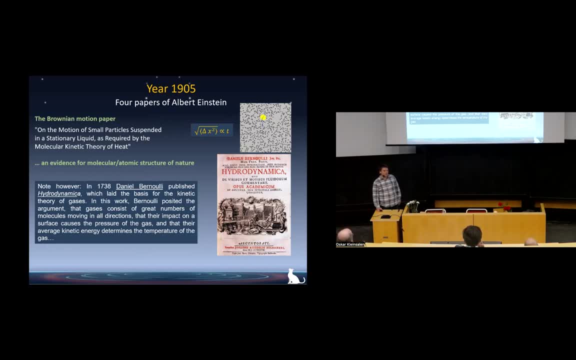 many other small particles. they push it around, so it's a very complicated movement. it was considered as an evidence for molecular, molecular or atomic structure of nature. uh, and i i cannot still have been surprised, because 1738 bernoulli already say: okay, we have too many molecules. 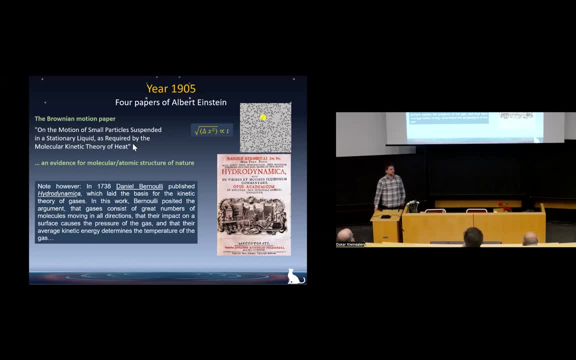 move chaotically, moreover kinetic, and more energy of them is temperature. he said it. i mean 1738 and, and in 19th century kinetic theory of gases and maximum distribution was known. it's common legend. i don't know if it's true that max will derive it on his example. 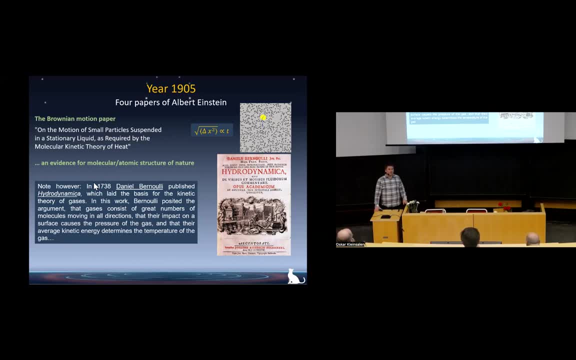 uh, for gradation, uh, i i mean. so i i'm sure that quite a few physicists actually did believe in atoms, but until this kind of years, there are very, quite a few people who did not. uh, it's come back to the story, which i could keep repeating, that it's very hard to believe that the 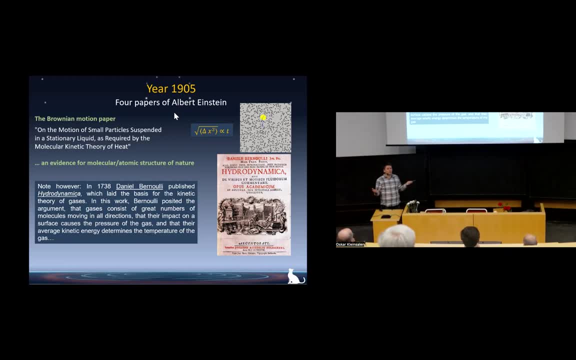 matter that we have here, becoming very different, will become small and many could not accept it, i presume. but after this it was quite accepted. and why are coming to the idea of atoms? because what we are going to do today, all the day, we are going to ask the question: what is inside, what is inside? what is inside? so i can take a chalk. 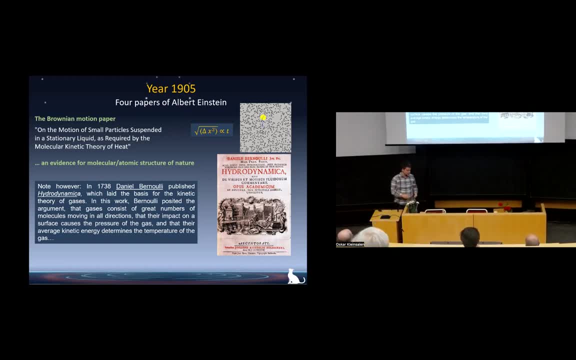 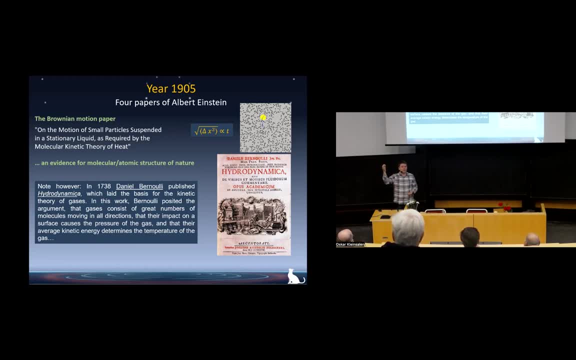 actually there are 10 to the power, 23 molecules here, or atoms, it's, it's, it's a huge number, but if you divide by two it's not that long that you uh get out or get rid of molecules. uh, important things happens when you get to the size of the. 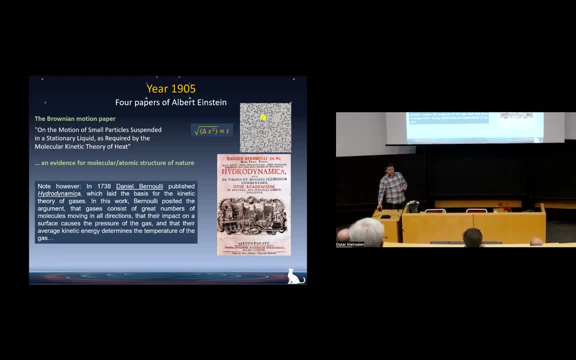 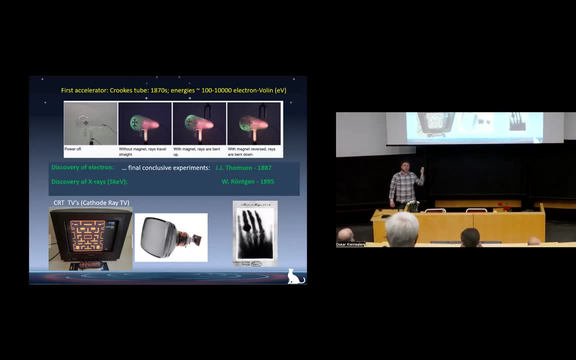 molecule, and that's why i brought it to the idea that molecules do this, because what will happen next is: we are going to discuss what will happen next. uh, happen next in ionization, and this is conceptually nonsense. new happens until you get to molecule size. everything is that electrically, not. 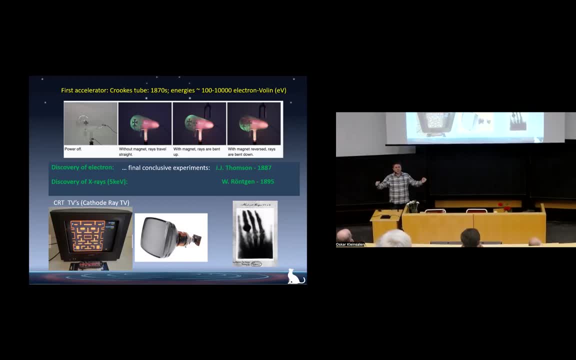 but when you break, well, molecule still breaks into atoms, atoms still electrically neutral. but when you start to break atoms, it's completely new situation. you have positive nucleus and negative electron. this is already different. feature like seriously different, and understanding that there is this positive, negative charges explicitly. uh, this is what i want to discuss now, because 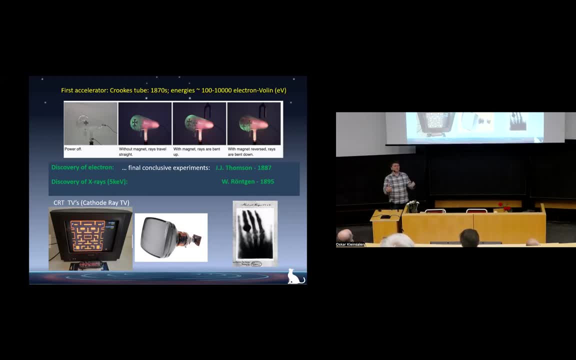 what i want? i want to show you the very first accelerator, so basically this old style tv which is called cathode trade tube. so the rt is for tube. actually, this tube here, this is, uh, ancestor of the first accelerator used by humanity. this first accelerator is for humanity, it's called crook's tube. 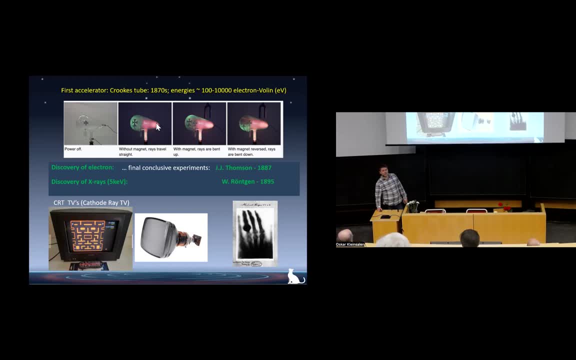 the idea that you have here an image emitter of electrons and there is some another like change of potential, and electrons just couldn't accelerate it and they start to bombard something. i mean the first thing, not even discuss what they bombard, but just appreciate their existence. this tube was used by thompson to discover electron. 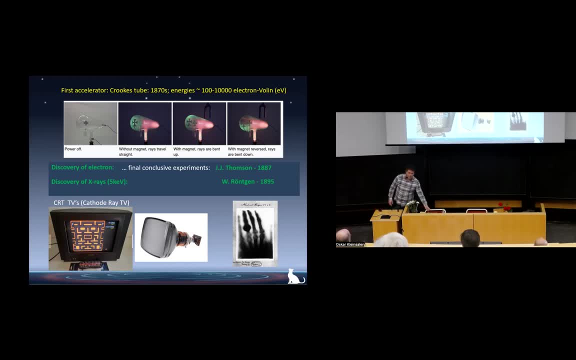 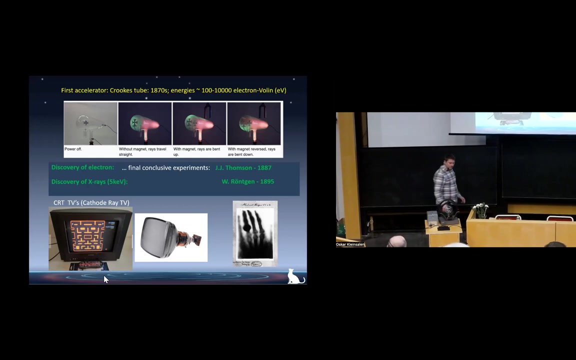 uh, well, so we are doing physics, physics, experimental science, and i hope experiment will work. problem with experimental science: it's not always working. um right, so. so this is basically an example of troops tube. it just it doesn't look like two tubes, looks like a ball. well, that's what i found in the lab. uh, so you don't see, see anything until i switch off the. 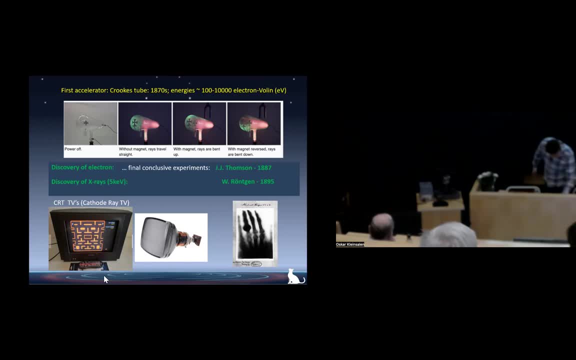 light and you still will not see anything, because i'm waiting that it's gets here. oh, you see, it doesn't work because, uh, because one, yeah, because this went loose, so i switch it on now, really, uh, so now, now it will work. uh, so what's happening here? there is a metal plate, i mean on the, on the break. you can come here. 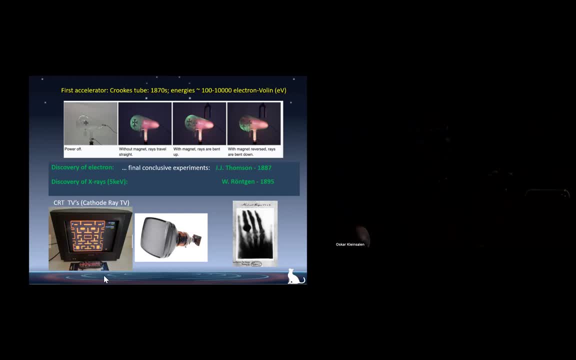 and see for yourself and try yourself. but now explain: there is a metal plate which is getting heated. you probably don't know if you see a little. do you see a red light? yeah, well, anyway, that's not the most important part, uh, but there is some secret, it basically. 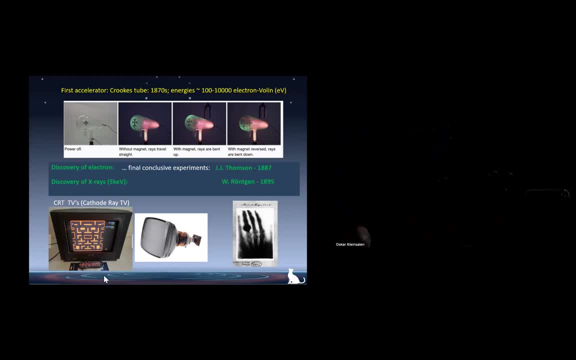 just hit the metal. it helps electron to escape the surface of the metal. and what we are going to do now? we are going to apply a difference of potentials just here. uh, we apply actually 300 volts, so quite a bit like it's like the same similar potential we have in the in the outlet, except 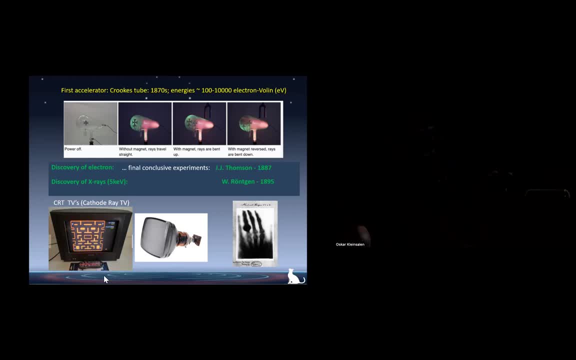 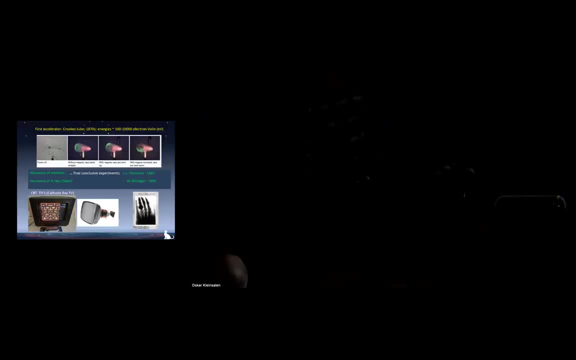 it's, it's stationary current, stationary potential, it's not oscillating, and electrons that emitters are getting uh accelerated, so now, and so now it's about uh 50 to 100 volts and then increase it. okay, so uh, this, this beam here actually is, it's a beam of electrons. 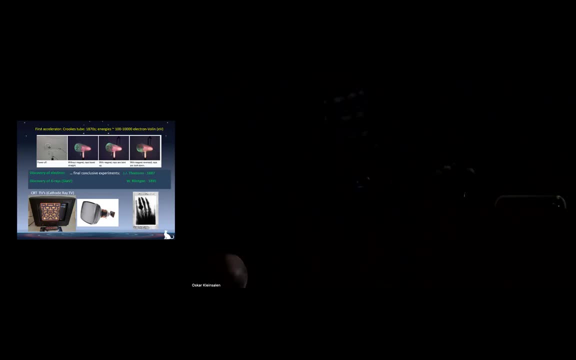 and uh. so the point that's inside it's quite a good vacuum. there are quite a few molecules- uh, just enough to get your nice, and that you can see electrons. if you put just normal air inside, uh, all the certain cells will absorb it very quickly. we'll see nothing, uh, so just almost a vacuum and 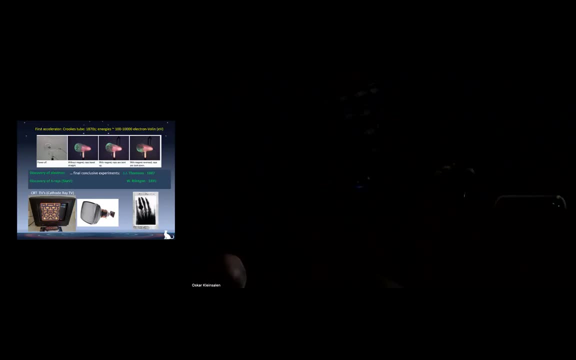 uh, just few molecules left there, ionized by this electron, so you can see them. if there are no molecules at all, then you will see nothing. uh, so now i think about this beam that it's really really straight, it's it's not some chaotic movement, it's really very straight and i mean you can make it. 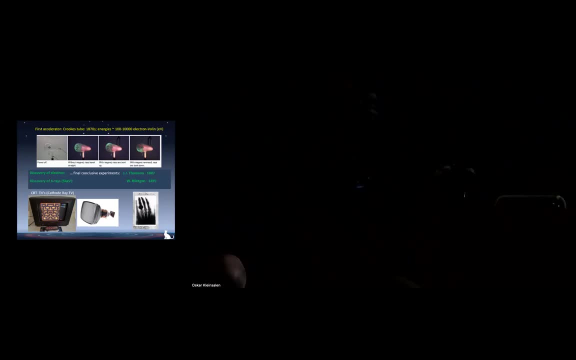 very long and shine against some objects, see shadows and measure. one thing you can do: you can take a magnet- it's here magnet- and you can check that the sink has a charge. okay, do you see it? so i i change the trajectory of electron, uh, by applying magnetic field. 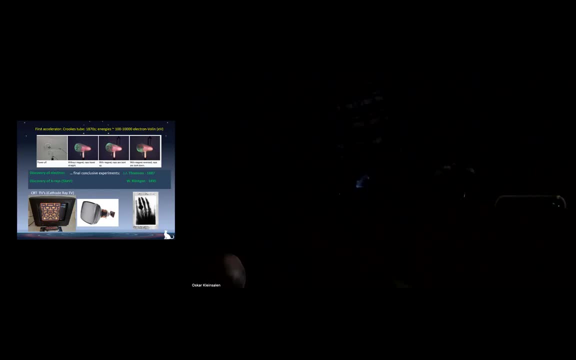 and of course in the laboratory you can know how much magnetic field you applied. you can do it a controllable way and you can measure a ratio of electric charge to the mass. so curvature of banding with electron is the magnetic field of the electron. so you can measure the electric charge. 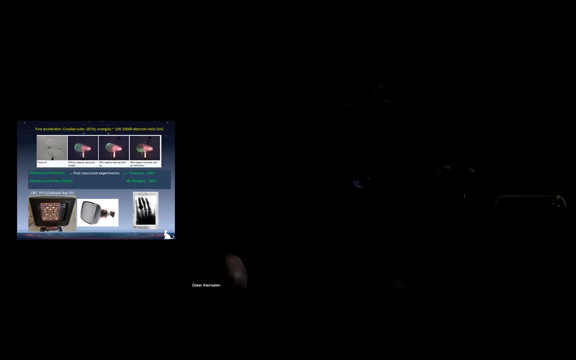 is like this: you see curvature of this. curvature here proportional to ratio of electron electric charge to the mass. so if it's negative it goes here, in the positive you go opposite way. and it was using magnetism. it was clear that it was negative charge. eventually people realized. 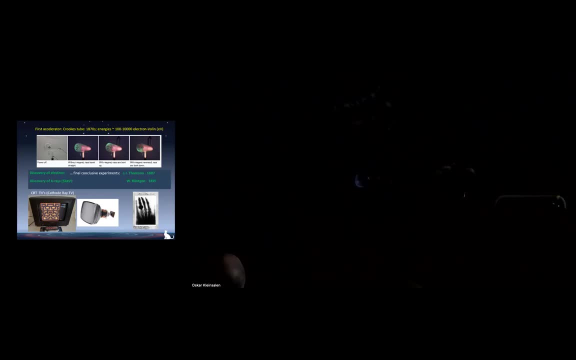 that it was electrons which carry electricity, which was already known because they were running locomotives in the london underground already. the new electricity is new how to operate, but still still didn't know what is the carrier of electricity. but with this experiment they could do it first time. they actually did it by surprise, they did it basically. 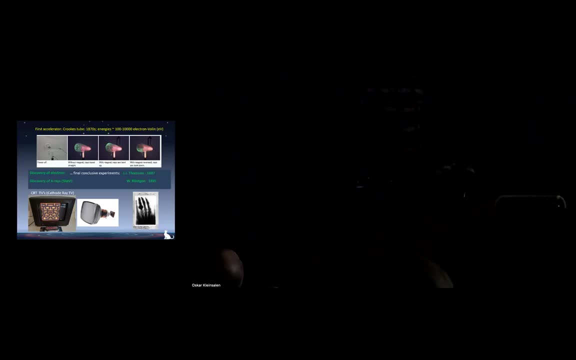 they could not believe themselves. they got that ratio of electric charge by the mass is thousand times bigger than they expected and they discarded it for about 10 years until thompson, did a scrutiny experiment, say no, actually this is correct. this is thousand times bigger than you think and it's. 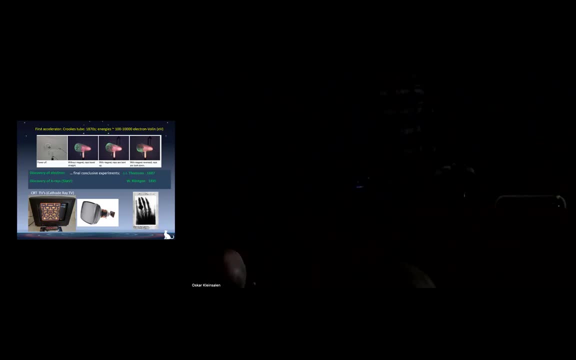 because electron is just like that and white thousand times bigger, because all the mass of atoms is a nucleus, not an electron. electron is 2 000 times smaller in mass than proton and people, of course, do not know it in the past. okay, this is experiment, this is what is. uh, was done. okay. 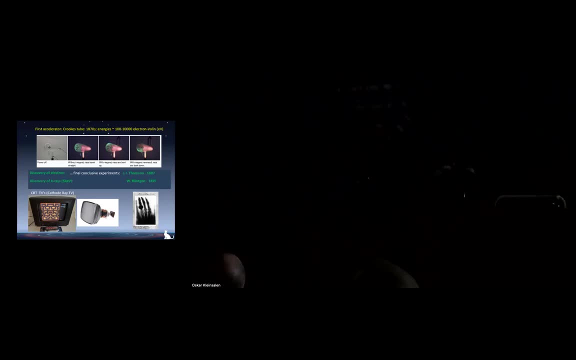 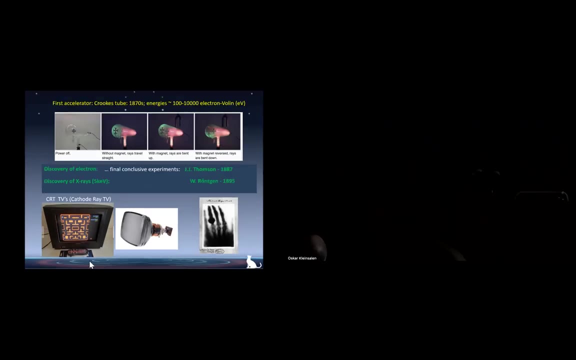 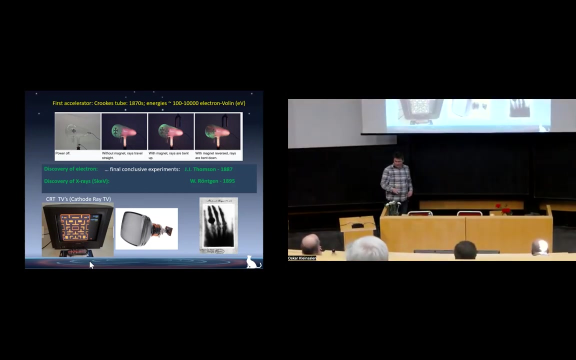 on the break you can come and try yourself. it's quite fun how it works. okay and right. so this is just another incarnation of the same device. you see that i mean here magnetic field. this is magnet here applied. change your direction. so electron was discovered, moreover, if you increase. so i used 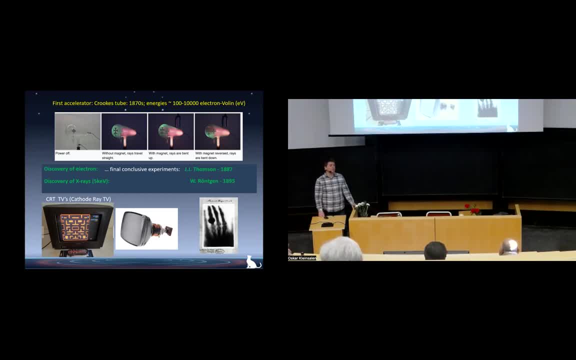 300 volts. by the way, here introduced energy scale, it should be electron volt. i'm not sure why it's become my family name. maybe i was tired to type the slides, or maybe it was autocorrected, i don't know. uh, anyway, so it should be electric scale. 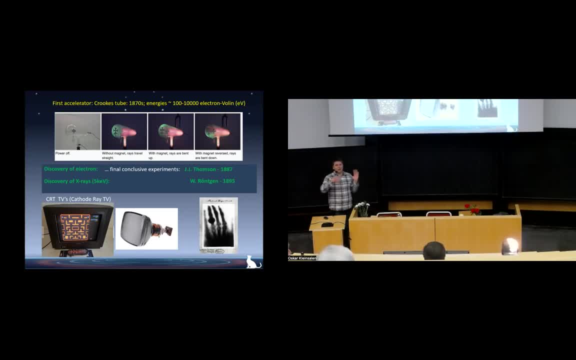 electron volt, and electron volt is energy achieved by electron by passing potential of one volt. So when you're passing through this tube in the device I showed you, energy of electron was 300 electron volts. If you do it, 5000 electron volts- electrons actually. 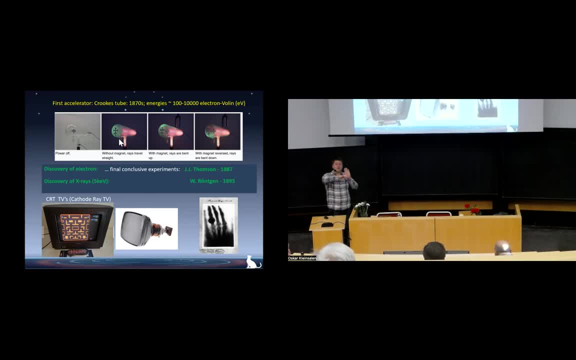 when it's close to the nucleus, it can emit X-ray radiation. It's called- in this case this is called Bram Strallum effect, And this X-ray radiation was found by Röntgen, for which he got Nobel Prize, And this is a picture of his wife's hand. It was not intentional. 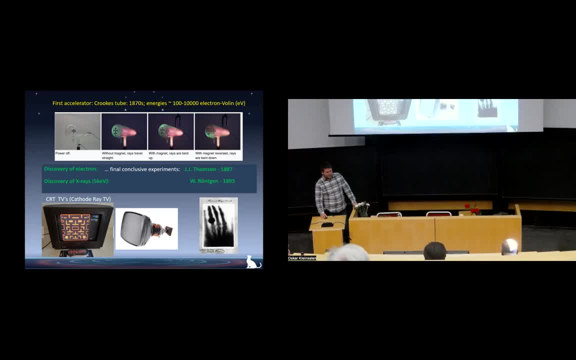 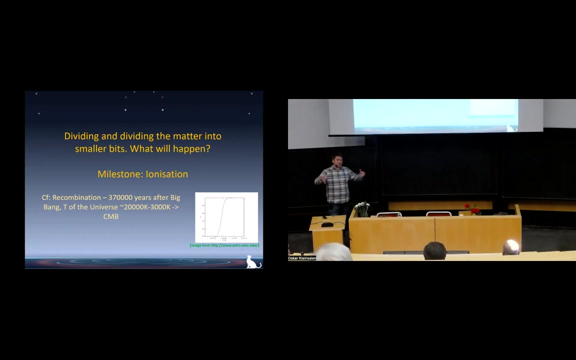 nobody knew that it's harmful, I hope, And anyway. so this is all this stuff And eventually they were used to do television and I still remember I had it at my home before it become a modern television. Okay, I'll tell you this: that people discovered electron. 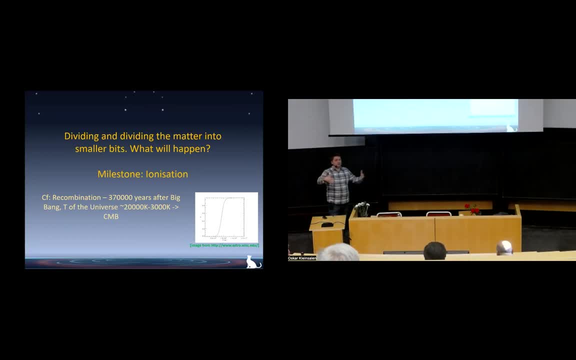 at this time there is protons. I mean because matter is natal. If there are electrons, there should be something which has compensate charge, should be positive And, moreover, we know that the mass of electron is almost nothing compared to the mass of the atom. 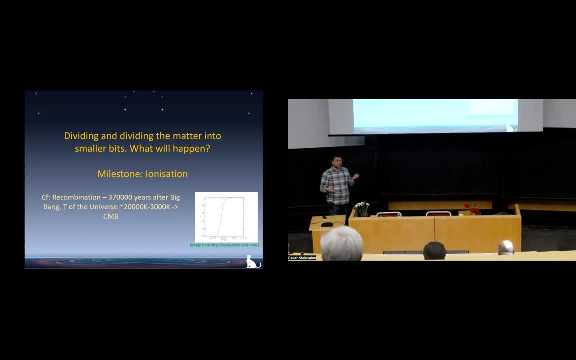 So everything else is a mass of, or should be of, what is positive, But it was called proton eventually, And now we actually want to ionize and ask what's happening next. So this ionization is a milestone in our decomposition of matter into small things. 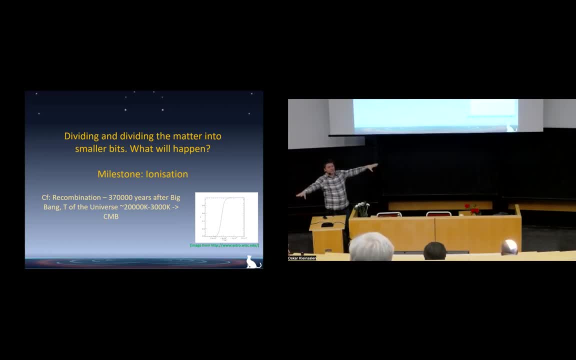 Actually we're doing a little bit the opposite. what happens with the evolution of the universe? This is a plot. It's not clear numbers, probably, you can't see them, but I will tell you. So here is a temperature. So here it's 5,000 Kelvin. 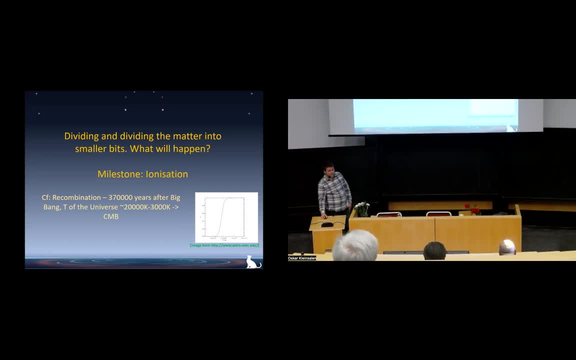 which is surface temperature of our sun, And this is 15,000 Kelvin. It's temperature of quite hot star. The hot stars have temperatures of 50,000 Kelvin, So it's quite here already. And this axis is a fraction of hydrogen atoms. 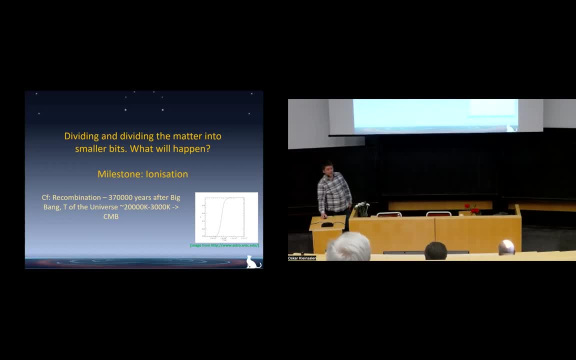 that are ionized to proton and electron. So at 15,000 Kelvin almost all hydrogen atoms become ionized. So it's becoming really full plasma. proton separate, electron separately. That's what happens in very hot stars on the surface. 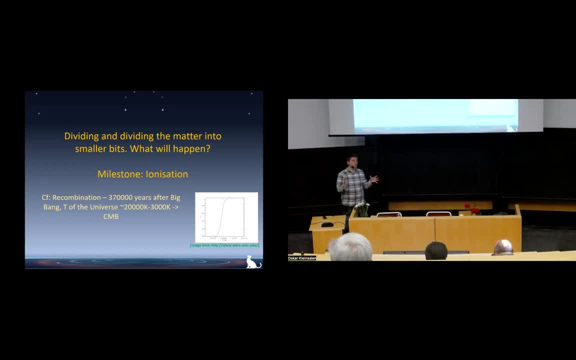 In our sun. actually, on the surface, we have hydrogen atoms. We do not have hydrogen ions, We have hydrogen atoms. Hydrogen atoms exist inside the star, but temperature is much higher. Anyway, after big bang, temperature is very hard. everything was ionized. 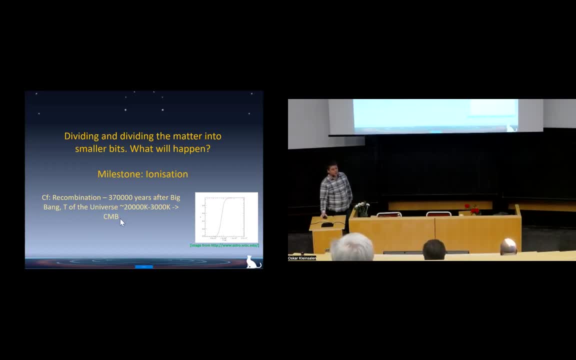 until it become a combination epoch. this number of years after the big bang, And basically between 15,000 Kelvin and 3000 Kelvin, is when electrons and protons start to form hydrogen atoms. After it's cooled down to 3000 Kelvin. 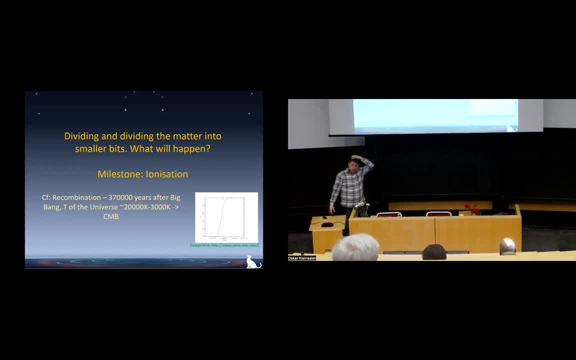 slightly less than temperature of surface of the sun, matter become electrically neutral and all the photons escaped interaction and flew to the sky, to the space, And they flew for 13 billion years until they reach us today And we observe from the sky. this is called cosmic microwave background, The oldest light in the universe that we can observe from the sky. It was 3000 Kelvin when it was emitted by Q2 redshift. These days it's only 3 Kelvin, maybe a little bit less even. 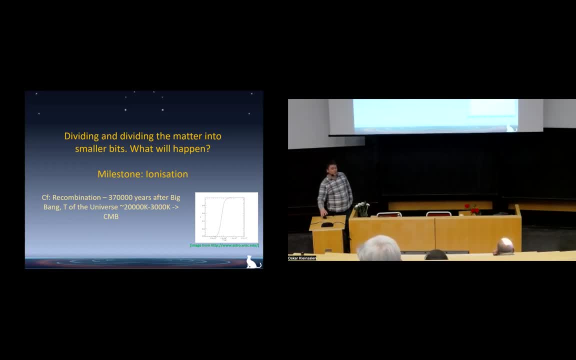 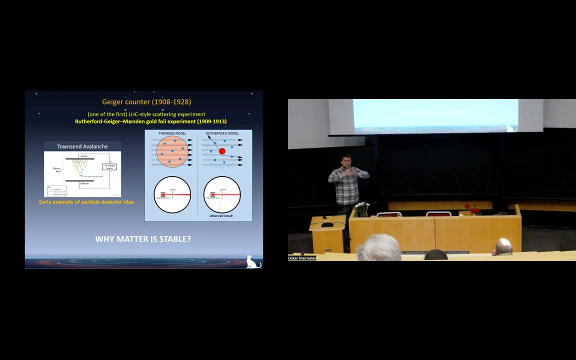 Anyway, we're going opposite. We're kind of exciting atoms, we want to ionize them And because now we know that there are electrons and protons, it's a really important question how they combine to. this First idea was by Thomson, that this big pink stuff. 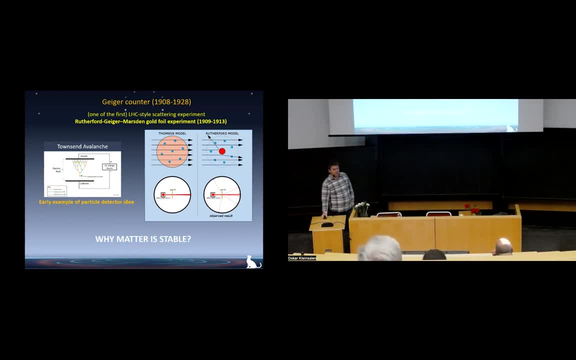 is a proton, it's a big pancake and blue guys are electrons. But actually it was disproven by Rutherford-Geiger-Marsen-Fold experiment And this is the first LHC-style scattering experiment, I would say, And the first emission was first accelerator. 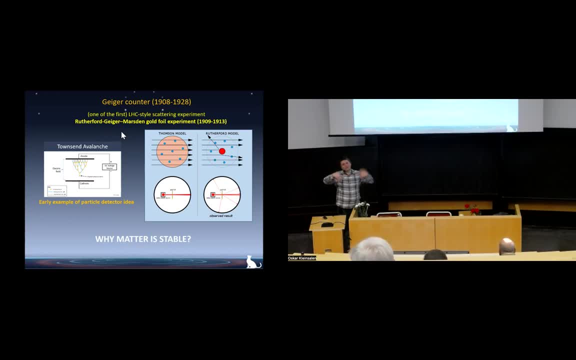 that this is the first. like good scatter, We accelerated electrons, but we did not much with them. we just curbed them. But now we actually emit alpha particles. Alpha particles is helium nuclei which sources radioactive elements. they were known by the time. 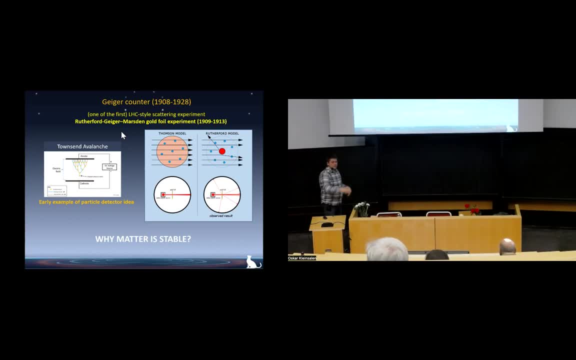 Alpha particles source and we put it, push it towards foil and see what happens. This is typical scattering problem, the same type we do in the logistics, And this was done in 1909, in 1913. It was possible to do it because there was Geiger there. 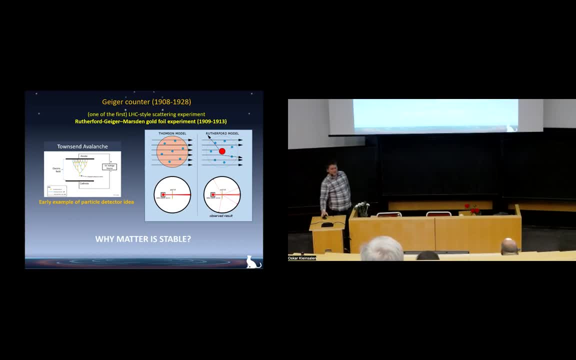 who developed Geiger counter. The Geiger counter that you use these days it's 1928, it's like cheap economic questions that you can sell. But early version of Geiger counters appear in 1908, like in Geiger experiments. 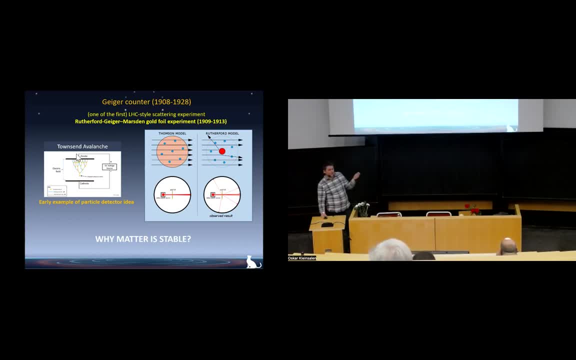 Of course, and he used the method. what is called, I mean, Geiger counter is based on Townsend avalanche. The idea is that you have, if you have a nice particle, if you have a difference of potential, ionized particles can accelerate. 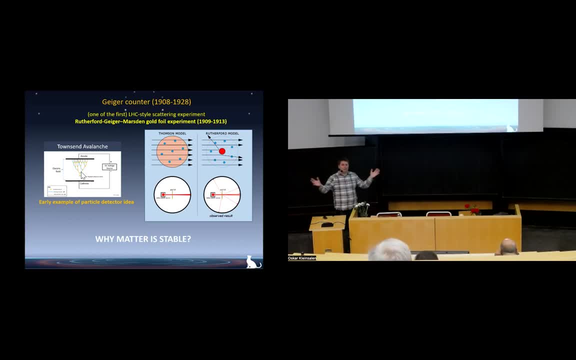 hit other particle, this particle will decompose, not decompose, ionize again, hit another and become an avalanche of ionized. So this particle accelerates, hits somebody else, hits somebody else, ionize. Two ions go away. hit somebody else, ionize again. 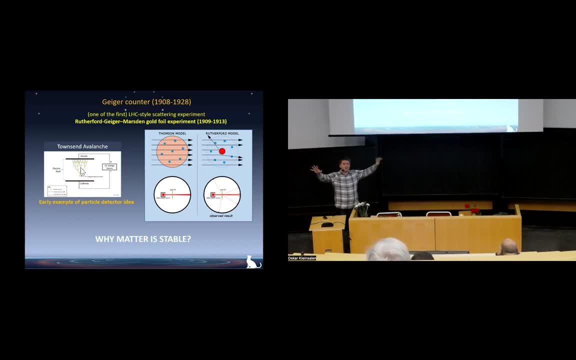 And this is avalanche process- become bigger and bigger and bigger. So the trick here is to make a fine balance between density of gas. If it's too dense, everything just die off. If it's too sparse, this particle will hit nowhere and reach anode, reach anode. 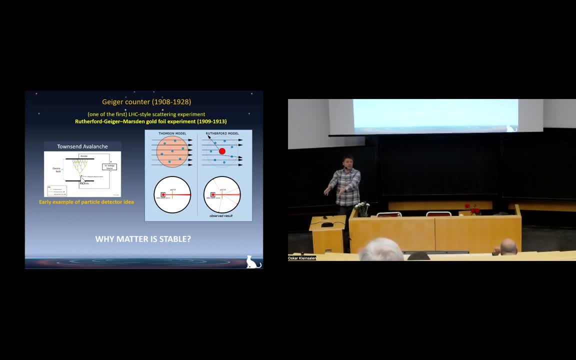 So it's the same setup as this cathode you have here, but it's very well aligned density of particle. It's very well aligned density of plastics inside, as it allows for avalanche. And why we need avalanche? because we want just one single particle, alpha particle. 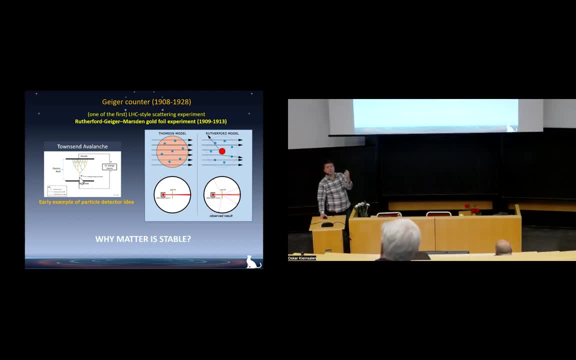 create a lot of one so we can actually measure experiments. This is how detection of various small events happen these days. For instance, this is how we detect single photons- is we are detecting single photons by something called photo multiplayer. It's exactly this thing happening. 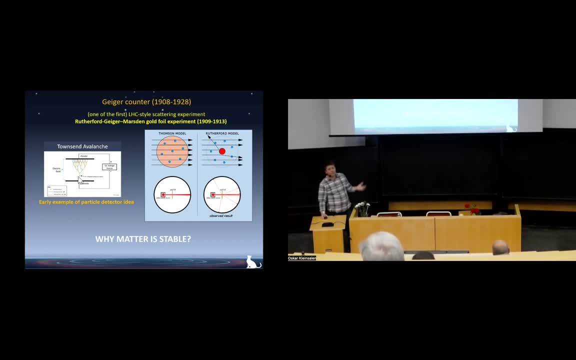 One photon comes and creates an avalanche of new photons that we register. This is superb. It's exactly this thing happening: One photon comes and creates an avalanche of new photons that we register for pre-course of motor measurement devices. and this how geiger counter works, uh, by modern. 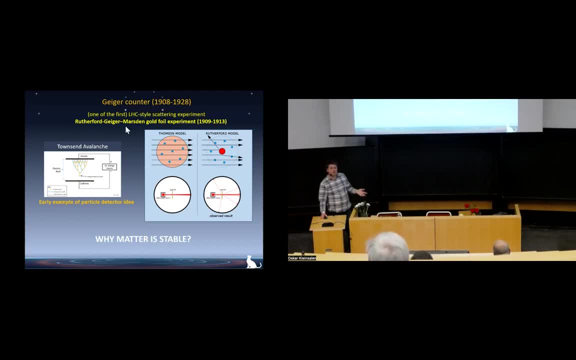 standard. geiger was also for further fork and martin was phd student of geiger. this is the same name but there was no post-op in modern sense. but this is basically how they were related and they did this experiment and what they realized: that alpha particles passed. 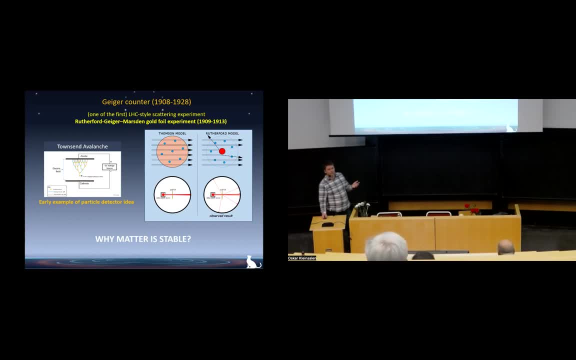 through gold foil almost is no deflection, it's only very few events. that was reflection and uh it's. they concluded that nucleus was actually very, very small compared to, to, uh, to the size of atom. i mean, you can estimate the size of atom just uh, take volume, if you see. 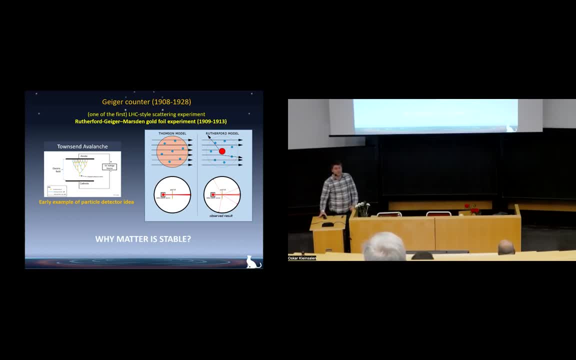 some divided number by number of atoms, you have that it will be size of the atom. so nucleus happened to be very small and this was a conclusion. and this conclusion was troubles. so why? because i mean, people were not naive. there was a reason to do thompson model. 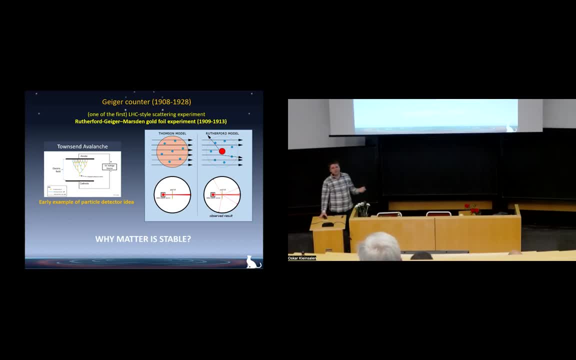 because in this model, electron is actually attached to positive charge. when you have positive an electric charge, they want to be together. it's called coulomb attraction, right? so why this electron doesn't fall on the proton? why, why not? i mean it should. well, if it goes around it. 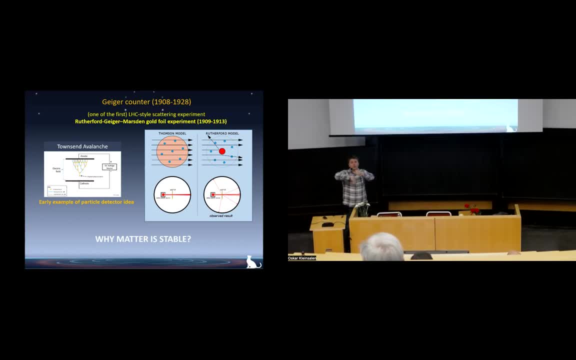 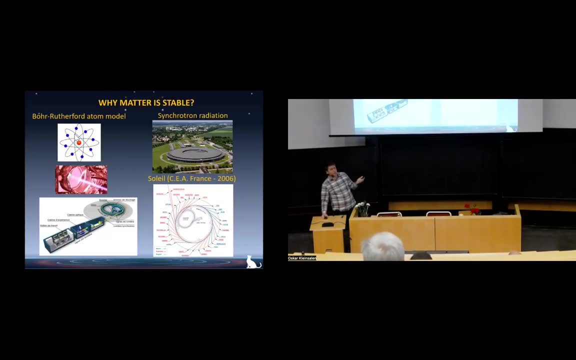 will be like a earth going around the sun. the earth going around sun. it's like a capillary problem, but for it- and that's what people did- this is called uh. this is they uh, for like a model, but it doesn't work. it should not work. some people actually wrote statement: yeah. 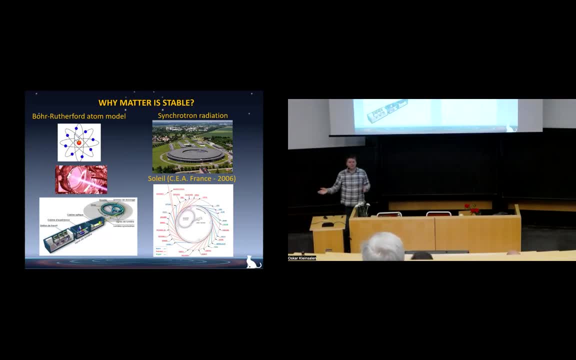 it should be like this. somehow it doesn't work but it takes forever. it doesn't take forever. this model, if it's classical, doesn't work, and modern example of this doesn't work- is called synchro. synchro from radiation, it's classical, result from classical electric dynamics and we have 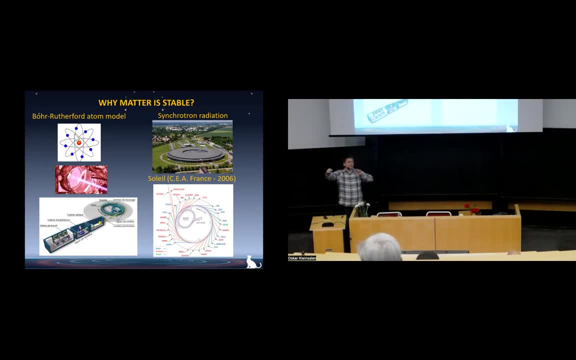 charged particle which accelerates change in direction, it emits radiation. if particle goes straight, it will not emit radiation, it will be okay. but if particles bends, actually tangent to its direction will be radiation going out. emitting radiation means losing energy. losing energy eventually means losing velocity, falling through the nucleus, through the synchrotron radiation. electron should lose all its energy actually quite fast- you can estimate how fast- and fall to the proton. so matter cannot be classically stable these days. synchrotron negation can be problem and it can be benefit. it can be problem if you want to accelerate particle to very high speeds because the faster particle goes. 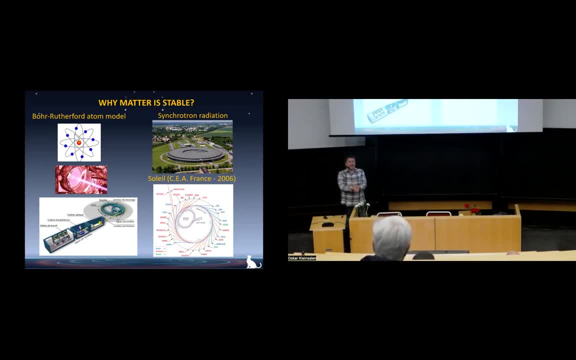 the more radiation it will emit. if you do it on circles, and the lighter particle is, the more radiation will be there. so for this reason- uh, it's one of- i don't know if it's all the reasons, but definitely it's cost much more energy uh to uh to accelerate electron at the energy scales of lhc. 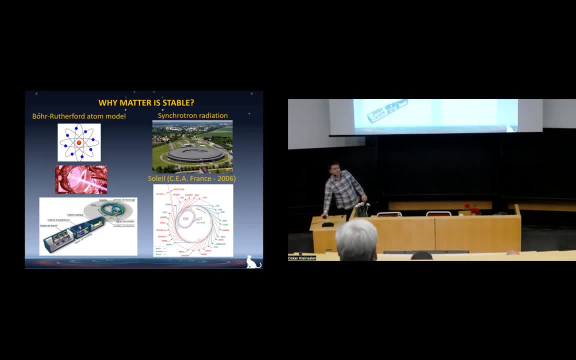 uh, so you can accelerate electrons to, to geek electron voice. so, uh, here it's 300 electron volts. x-ray happens at kiloelectron voids. uh, like 10 times more. uh, mega electron voids is energy of nucleus. this is one thousand more. it's a giga electron. uh, lhc, it's terra. 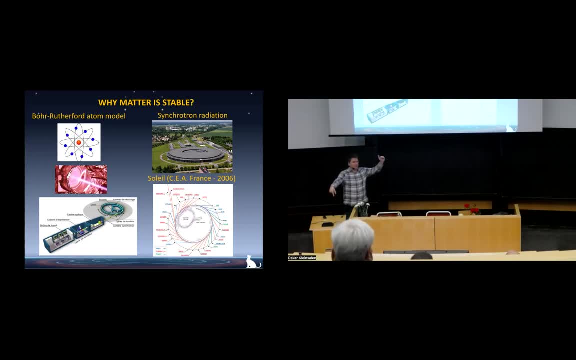 electron volts, it's a one thousand more uh. so you actually it will be very pricey to excite the electrode more than giga electron volt because of synchrotron radiation. so they do not accelerate electrons, they accelerate uh electron voids. so they do not accelerate electrons, they accelerate. 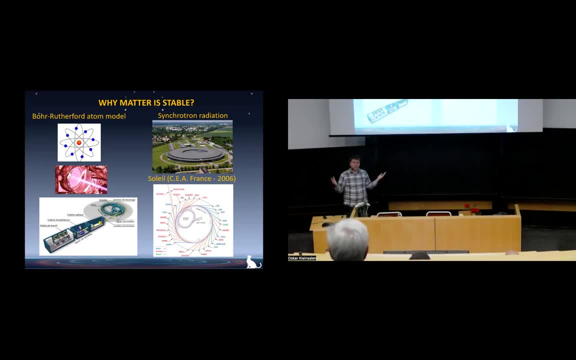 hadrons protons on lhc because they emit less proton radiation so it's cheaper at that high notch. on the other hand, synchrotron radiation has nice features that can be useful, because this beam has you can have very, very good control on the beam. it's very well focused and you can control. 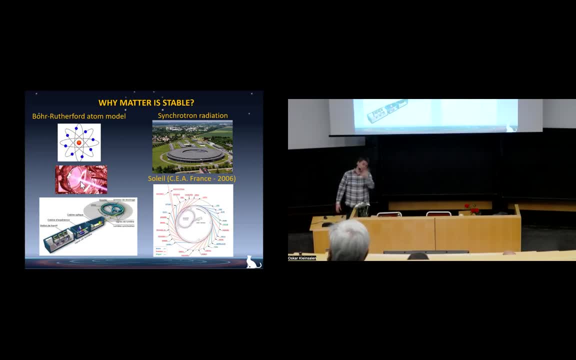 its high precision characteristics and it's used in very many different applications. i don't, i know only one, because i'm a theoretician, i don't know much. uh, one is: they try to cure constant. they shine with this radiation on tumor cells, killing them, because it's very press. it can be done in a very precise. 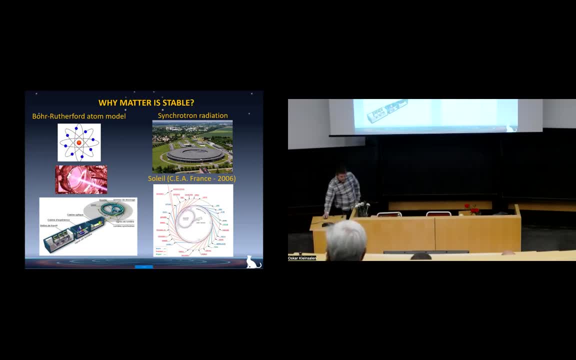 way and but here there is about 20 to 30 different labs, so this is big accelerator around uh, so it's a small one. accelerated electrons, 2.7 g electron volts. then it injected in a big accelerator here. they do not want to say it more, they wanted to keep going and would constantly radiate. it will. 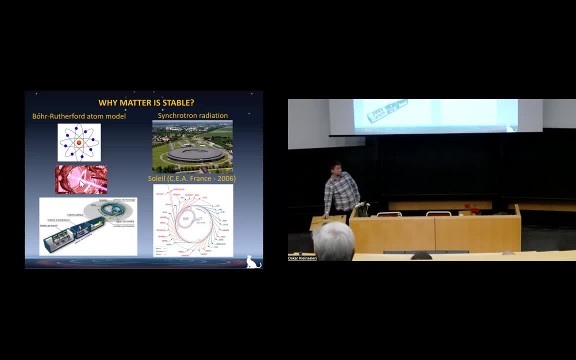 radiate this, this radiation this is. it's very similar to what we saw, right with the electron, but this is em light. it's just electromagnetic waves, just very highly energetic noise and things around. and well, this, this is electron moving around, shines beam light here, here you. 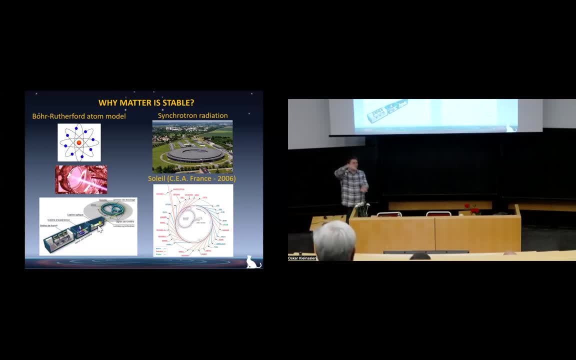 do some optical devices to turn it around, split like whatever you do this in optics, and here you have all the computers, devices to measure and finally, here, people sitting and typing my emails, right, uh, so this is how it looks. this is one of the examples of synchrotron it was built in. 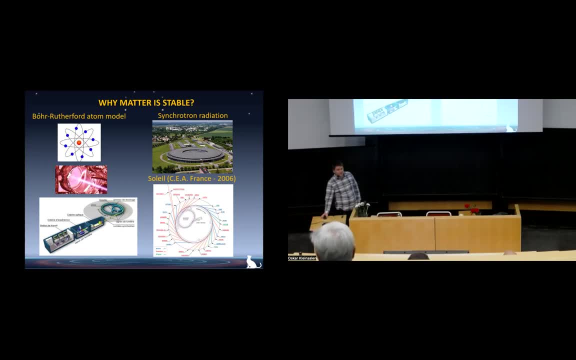 2006.. uh, it's a. it's situated in central energy, atomic france. um, so why? why i chose this one to show? uh, well, because here. well, let's start from here. this red building is actually institute of territory of physics. this way i did my phd, so i never was here. i was never here, but i saw it every day. 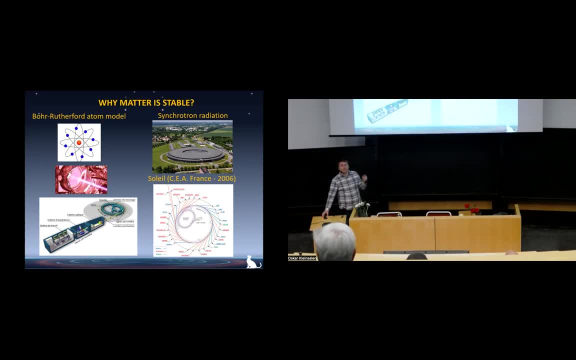 not it working, but it was. i finished my phd. no, i started my page in 2006 and it was kind of- i mean, it was already working, but all this was still construction work. is parking slots lots not working yet there was a lot of, so i saw so progress of it's starting to work. 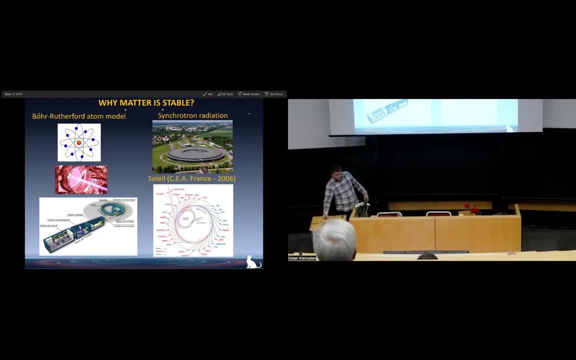 while i'm doing phd, uh, in this building, red building, here and here, this white part is actually actual center of atomic energy, which was a french atomic project. well, still is, but it's much was more important in, like in 50s, 60s, when people were building. 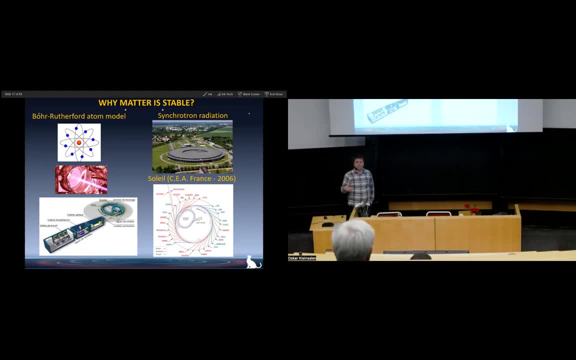 nuclear plants have to develop nuclear, different nuclear things. so it's a big thing, this security. you cannot enter that easily like they will check. you have a budget, small, small, it's a big thing there. we went there to have lunch, okay. so it's good memories for myself. 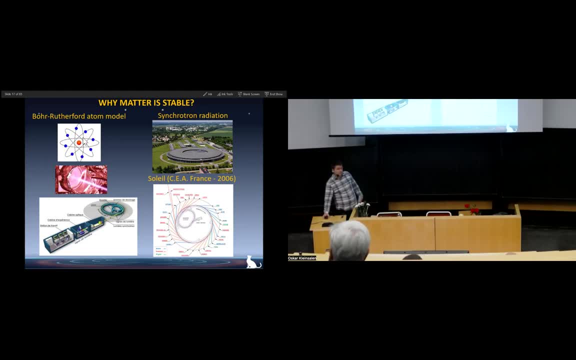 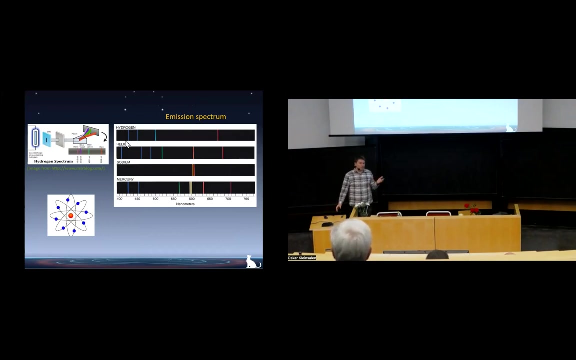 right. so this example, central radiation, what I showed it to you because I wanted to tell you that classical atom in reserve for port type is impossible. this is one problem. another problem is is that emission spectrum of hydrogen is not continuous. this is a standard experiment. here you have hydrogen. 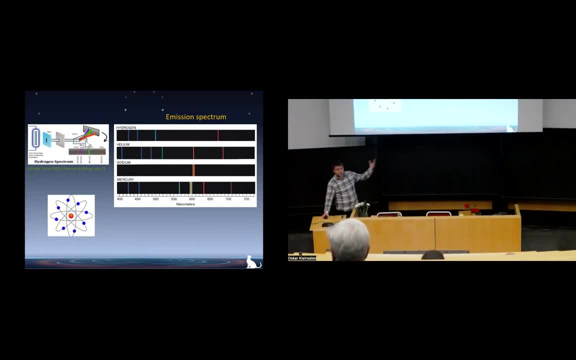 it shines through some slits and here you have prism, like Newton did 400 years ago or even more, and splits in different colors. and hydrogen actually shines only very narrow, but it's discrete. it's example of quantum phenomenon and this is true for most of atoms and molecules. they will have. 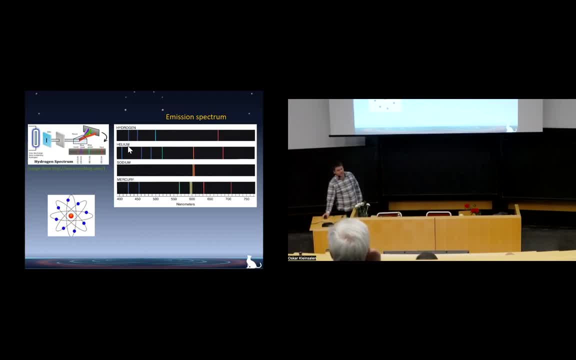 the more complicated things, some bonds you'll have, but it's still discrete and it's also going to be explained classically. so first thing was done. Bohr did it. he said: okay, I will postulate that EM radiation doesn't happen. I do not know why. 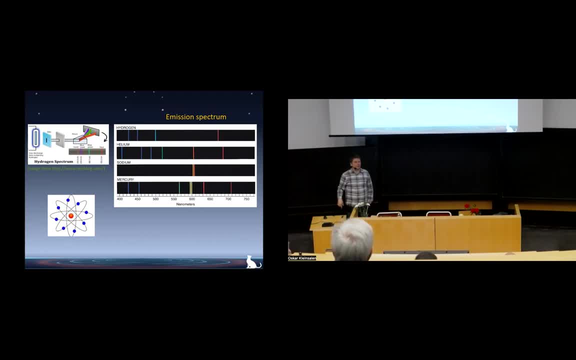 and second, I will postulate that orbits allowed for violet to not be quantized. postulate this compute and he got correct answer and people were very happy. that's because answers were correct. I mean, these lines were reproduced from theory. we use these postulates and this type of Bohr answer is very good. 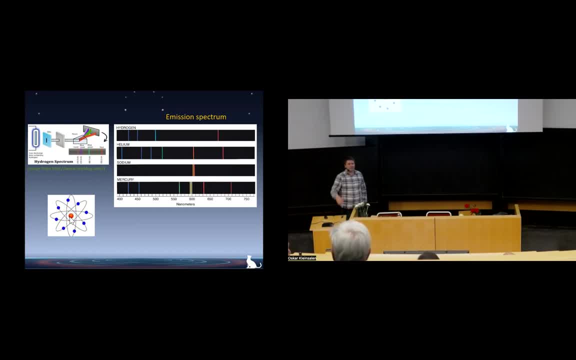 and this type of Bohr answer is very good, and the Atom picture is still quite popular. at least they were popular when I was student myself. I saw them on different buildings, like on different books. actually I have students now. they wearing experimental sports and on the back of them. 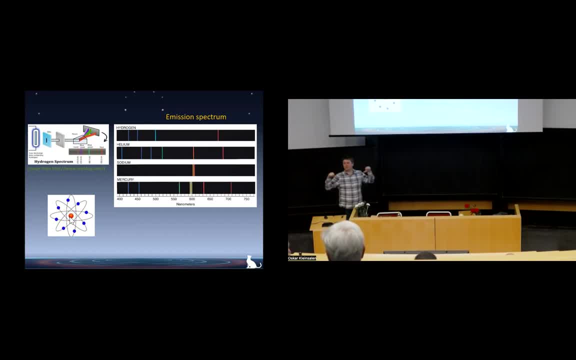 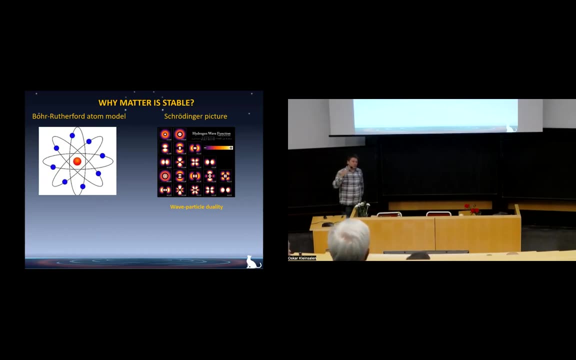 they have big Bohr atom drawn now, in 2022. anyway, it's good that this postulate works, but nobody understands why, and here we actually need to go to quantum mechanics. so we have to apply wave particle duality and change classical movement by the two wave probabilistic description. we say that 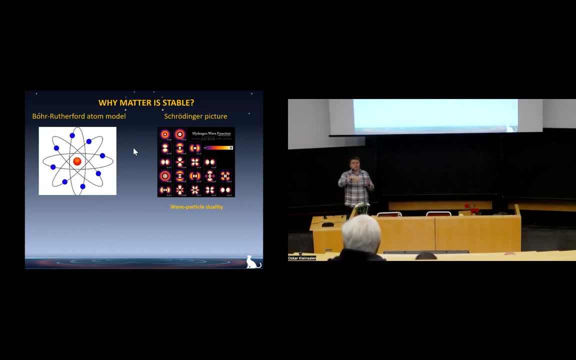 electron is not, is not here or there. it's actually a probability wave and it's probabilistic distributed like like a jelly around it. there are different configurations of orbitals around tatum. this is like probably it should be ground state. no, it's actually first excited state. this is: 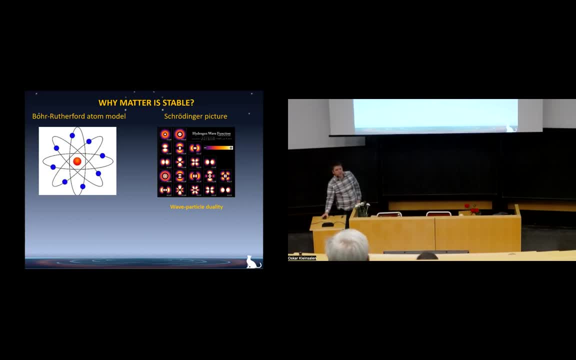 another excited state. they actually didn't show ground state because it's too boring to draw. this is what's called p orbitals, and so this is how probabilistic distribution of works. a lot right. this is what follows from hydrogen, from schrodinger equation, and explains how atom 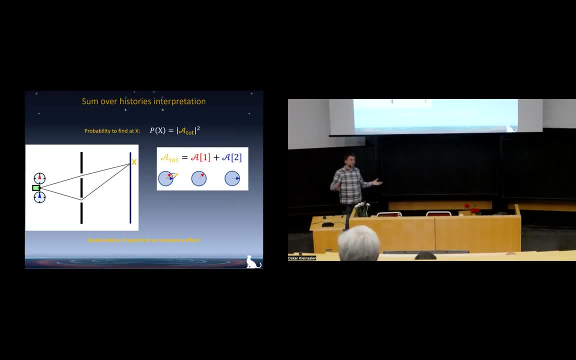 is working. but also i need to remind you- or those who are new here tell it for the first time- some of the history interpretation, because what we're going to do, we are going to do scattering for scattering. it's very useful, so in quantum, so what it is in quantum mechanics. 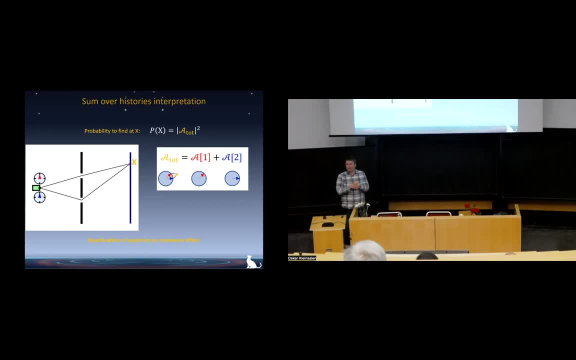 it's de facto denial of objective reality, so denial that you can say something about the world without observing it. and so what i'm going to do is i'm going to close my eyes. i cannot say you're here, because to to be sure that you are here, i have to open my eyes and see. 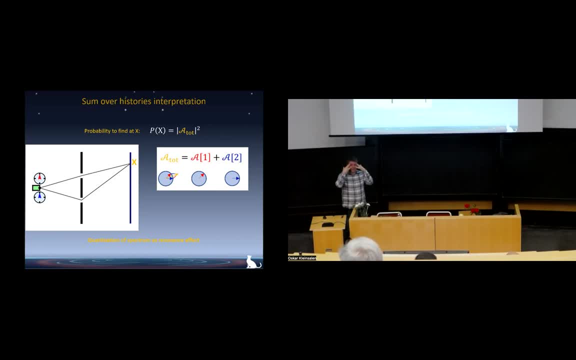 okay and in quantum mechanics a big problem. i tried to explain it several weeks ago because sin- sin is actually perturbing the system in quantum mechanics. so i denies knowledge about so. basically i'm agnostic, i deny that you exist or don't exist, i don't know because i do not see. 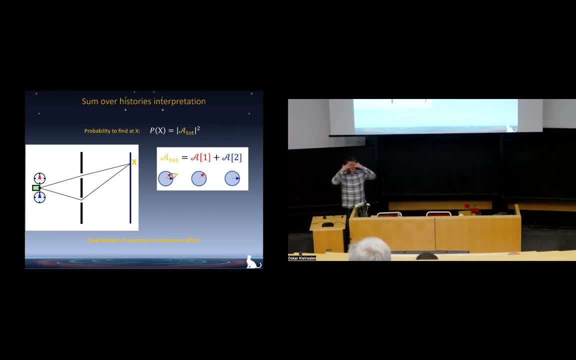 whatują, and now we're going to accept the fact that you are not here? you don't know you are here and now. i don't know you're here and now. so every time i close my eyes, i do not know if you are here. in quantum mechanics, uh, you even cannot ask whether you're here. 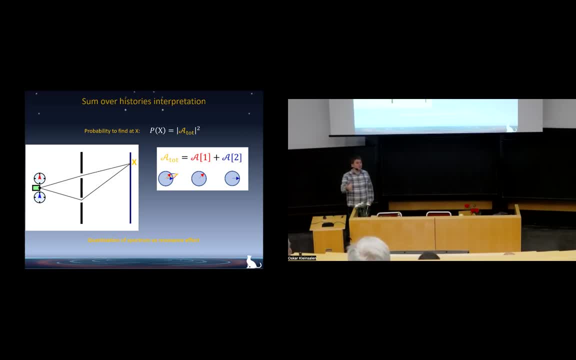 you can ask the question i, what is probability that you will be here if i open my eyes, like 50 percent here is a here or not, right? uh, this is from the double slit story and you can ask question: what's probabilities electron will be here and there is a prescription to compute it and this is very interesting prescription. 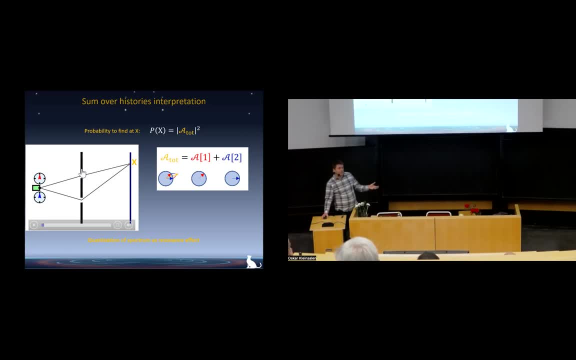 because, uh, it's mathematical tool. again, nobody knows that electron is actually there because nobody can measure it. it's forbidden to measure, but it's mathematical tool. to compute probability to for electron to be there is to do the following: assume that electron went from the emitter to the. 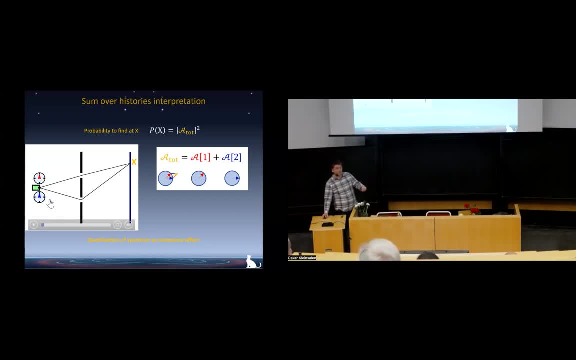 final point: in all possible ways, uh to each way. in this case there will be two ways to each way you associate the complex number. complex number uh can be represented if it's half absolute value. can be represented by a clock and this complex number will change uh while uh electron propagates. 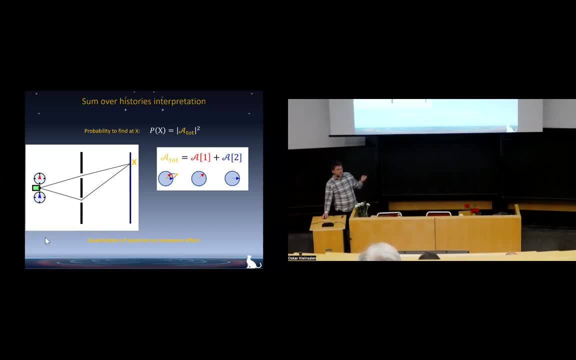 uh. so the point is that if originally complex numbers looked at the same direction, uh, because passes are different, they will uh become not aligned after movement finished. you see that, this line and then a complex number, represented by the mechanics, what is called amplitude. so this is just a number, amplitude associated to red pass, like this straight line. 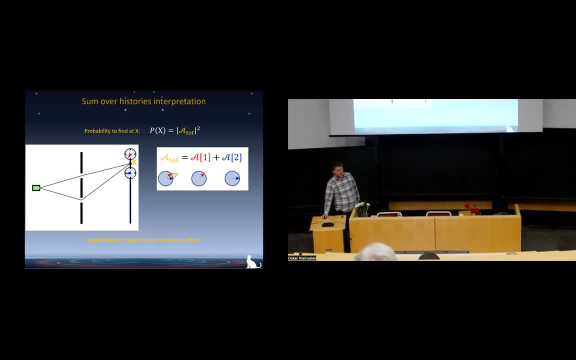 and blue pass, and what you do next? you have to sum them up using addition of complex numbers. so this is called amplitude, complex amplitude, and it's absolute value, square, gives you probability. so this mathematical recycle, uh, if you want, you don't care about all this mathematical stuff. 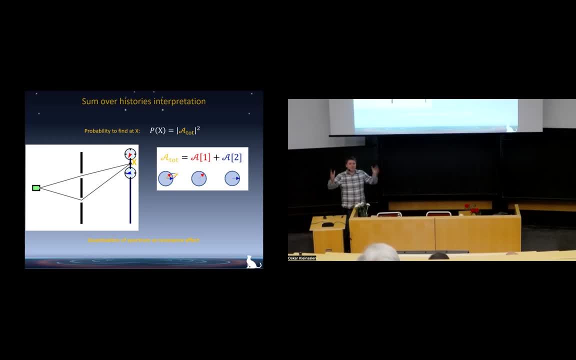 what you care about is that there are possibility for different things happen at the same time, at least, at least in our imagination. what happens in reality, we don't know, we just don't ask the question, but but it looks like electron does everything at the same time and in this interpretation, 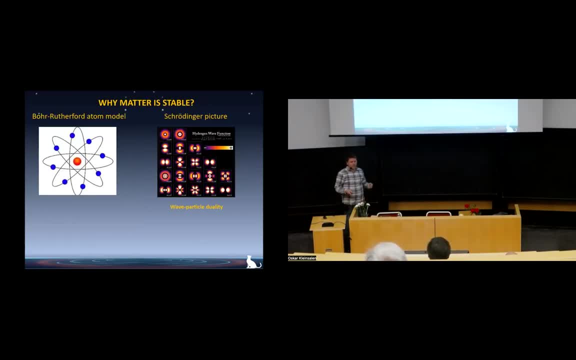 uh, uh. when we come back to uh this uh thing here, how to understand that bore model actually worked, because what you can think, that electron simultaneously goes this way and the opposite way. uh, both way predict the same energy, but they will actually cancel current and canceled current will be no radiation. so in this 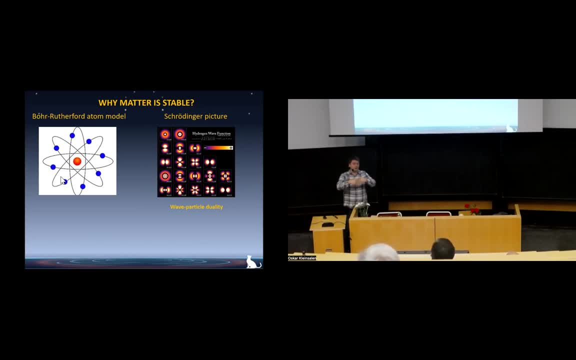 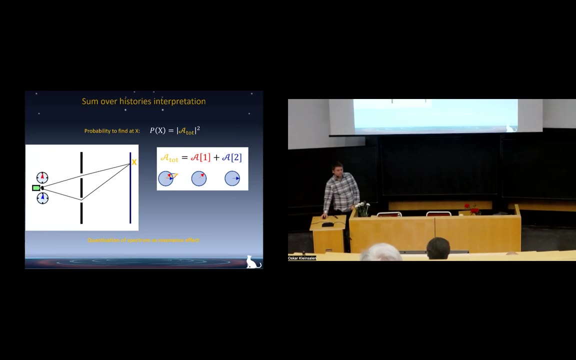 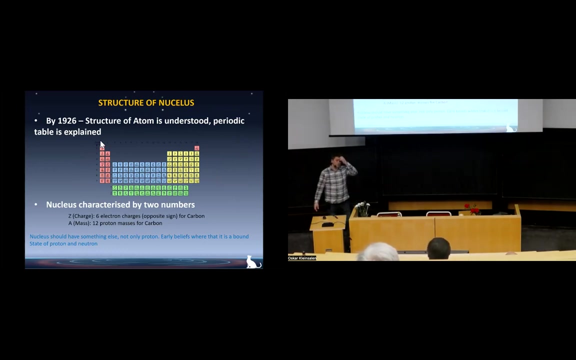 uh, past history interpretation. you can kind of explain why borer atom worked in principle, because you think about it going one way and another one sometimes. okay, um, so by 1926, uh, structure of atom was understood. uh was explanation, but periodic table. so we successfully decompose atom to electrons- fly away and to nucleus- nucleus- here it's now. 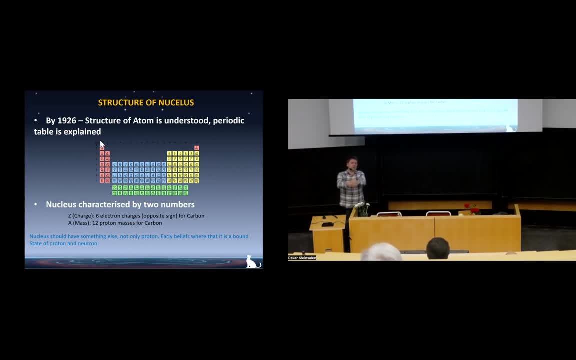 our next problem. remember, our goal is to reach lhc. so i spent for how much? 45 minutes and 20 years, right, so we need still 100 years to go, right, uh. so now we came to to the nucleus, and the nucleus we have, uh, two numbers which are important: what's the charge? and another is its mass, and uh. 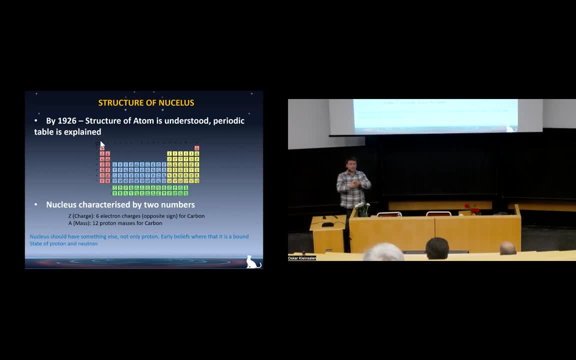 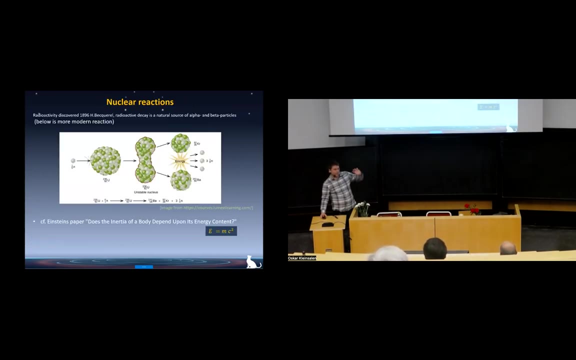 so now we know the charges. for example, carbon is six. it means there will be six positive things, and, but the mass is 12.. so it should be six of something else. who knows what it is? so eventually people understood this is something called nato. but before we go in here, i want to tell you something which will be very important for every. 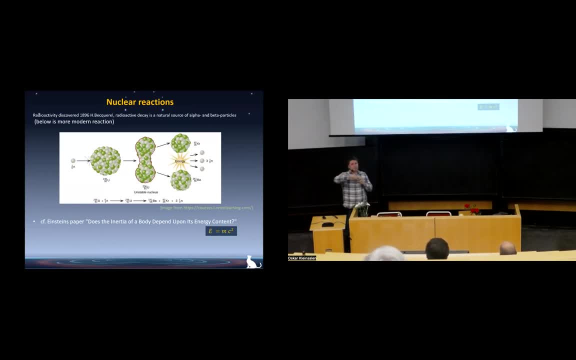 city which goes in. uh people were able to decompose uh nucleus without at the beginning, without shining, with all the complicated radiation in the nature. we have uh radioactive elements which were discovered 1896.. uh radioactive elements emit alpha particles, which is helium nuclei, beta particles, which electrons. they also emit gamma quants, just photons and 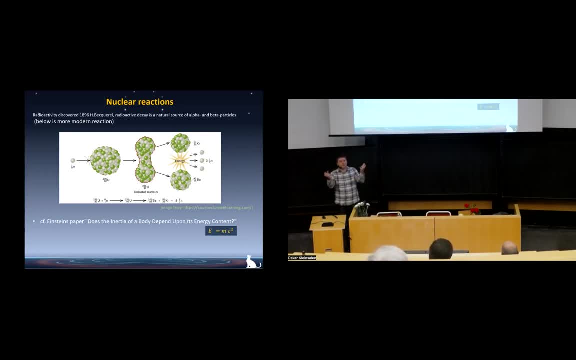 and you basically see that nucleus. well see, you can understand that nucleus decomposes and uh uh. what i wanted to emphasize is that, for instance, uranus decomposes into krypton and barium and also three natrons which fly away. so this is a chain reaction which behind uh atomic plants, or 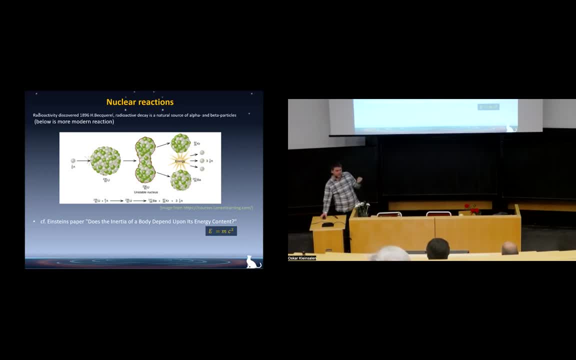 nuclear bombs, uh. but what i wanted to emphasize, that some of masses of uh volume, uh, krypton and and the three neutrons- is less than total mass of uranium. here and difference is energy which is emitted and which we use to to power our nuclear plants. and here it basically the first time when 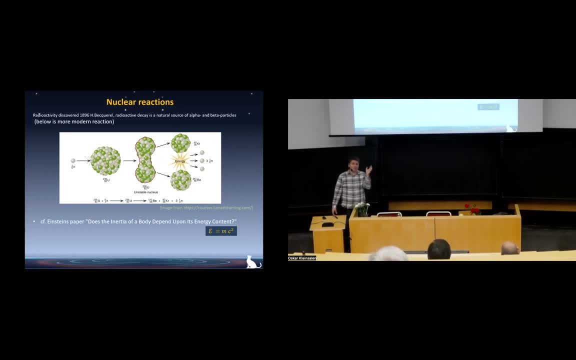 instant formula equal mc square becomes useful in practice. uh, so, because speed of life is very big number, uh, until now, change of mass, because of change of energy, cannot be perceived in the next experiment. so if you have think of one mass, think of another mass, put together just some of masses. 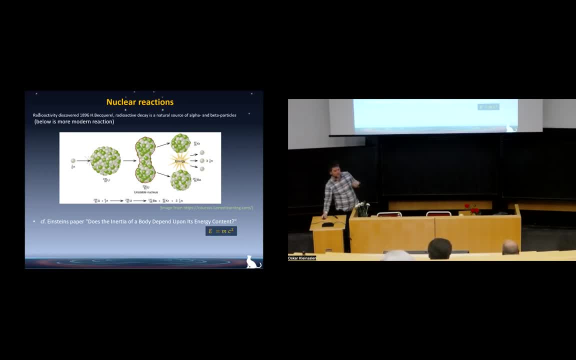 so this is example. when putting this together, we give you not this mass, give you bigger mass, and the difference is actually energy. by hd formula, we by. when you speak about nucleus, we reach the situation when transformation of mass into energy becomes important, and that's what is important. 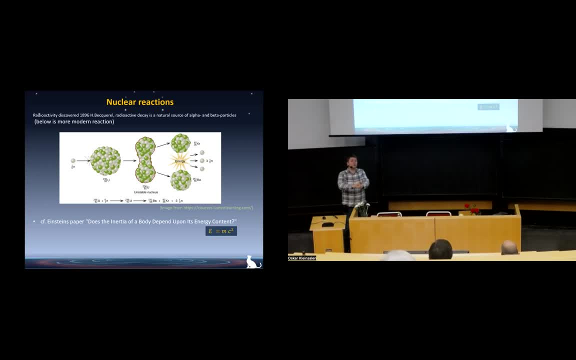 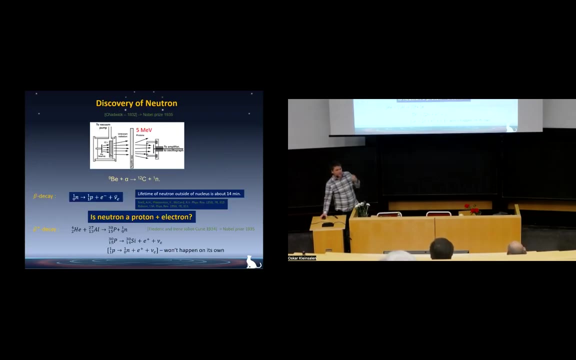 uh about nucleus. it's again something new. until now it was not important, it was just understood. but an experiment played normal in nucleus this place role. a few words about discovery of natron. so natron was discovered in uh in uh 1932 by chatwick. he got a normal price for it. uh, he actually used experiment of uh frederick. 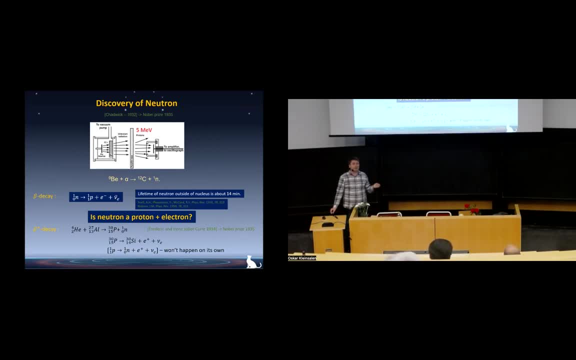 and iran julius curie. but he made the correct interpretation of experiment. iran julia query is the daughter of marie curie and, by the way, they also got a noble for price, but for a different reason. in chemistry they got the nobel prize for discovery of artificial uh- non-stable isotope of chemical. 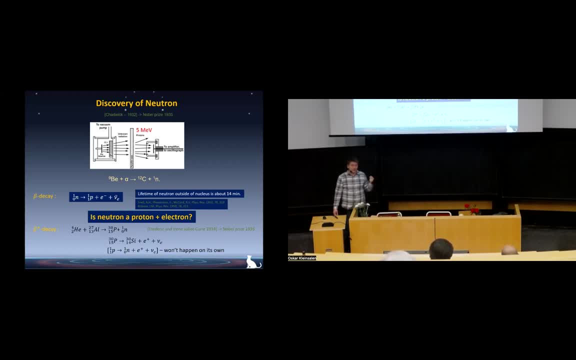 element, also in 1935, the same year, uh, anyway. so this was a top. so they took a source of alpha particles and now they shine on beryllium and eventually that is a neutron, and this is called beta decay. if we remove all the atoms, what happens is: 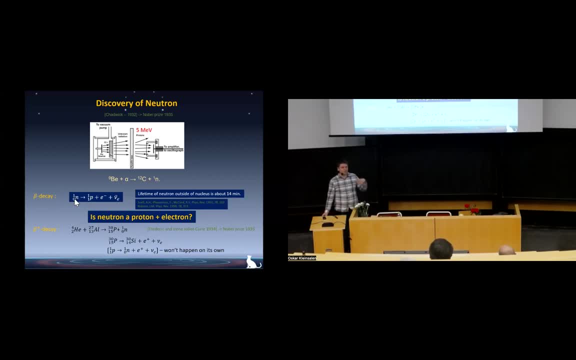 natron decomposes into proton, electron and also anti-neutrino. this experiment is no atoms nucleus attached to it was performed in 1950, but nevertheless, when you think about this, you say: oh, natron is combination of proton and electron, so it's a composite particle of proton electron. well, maybe the problem is that there's also beta. 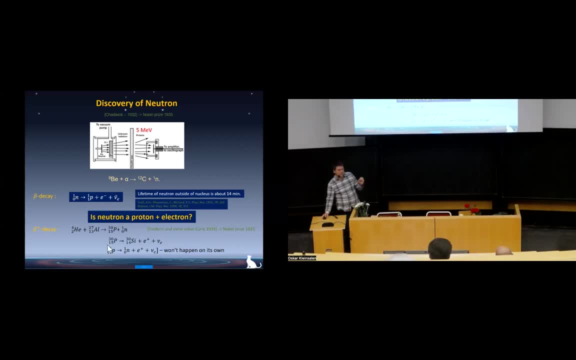 plus or positron decay. so proton, which is inside the nucleus, can decompose into neutron and positron and neutrino. it cannot do it by itself. if proton leaves, proton is stable. neutron leaves for about 14 minutes. if it's not inside nucleus, naturally 14 minutes like it flights in there, 14 minutes. 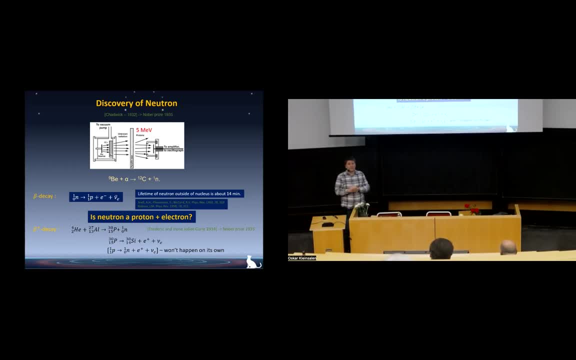 proton will stay for basically forever. actually, in when we speak about theory of everything, we will discuss why people want that proton decays. because, uh, ground unification theory predicts that proton will decay into something. uh, they look for it but they cannot find it. until now, proton is stable. 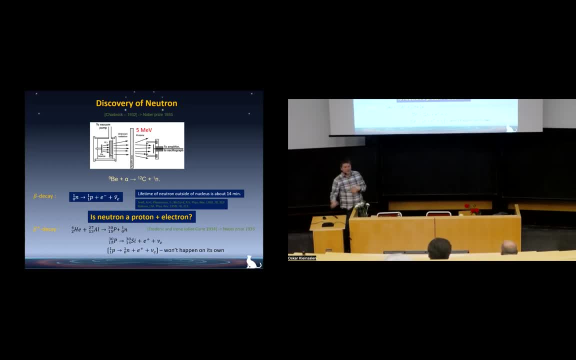 but even inside nucleus, with many other things around it, actually can decompose into natron and positron, which is antiparticle electron. and then we have a paradox: if neutrons, let's a natural is, is, uh, is composed of proton and electron name, so it's like a trash and adult story. uh, so in reality, uh, at this level, 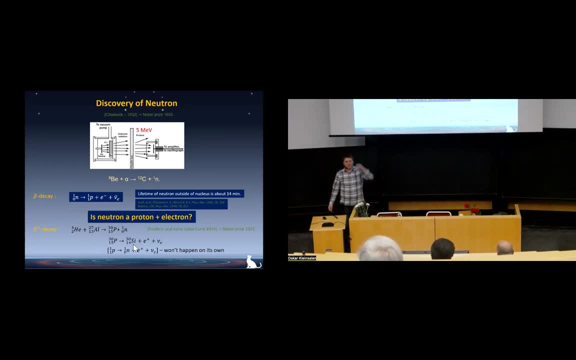 we stopped speaking about one particle. building consists of another particles. what happens now that particle start to transform from one from one to another? instead of splitting them, they transform. what happens? that when we want to split them, we supply so much energy that we can create new particles from energy. and this is what 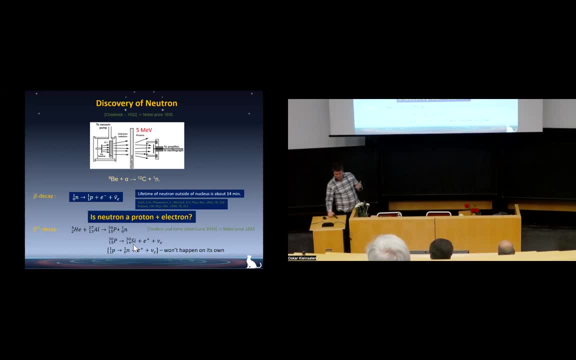 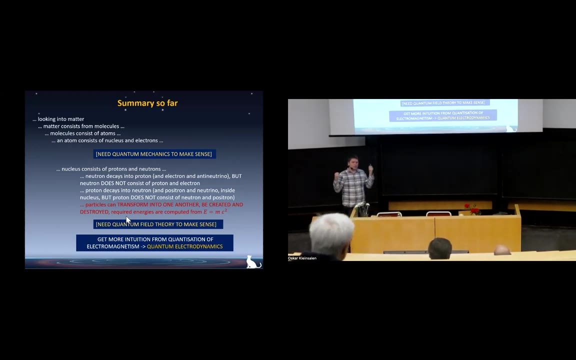 different happens and the nuclear scales. it's coming back to this here. we already see this energy present, but now we actually see that this place at all, because particles play the game. okay, summary: so we want to look into matter. we know the matter consists of two molecules. this is okay. 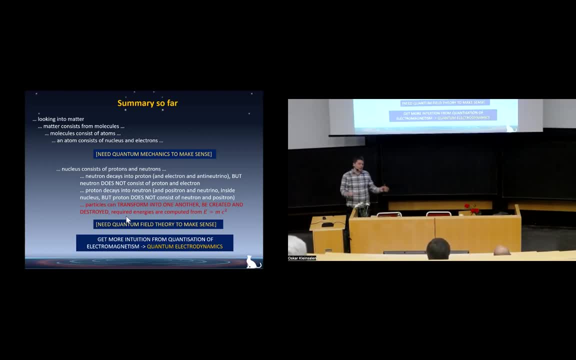 molecule consists of atoms. this is also okay. an atom consists of nucleus and electrons. nucleus is positive charge, electrons negative charge. and now, because nucleus is very small, electrons negative. for electron not to fall down, we need quantum mechanics to make sense. big change in our description. but then you say, okay, electrons far away, but 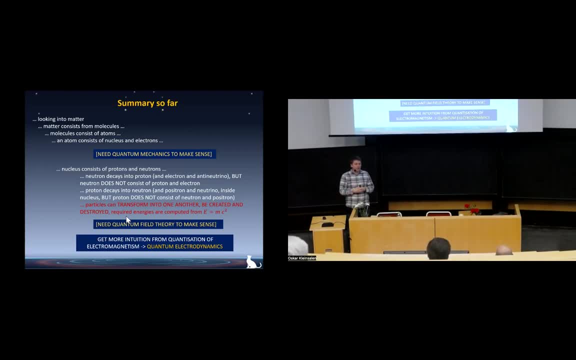 let's speak about nucleus. nucleus consists of proton, neutrons, and now neutrons decays into proton, but and, and, and electron and ethene. but it doesn't consist of these particles, and likewise, proton doesn't produce neutrons. what happens? they transform one to another and they use Einstein's formula to see how it works. 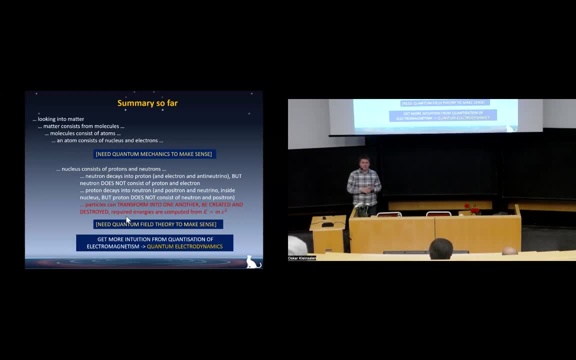 okay, we kind of get it. but what is the correct way to describe everything? well, that is where we need quantum field theory. so it's the next level of theoretical abstraction. so quantum mechanics was one level of abstraction, but to actually properly describe transformation of particles one to another, we need quantum field theory. 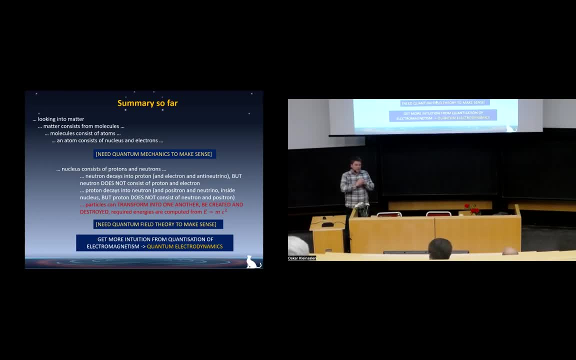 and we get more intuition about quantum field theory from electromagnetism or quantum dynamics. so i think it's a good moment to go to break, and so what we are going to do after this is the break we start. i will try to explain to you what is quantum field theory. 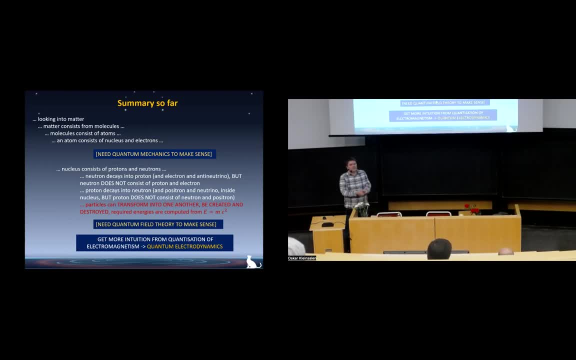 and if i don't succeed, you still stay with me because of that, i will tell you what the github lhc anyway, right, okay. so this first part finished, let's come back at 15 past 7.. Welcome back to the second part of quantum field theory lecture. 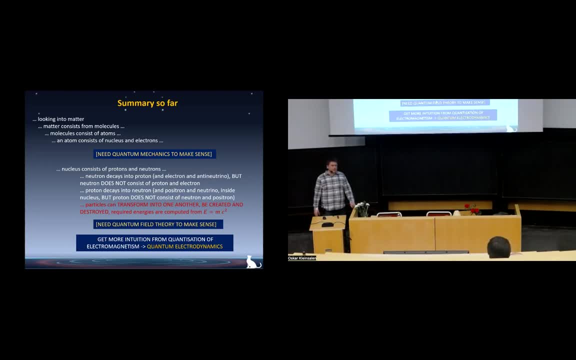 We ended up the same: that we need quantum field theory, and why we do. we need it because we do not have only quantum mechanics, where particle is both. well, everything is both particle and wave at the same time, or, more precisely, it's probabilistic wave which is measured. 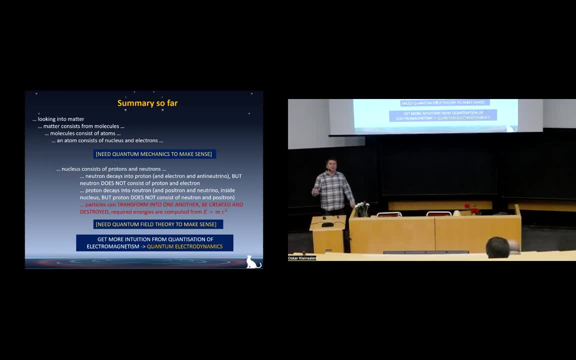 as particle. we also need the mechanism that one particle is transformed into another. this is something that we need. There is one theory in this world where this transformation happens all the time, which is quantum. well, just electrodynamics, because light is always emitted, absorbed it's not. 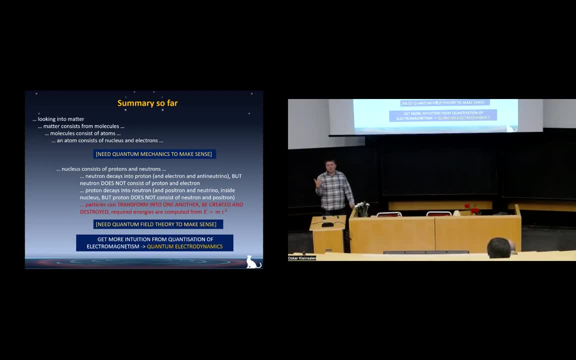 something that this number of light, amount of light is. dark is not something that is present. It's the easiest way to transform energy And this theory was quantized. And to quantize everything else, we actually can follow a lot of analogies. how? 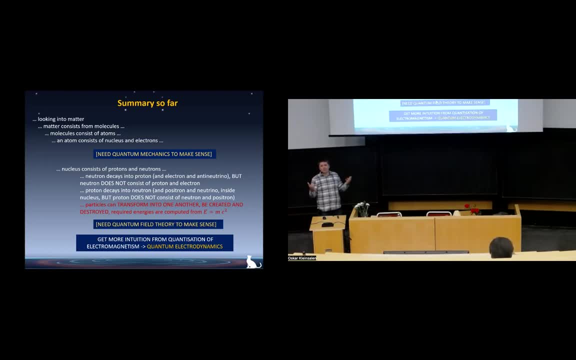 electrodynamics was quantized, Eventually realized that all follows very similar patterns. Our main analogy will be quantum electrodynamics, although I did not insist, But you can always think about electromagnetic phase in your head. So we are going to study quantum field theory. 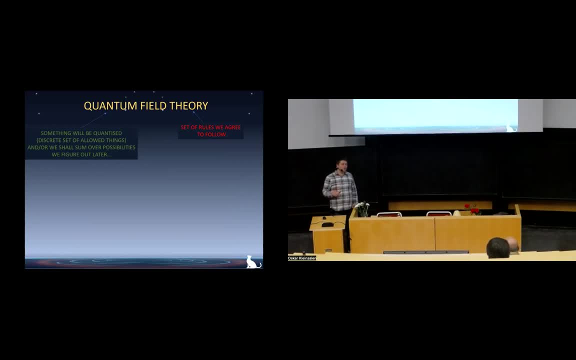 There are three words. Word theory means that we agree on a set of rules that we will follow. So what quantum? Well, you've heard enough of quantum in your life. It will be something about waves and particles. There will be something discrete. 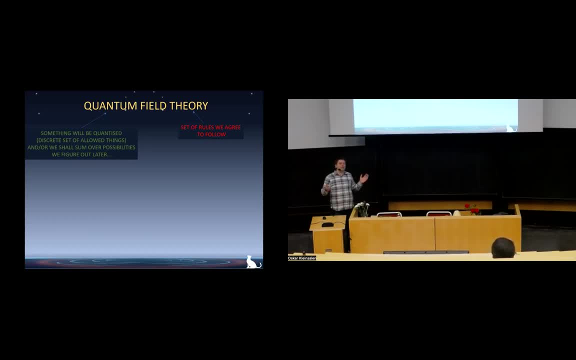 Most importantly, there will be possibility. It will be some overalternation, Alternative evolutions. This is what about quantum? But there is a new word, which is field. Yeah, OK, I mean, is it about that? You know, people use the word field. 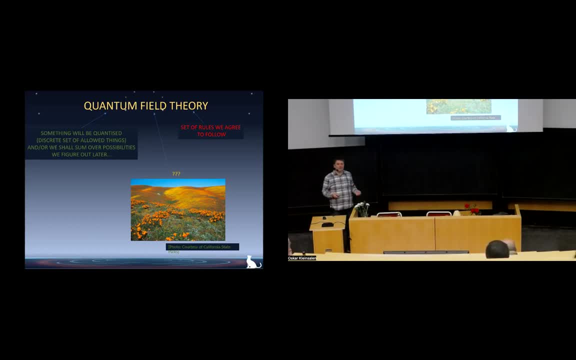 because they were a part of using the word waves, Because they also could say quantum wave theory, but then it will be fully confusing. But it will be. It will be actually more understandable. what they mean So in physics field is actually anything. 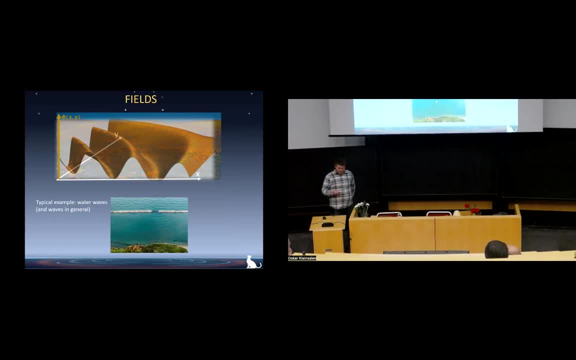 that depends on coordinates. So what we are having here, so if you have actual field, then you introduce like a surface, introduce x, y coordinate system, And in this direction we have something. Well, I just put some height function, call it phi. 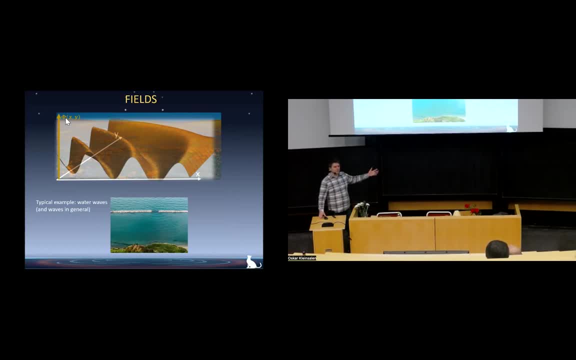 But it can be colors of flowers, smell of flowers. It will, should be. It's parameters that somehow depends on coordinates in which you live. Anything that depends in some way, anything valued somewhere, in principle can be called field In practice, of course, most like most often. 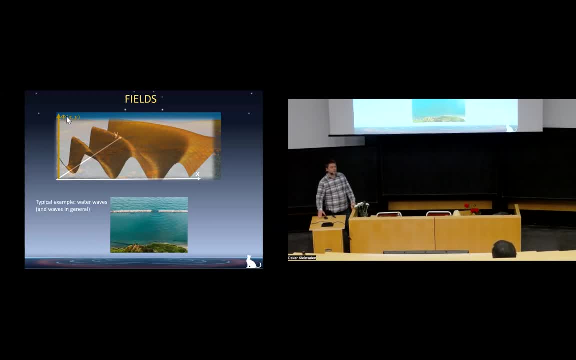 to be some explicit number, complex number. Here it's real, but it's usually complex. Anyway, every time you're confused, think about waves in the sea. It also relaxes. So what field here is actually height of this ripple? 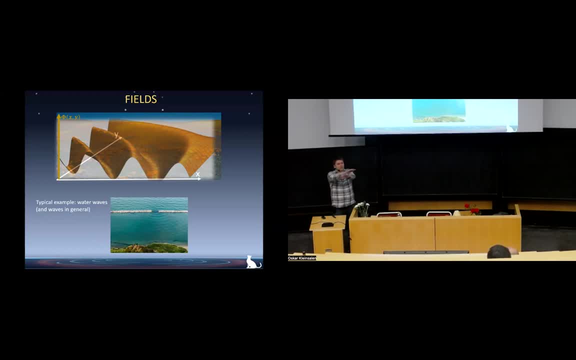 OK, OK, OK. So this is like: when everything is still there is nothing, Then field is 0. When this waves, then field part which is up and some part which is down. Yeah, so if you say waves instead of field, 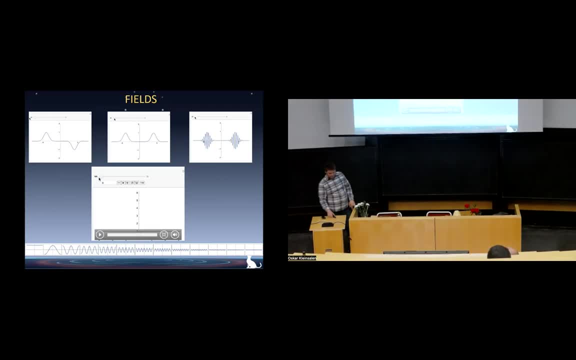 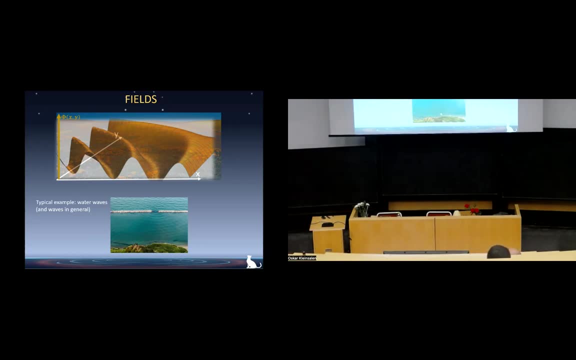 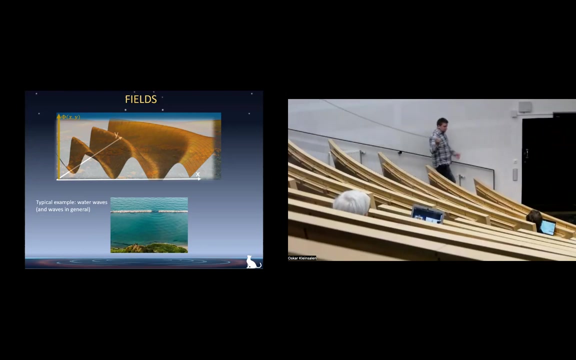 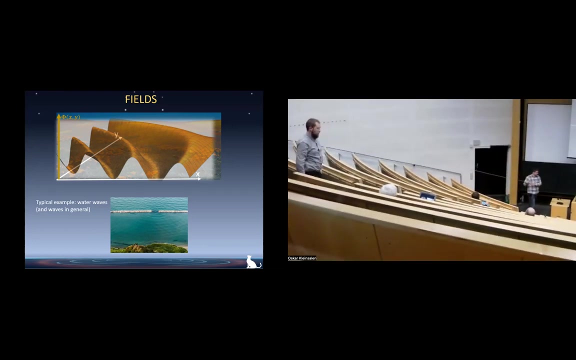 it will make full sense. Before we go to- let's keep nice light- I will show you one dimensional field. So it's the only dimensions that they have is along the length of this spring. So, Sasha, be careful. I fixed it, but who knows? 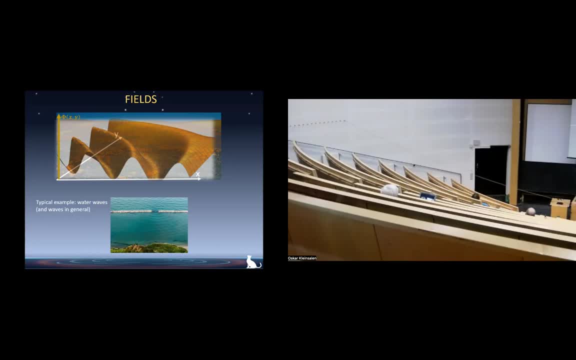 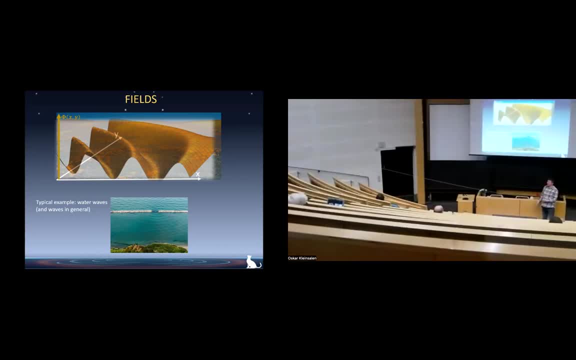 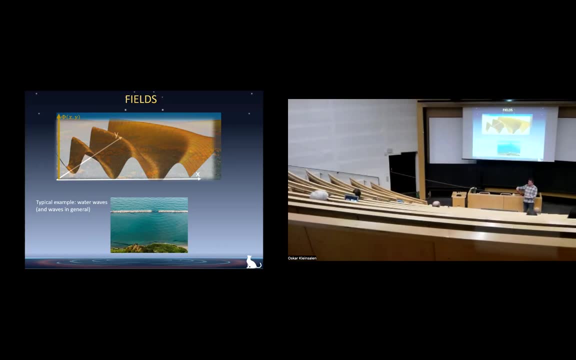 OK, OK, OK, OK, OK, OK, OK, It's a good decision. yeah, So now it's not excited. So field everywhere is 0.. Now I'm going to make excitation of the field, So this is vacuum. 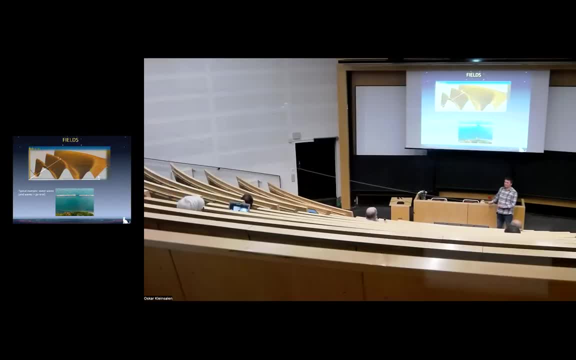 Now I make excitation And it propagates with certain speed, which should be called speed of light for this system, Or if it's a material, it will be called speed of sound, And I can make several excitations. So what I'm doing in mathematics- 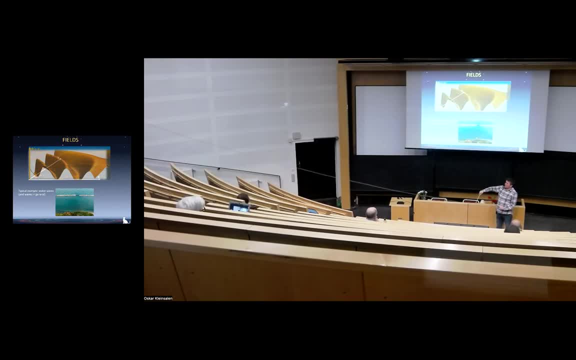 I just put coordinates along this line and plot the height of- I mean how high it was- excited. This is an example of excitations which are transversal to the propagation of a wave. So, yes, this is a wave, Signal propagation is a wave. 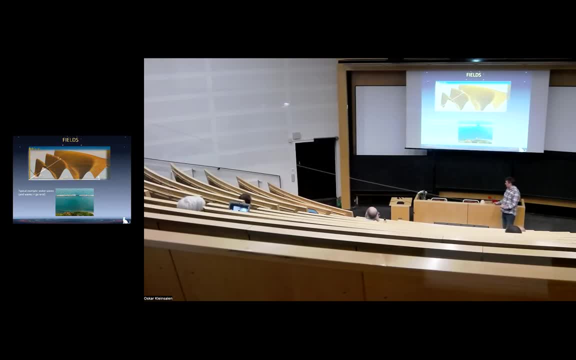 Yeah, boom, boom. And this is an example of transversal excitation. Actually, there are two ways to do that: Like this And also like this. This is more dangerous one. You can make a superposition, You can rotate. 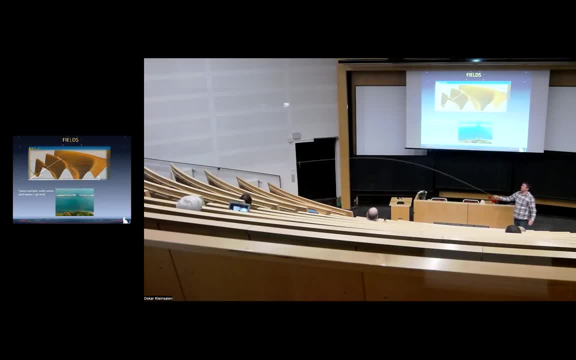 You can also make standing waves. I will try to make higher frequency. yeah, Standing waves. You see It's actually. there are nodal points that do not move. Okay, But this is example when we have one dimension Here it's two dimensions. 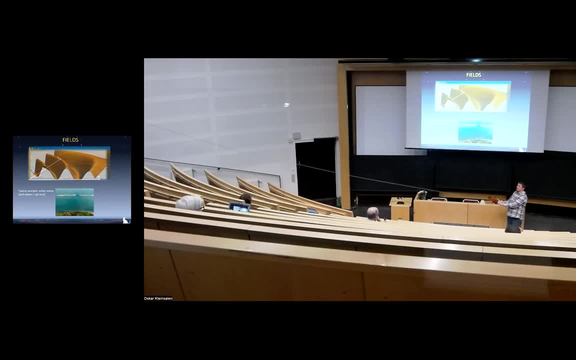 Here it's only one dimension, But we have actually two possible excitations, This direction and this direction, And we can make actually they form a vector-dimensional vector, We can make a combination. So this is example of transversal excitations. 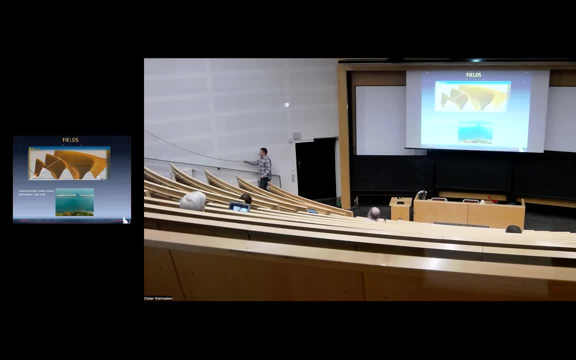 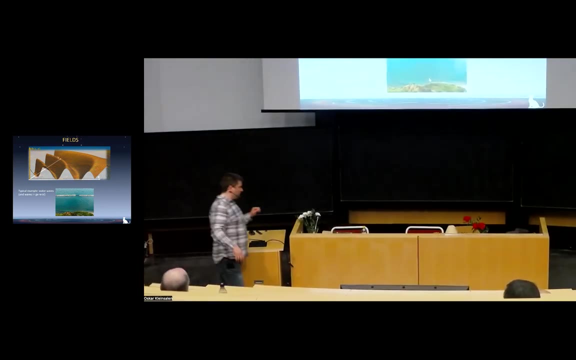 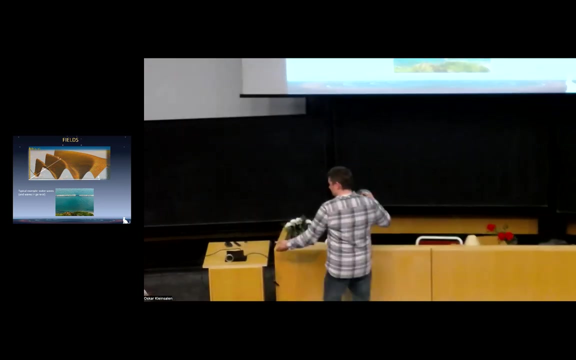 And these are most important for us today. But in nature, sound waves, for instance, are not transversal. They are actually in the same direction as their propagation, And for this I have another example of a field or wave, Uh. so the situation you can see here. 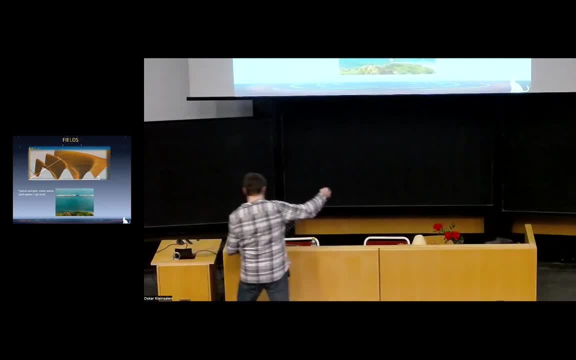 where the signal is this way. So this is a wave And this wave is very, very, very, very, very quickly decaying Because of friction. So because of friction it will very quickly decay, but still you can see signal propagation. 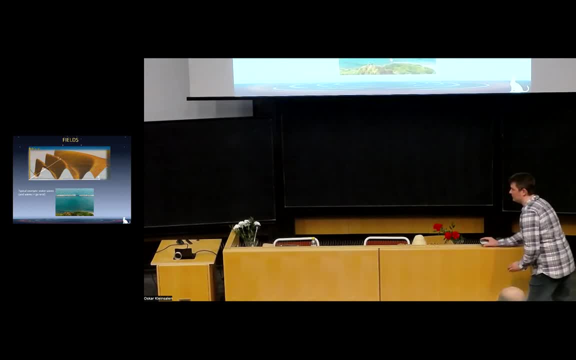 So you see, excitation is the same direction. So you see, after this problem, if you can also see the signal propagation, it will be in this direction. So then your scaling the current signal propagation. So you see, So you see. 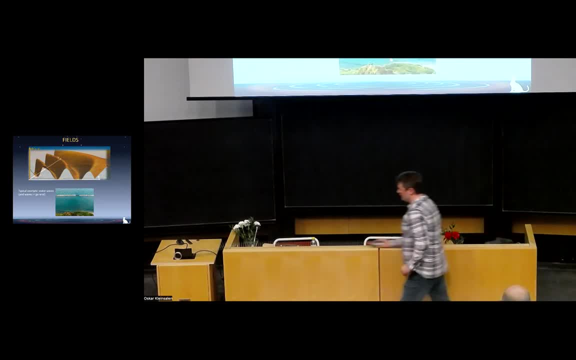 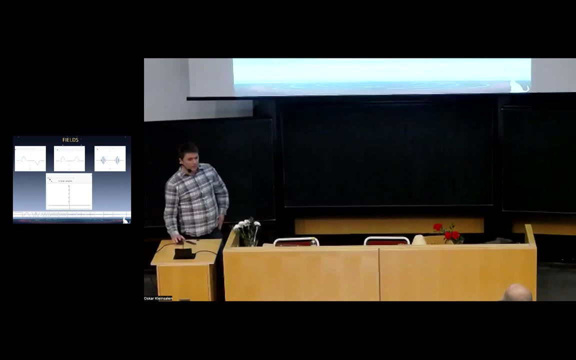 And so you can see. So this is the opposite direction. This is longitudinal signal propagation. So all the fields can be understood on these analogies. Important part about fields is that if you have one excitation, another excitation you can add. 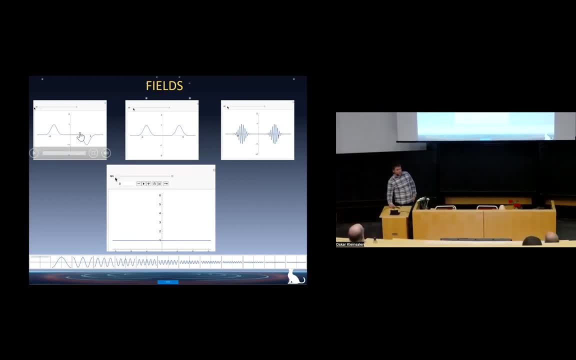 So, for instance, here we have one bump and on this rope I showed you another bump opposite direction, And so when this bump moves they actually add up And this is an example of destructive interference. I mean, actually, in English it doesn't make sense, it's just. 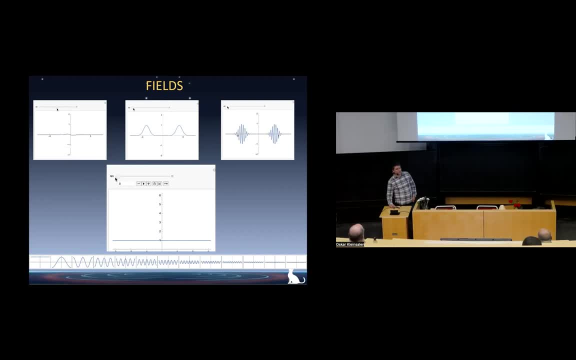 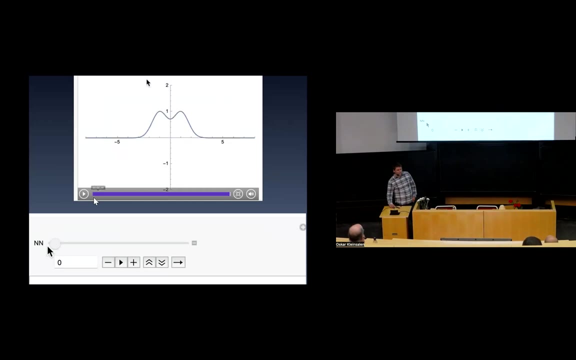 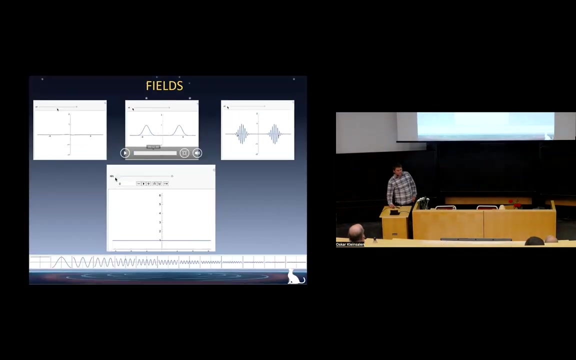 interference. There is no constructive interference if you use English as a native speaker, But nevertheless people say destructive and constructive interference, Like you see. so actually waves can cancel away and be nothing, Or if they're in the same direction they become bigger, right? So usually when you have waves you have some oscillations. 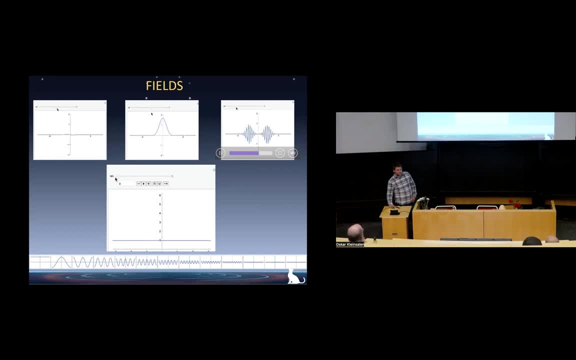 so things look more interesting. something like this: And now in reality, we can see. we can see that the waves are moving in the opposite direction. So we can see that the waves are moving in the opposite direction. And now in reality, we can see. 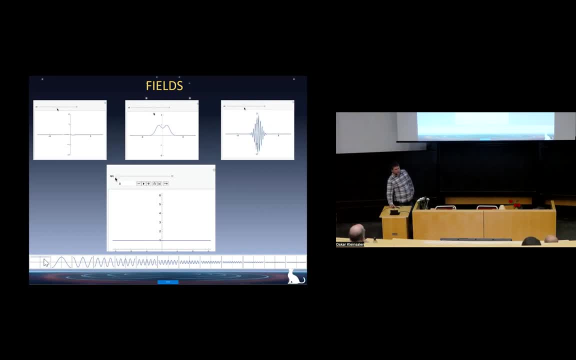 have very many different oscillation modes. So for instance, here I took 12 different oscillation modes. So this is constant, this is one peak, this is two oscillations, this is three and so on, And they actually exponentially decrease in amplitude, so become less and less. 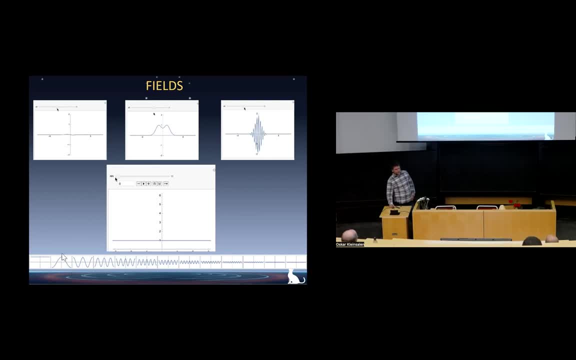 So now I am going to add them up all together. For the moment I didn't call the first one, but then this zero is on the first wave. Then I make a sum of this guy and this guy- two of them- When I make sum of two of them. it doesn't work this way. 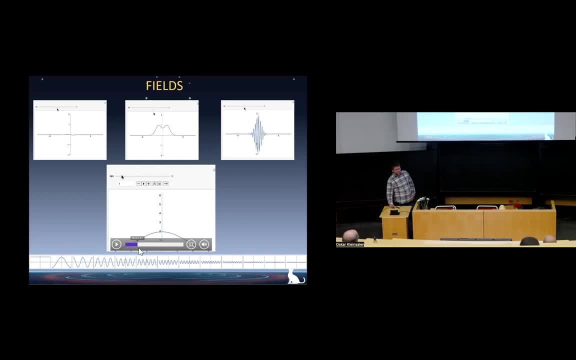 This is one, so this is sum of two, this is sum of three, this is sum of four, five, six, seven and sum of all. So look, this were all waves, like a sine normal, sine function, oscillated normally. 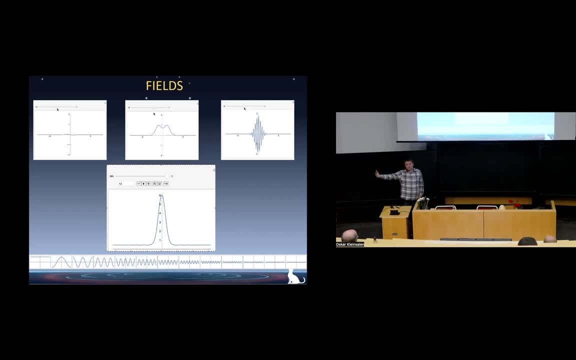 But when they add them together they form something that doesn't look like oscillating stuff, it looks like just a bar. This is something local in time. So by adding up waves, adding up fields is called superposing. I mean they use different words superposing. When we superpose them we can make some bumps. 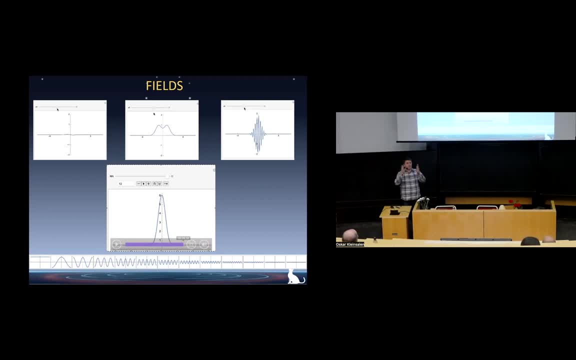 And this bump sometimes can be interpreted as localized particle. It's in good place. So if you have this bump you can say: okay, this particle more or less has a different position In mathematics. decomposition of this bump into signs of gain: frequency. 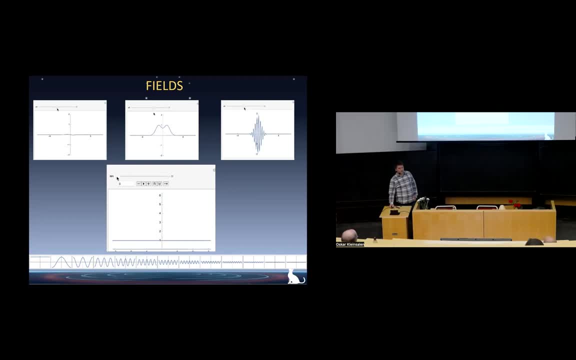 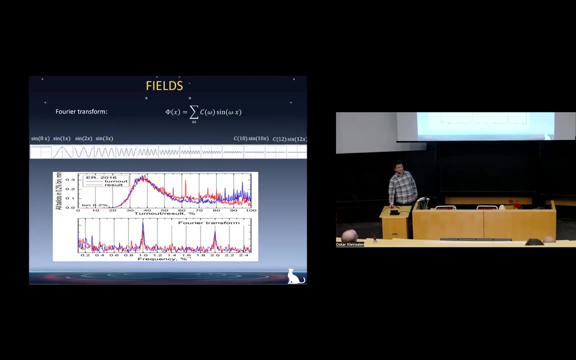 is called Fourier transform And there is important mathematical statement that any function can be written as a sum of a sine function. So we have to sum over all possible frequencies. So for instance, this is sine zero x, this is sine one x, sine two x, and so on. 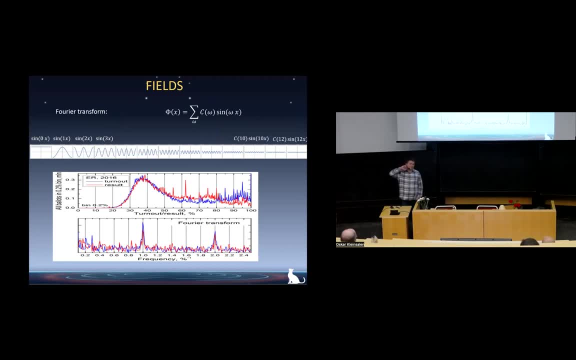 Our ER is a very good Fourier analyzer, So we receive signals And here decomposited to frequencies is how we understand music. I actually forgot on the break. we can try with a oscillogram on computer And you can think of every song and see what frequencies do you have? 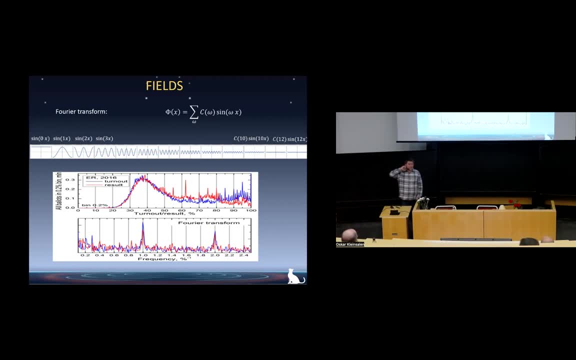 It's actually a very fun exercise. We're not going to do it now. And Fourier transform is useful for many reasons. For instance, when I was speaking about statistical physics, we were discussing how we can check that elections are falsified. So, for instance, let's take about 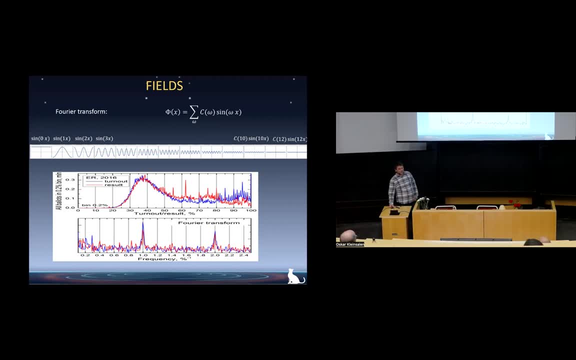 let's take, for instance, blue line here. So it's election 2016,. certain elections And in this direction, how many? so blue line corresponds to how many people did show up in a given. there are many different voting polls. 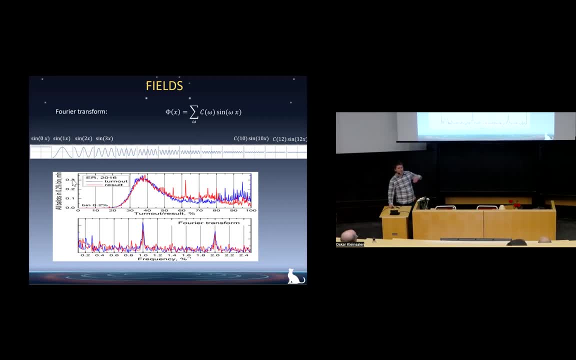 And number in here. it's like a percentage of voting polls that had this number of percentages of people that came compared to the maximum amount. So turnout can be 40% of vote maximum. 60% of vote maximum and different voting polls will have different turnout. 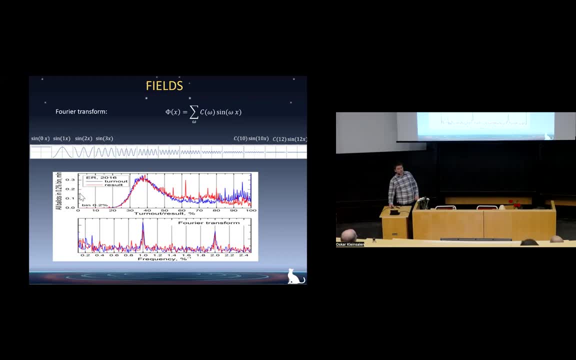 And so if you plot the number of people coming versus turnout, versus number of polls that have this turnout, this will be this blue curve, according to data which you can find line. So what you can. now the question, what you can do. you can make Fourier transform. 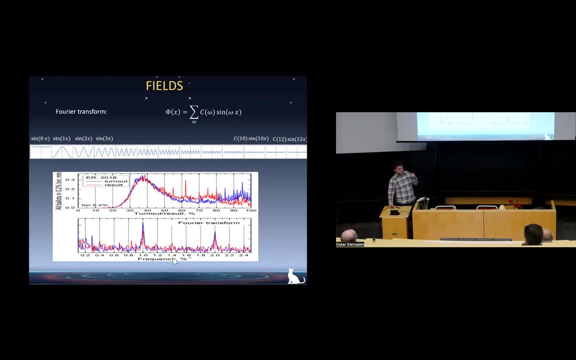 and when you do Fourier transform, then you see that there are peaks at 1% inverse and 2% inverse. So it's means that here the steps of one and two percent of one and 1.5% of the most probable. 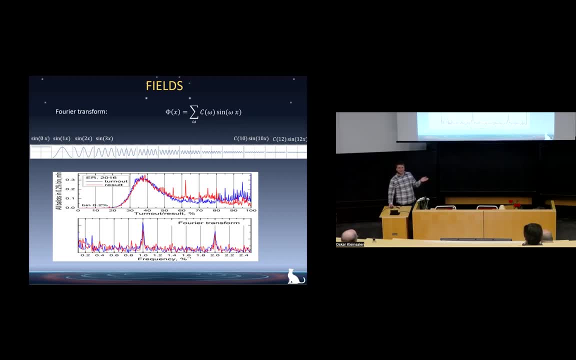 Well, this means that it was quite aggressive, was fabricated data, because steps and integer is improbable if you do honest turnout for elections. So these two peaks just tell you that this data was fabricated. This example of usage, Fourier transform, Anyway. so when we speak about field, we are going to decompose it into frequencies. 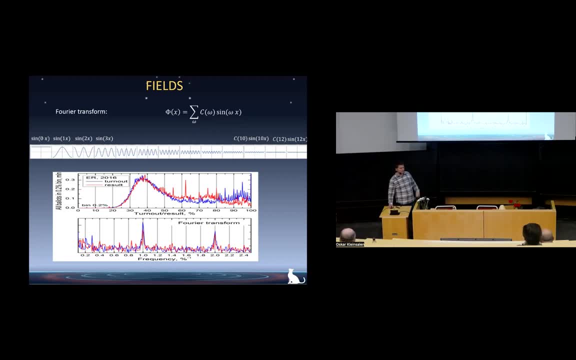 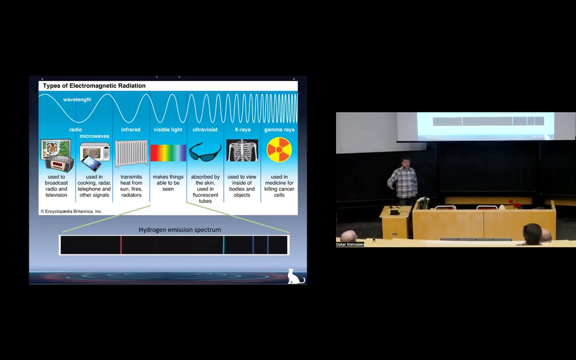 into sine waves with some coefficients and we will focus on these numbers. now This will be. I will see what it will be now. Decomposition to frequencies is light. it's used a lot. So colors is light of different frequencies If you go to lower frequencies, so long wave lengths. 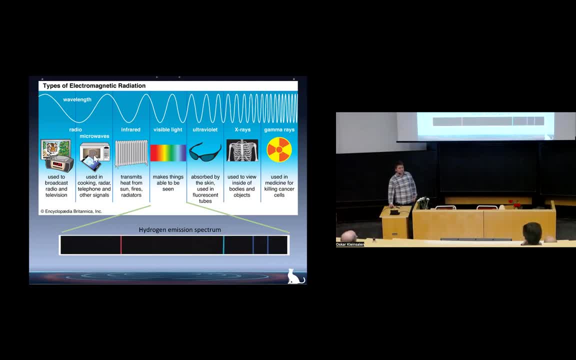 you have infrared, so you have what you have in mobile phone and microwaves. And if you go to high frequencies, like very often, that's why you have x-rays- the one we spoke about, that's Rutherford fault- And gamma rays, which is even high more in genetic radiation. 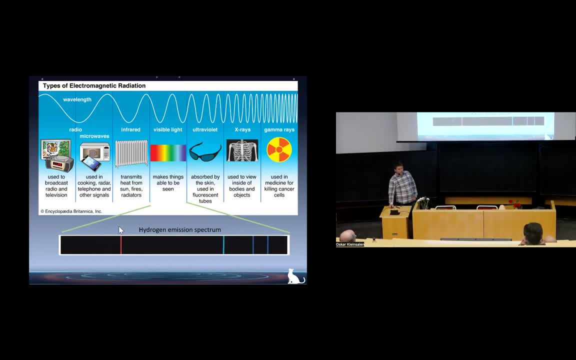 All right. so the hydrogen spectrum, or emission spectrum, lies here in this. well, I mean, it actually lies not only here, it's infrared and ultraviolet. just you do not see it, but visible part is here. So decomposition of light into frequencies or wavelength states, it's very typical things. 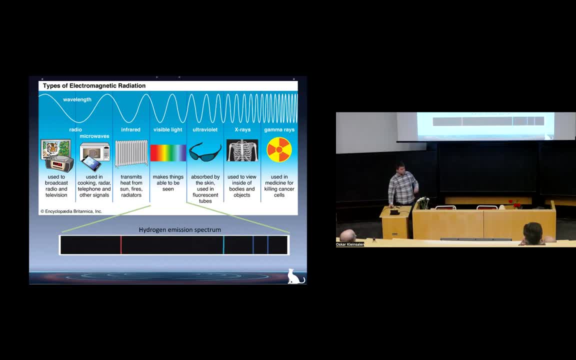 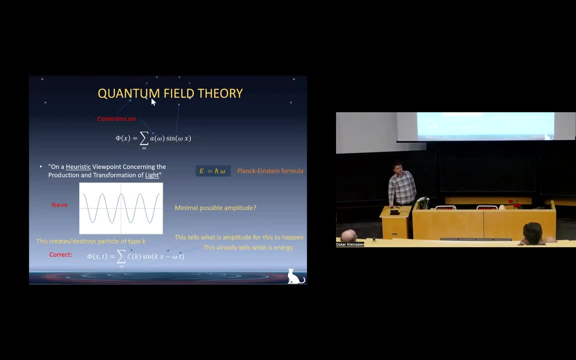 we do all the time. Rainbow is example of this decomposition, Anyway. so this, I tried to explain. what is field? Now coming back to the question of quantum. So quantum, at least naively, will put constraints on this. now Values, and here we come to the third out of four papers. 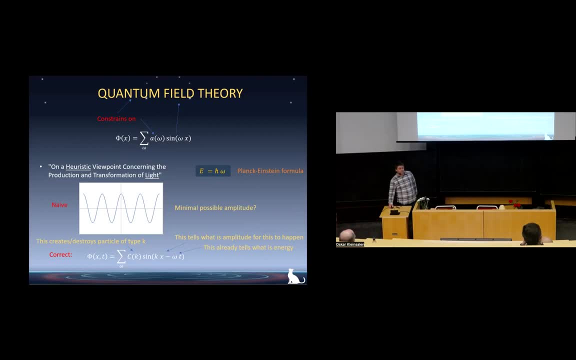 claimed from Einstein. So the first one is about Planck-Planck formula. So energy of light can be only so photons have energy equal to one constant frequency. this frequency here one photon, and you have two photons. If you put here two, then it actually means that you have this wave. 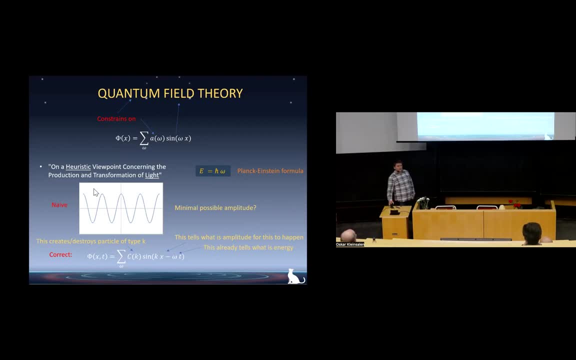 and you have exactly the same wave twice. this will be two photons. So like, very naively, what happens is that if you have this constraint, that energy equal to this number, this means that these bit, this is like first impression that you have from quantization and then you say, okay, uh well. 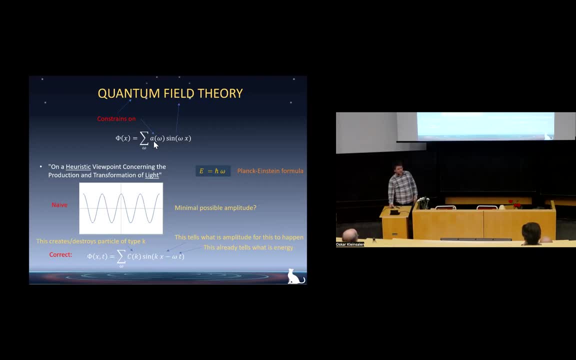 classically we know that energy for wave is square. of this height. this is classical result from. so what does this mean? if energy is constrained to this number, it cannot be less. it means that there is some amplitude. the smallest possible amplitude in the wave cannot be smaller. 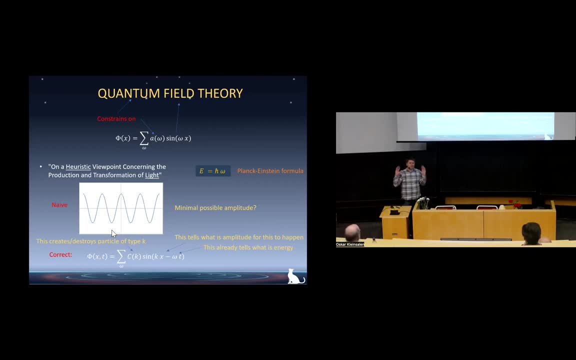 but this is against objective denial of quantum mechanics. so we cannot actually draw this picture in quantum world, because to be able to draw this picture, we should be able to measure it. but we definitely do not measure this picture. so this picture in reality doesn't exist in quantum world. so there is no such thing as 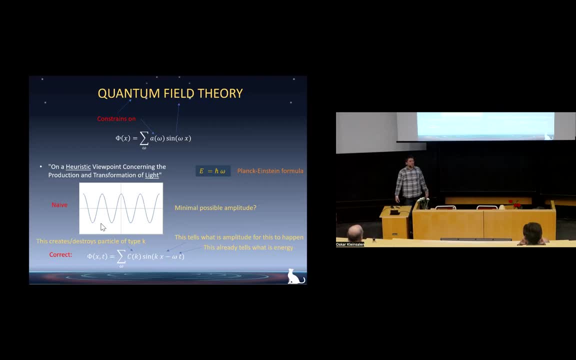 minimal possible amplitude. a bit a bit, because there is no amplitude in this sense. when you measure, you measure something else or like locally. so correct interpretation is actually quite astonishingly surprising. i did not tell you everything. i just told you that we have coordinate dependence, but in reality also have. 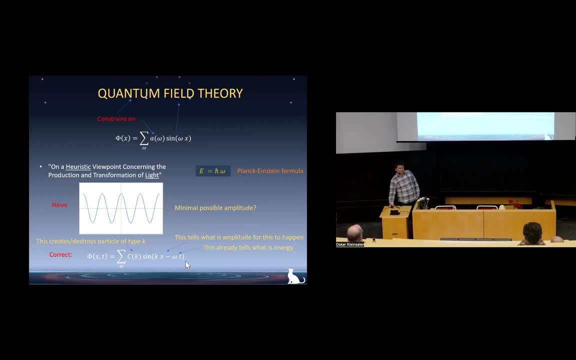 time dependence and actually coefficient- and this we were going to discuss just in a second- this coefficient in quantum world already tells you, regardless about this coefficient here- already tells you that your wave has energy h, omega, because energy is related to time translation. okay, and this coefficient- here i should be a, here it's not even a number. 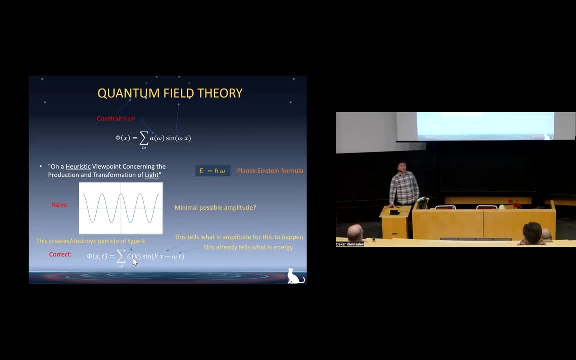 in quantum field theory, this coefficient stopped being a number. it starts to be operators. it creates or destroys photon. so what is written here? some of our all possible photons. we are going to create or destroy them. this will be their energy and this actually controls a probability or amplitude of probability. 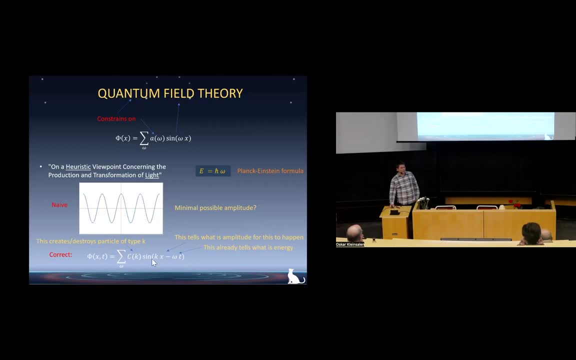 for that to happen. this is a meaning of the quantum field and quantum field theory. it's some of our all possible things that can happen. but remember that quantum mechanics is about. we have to consider all possibilities. some can happen if you want to do it, but at the 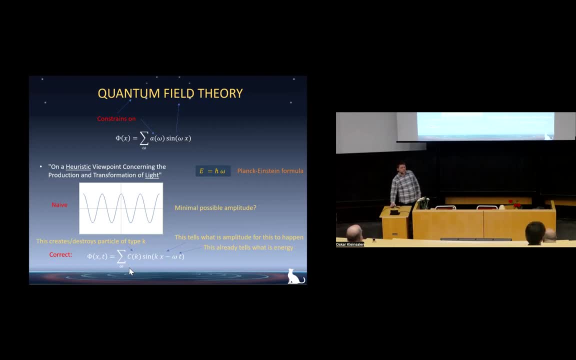 sums them up with certain weights. that's what we're doing here. we're summing up over all possibilities to create photons. this k creating photons, as this kx, tell you what is amplitude, what is complex number associated to this event, and this omega tells you what is energy of the 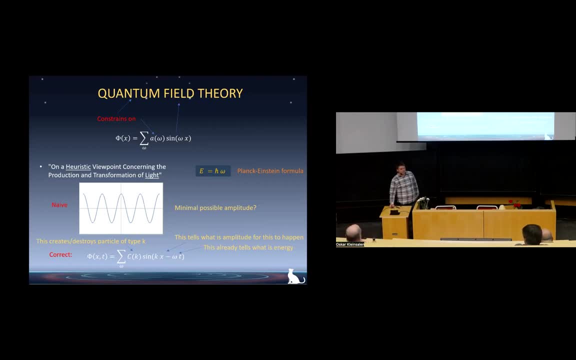 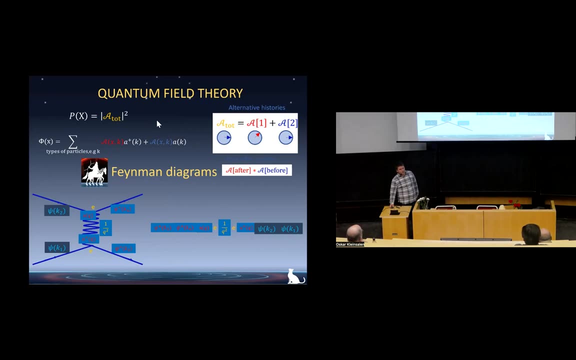 corresponding field. this is what is quantum field. so, and here, actually, it's explained a little bit more clear. so again, so remember that probability of something to happen is absolute value of a square, and this a is computed to sum over all possible histories and this error. i wrote it. 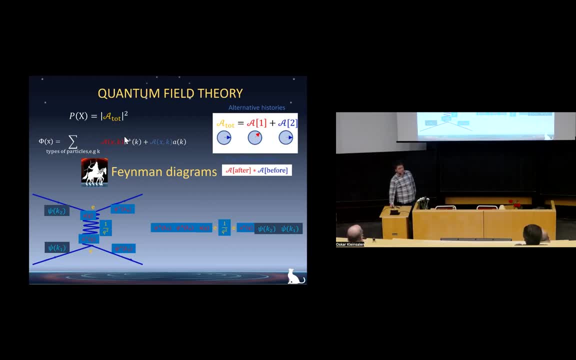 again. so the vr actually will be two types of thing: possibility to create something, this amplitude. so let's say that his red history is history of creation of particles and blue history is a history of you destroying particles. and quantum field is us is sum over all histories. 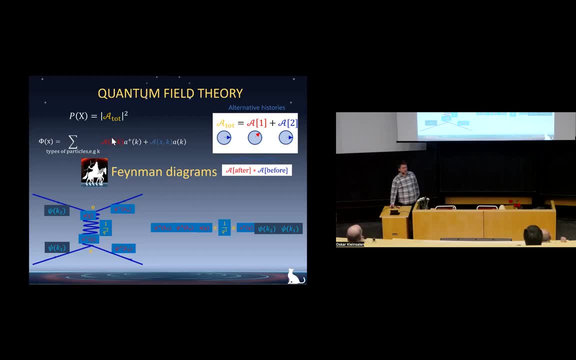 this just said that particles was created and this is amplitude for that to happen, and this is: particle was destroyed, and this amplitude was this was to happen. so this is what is quantum field is well, and now i- i should have done this- i cannot not draw from. 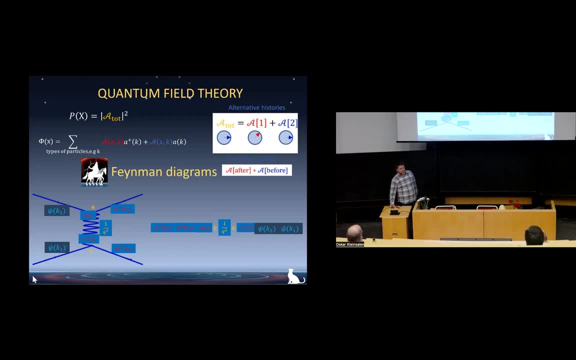 another diagram, right, to explain what it is. uh, so famine diagrams is actually. it's so this odin, so odin on the thing here- is holding fremant diagram. this is his hand, right, it's a tool to travel across the nature, but what does frame integrity means? 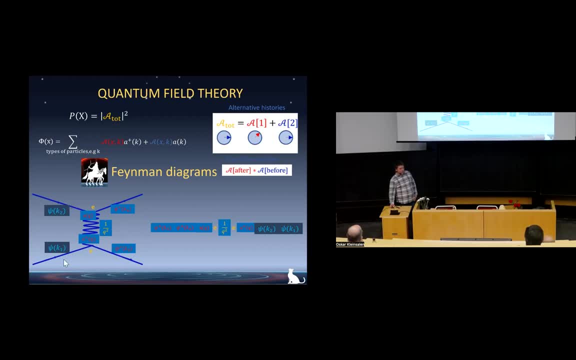 well, uh, so this is example of electron Scar. so we have two electrons, uh, and in simple words, two electrons fly. this electron emits photon, it propagates here, it's been absorbed to this electron. they fly away. But how to make it mathematically? So we want to ask question. 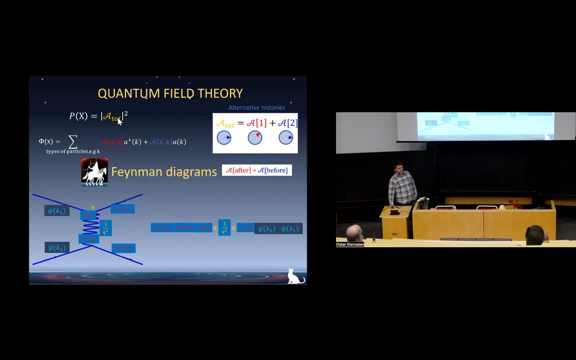 what is the probability of this to happen? Or, more precisely, what is amplitude for this to happen? Because if you know amplitude, probability is square of it. So what we have to do, we say okay. first of all, we were given conditions that particle did exist. 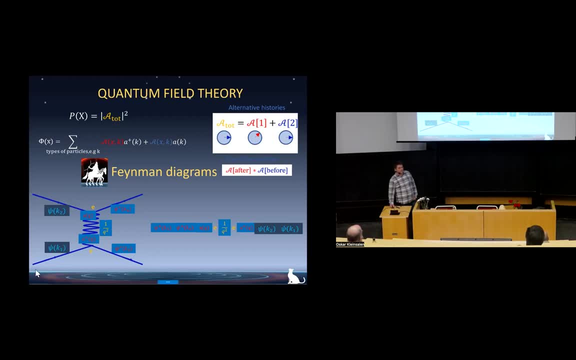 and they still exist here. So if particles existed, this picture says that. okay, actually we're going to destroy them. so there is no plus. it means the destruction of particles and psi derived because of the electrons, so electrons that you don't want to. 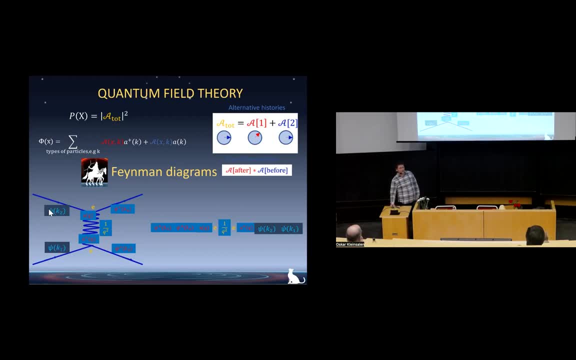 e, not a. that's one different thing. So we are just-. So this is just saying we are going to destroy this particle, so nothing else. and here we say we are going to create a flask photon with momentum q and also create another particle with another momentum, k3. and when this 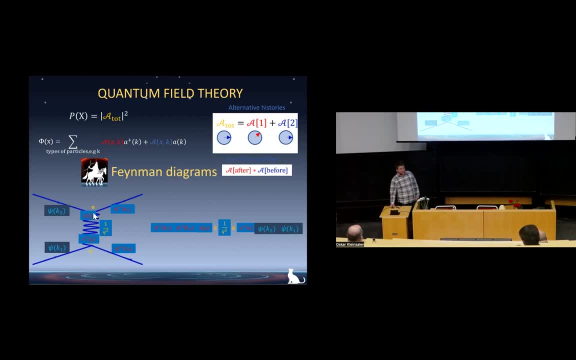 photon arrives here, we are going to destroy it and create another particle. so this is destroyed. destruction of particles, creation of a photon, destruction of photon, creation of particles. and finally, uh, two more things here we have: e is electric charge and it's actually number, uh, this amplitude, number associated to amplitude of probability for this to happen. so you have to. 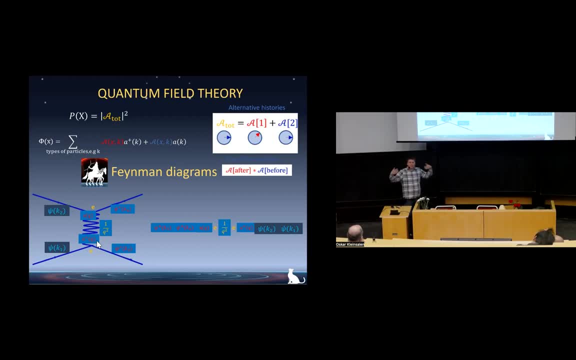 write some over all things that can happen in the world. but then you have to assign numbers for each thing to happen. so amplitude for this particle to destroy it and photon and another electron being created is equal to a number which is called electric charge, and amplitude of propagation of photon from here to here is equal one over q square, where q is its momentum. 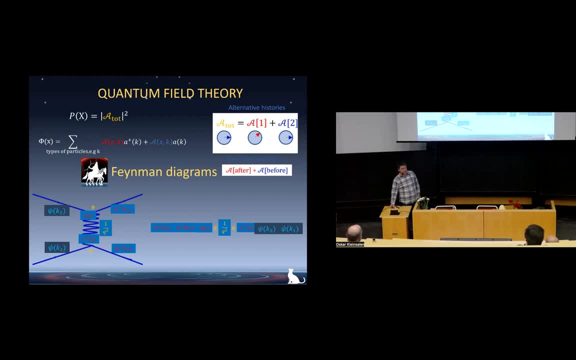 uh, and then you just write everything together and you do a computation. so if, if, if i do everything correctly, you'll get column potential here, but of course i skipped quite, quite a bit of things. but uh, for those who knows, fourier of one square is cool potential. this is the most important part. 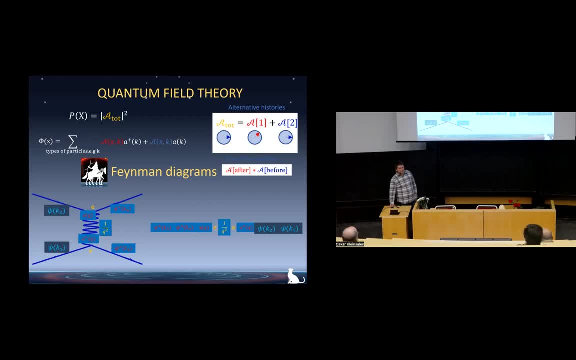 of it. uh, i mean, there are a lot of decorations which you have, but look just here. we killed two particles, created photon with this problem probability with amplitude e. it propagated with this amplitude. uh, then a photon was killed and two for toilet was created with somebody. so this is what was behind the hemograms. uh, if you understand, 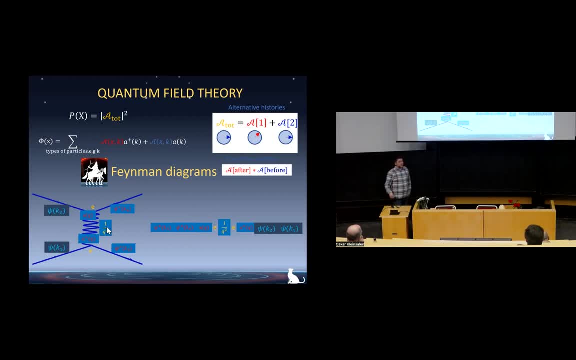 this principle great, and that's unreal computation. just a lot of decoration around, which is unpleasant mathematical stuff, or it might be pleasant if you like complicated mathematical stuff. it depends, uh, what you like. but it's a lot of a lot of indices. it will be quite. I'm not going to show it well. computing of frame. 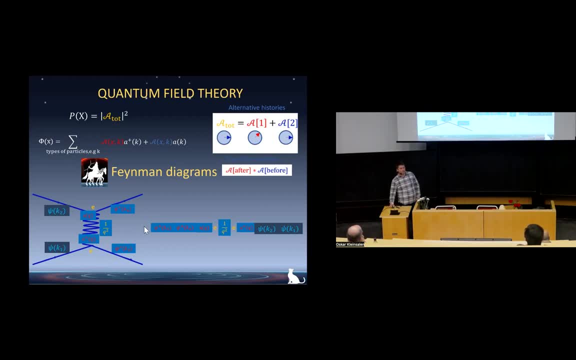 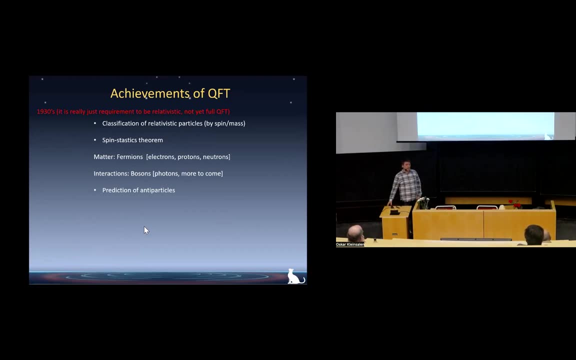 diagrams is the basis of like for perturbative quantum field theory and this is what people did. and what is the achievement of qft? there were two important, more precisely quantum dynamics. there were two important errors: 1930s, when actually was not really still qft seriously. 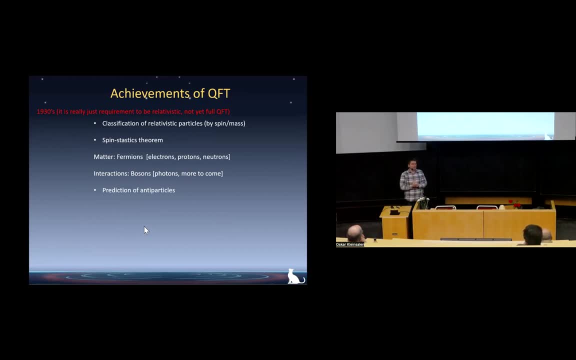 it was basically applying Einstein theory of relativity to quantum world, and I want to discuss with you one thing seriously and the rest thing not seriously. I want to discuss with you seriously classification of relativistic particles. I probably will go to the slide which I need for this here. 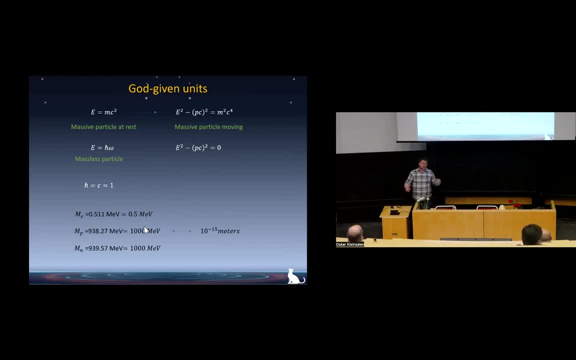 don't look yet. look at me. I'm going to tell you something. so I told you we're going to do quantum field. now I'm focusing on theory. I'm going to declare for you the rules of the game. so rule number one: we are going to be quantum. this means we are going to compute amplitudes. 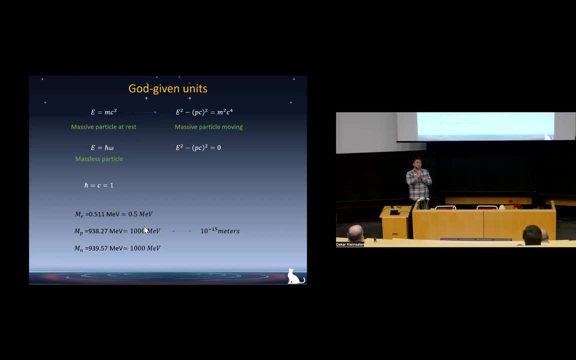 using quantum rules and rule number two. we are focusing on sample. rule number two: now we are going to say that we believe in Einstein special relativity. what does it mean that? so in uh, instead, principle of relativity says that if we translate our system, that we just change our. 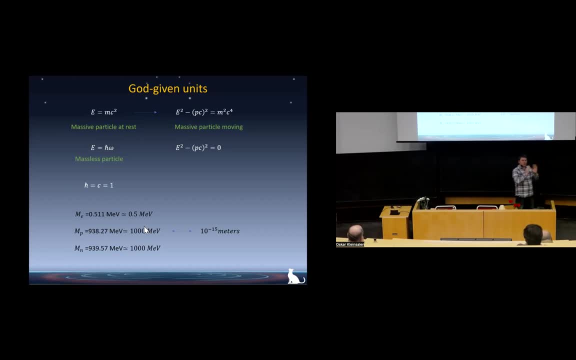 coordinate and go. so as we change our coordinate system here, description should not change. it says: if we translate in time, it's, it's worth translation in space. I cannot show translation in time. Well, probably have to go to sleep for this, I don't know. So if it translates in time, 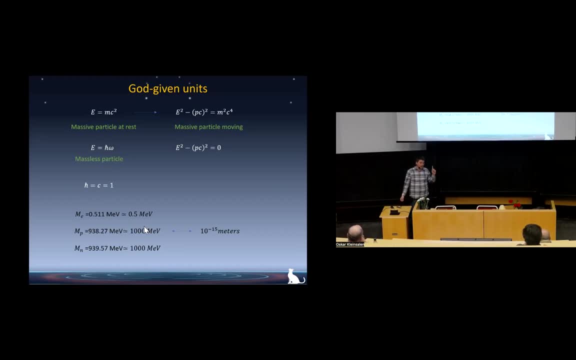 description will not change. It's another symmetry of a system. If we rotate, description will not change. There are three ways to rotate. And finally, if you boost, description will not change. Boost it means we're going to reference frame which moves at constant speed to respect the 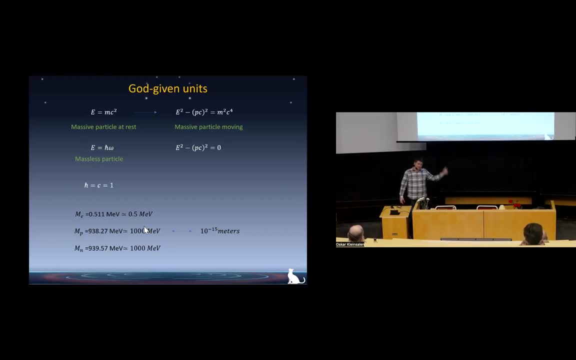 reference frame that we have now, So we can translate in space, translate in time, rotate and boost. And we say that we want quantum mechanics which satisfy this property. And already this is enough to give you a classification of particles. Well, not like you will see what I mean by this. 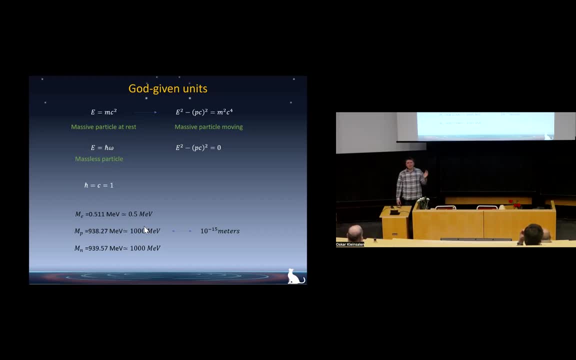 Invariance under the selection in time. this is important. This is a theorem in physics that tells you that the particle would have fixed energy that is conserved. So energy is something always linked to time, So a pair if time is a symmetry. 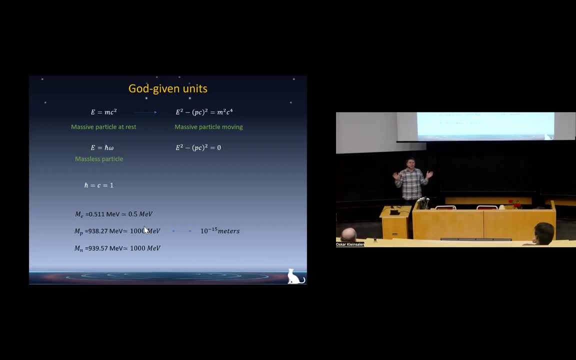 then energy will be conserved. So every particle in this setup will have fixed energy. Translation in space tells you that each particle which has momentum MV, basically in classical, in monorelativistic world, momentum of particle which is conserved, conserved, So energy moment conserved, invariance under boost will mean that this combination. 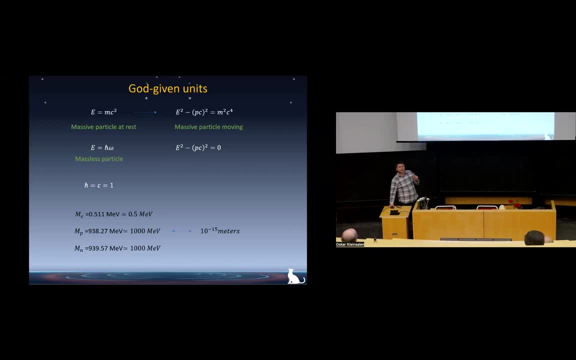 of energy and p is the momentum. this combination will be constant. This is what does it mean? invariance under boost, And in special architecture this is called computing interval Or it's like. it's like Minkowski-Pivogorian theorem. This was what Sasha was telling us last time. 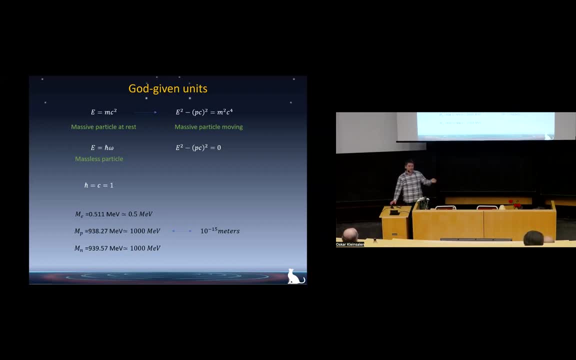 And because it's a constant, this constant should have physical significance, and its physical significance its mass, square times C4 of the particle. So mass of the particle is a constant that appear in this combination, which should be constant by. So we already 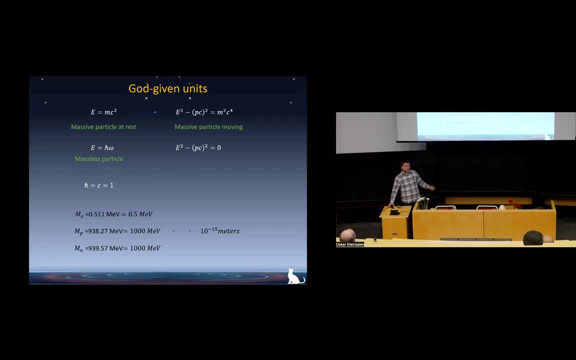 know that particle has energy momentum and this, their combination, gives you mass, so it can also have fixed mass. Then there are two types of particles: Massive when this is nonzero, and moderate. Massive when this is nonzero and moderate. Massive when this is nonzero and moderate. 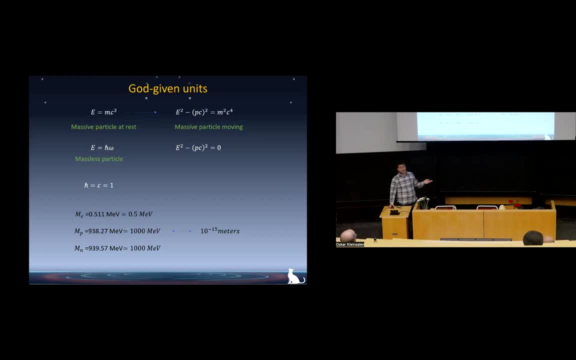 massless and this is zero. Both particles exist through the world. If the particle is massive, we cannot find reference frame, so then it doesn't move, Then this is zero. and this formula reduces to famous Einstein formula: E equal mc squared right. So if this is not here, then you take: 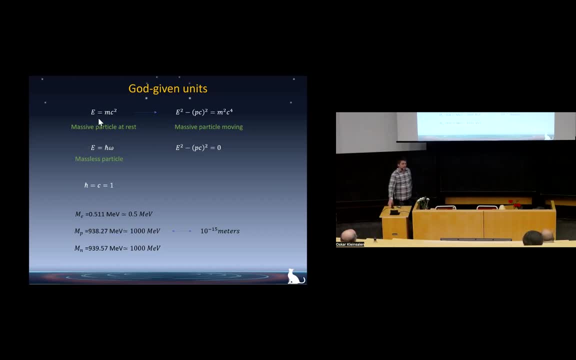 square root. on both sides, you get here. So Einstein formula is actually a particular case in this more general relation. And if particle is massless, you cannot find frame where it stands still, Massless particles always move. Moreover, they move with the speed of light. 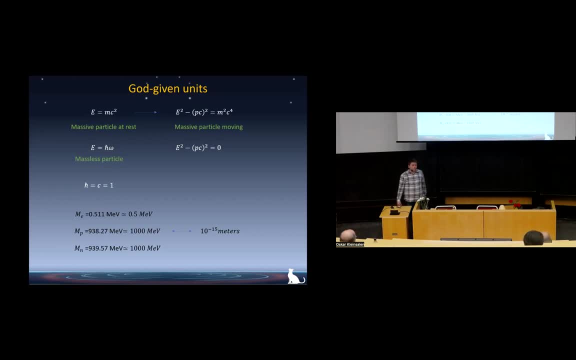 always This, just always: speed of light. In this case, the energy can be found using Planck-Einstein frequency. In this case, they should be waves like no other wave around, and this will be So, by the way, this on the left. so this was the smallest clear on classical world. 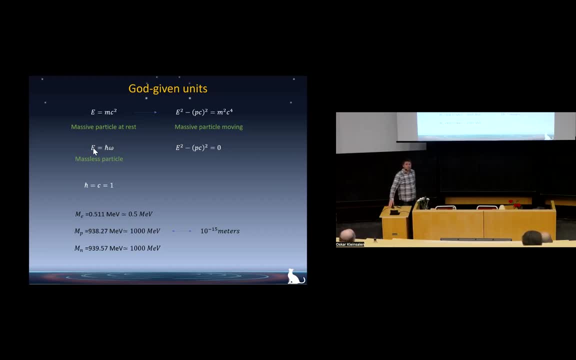 but in quantum world- it was understood by Wigner- It's 1931.. And this tells you that particles has mass energy, momentum and all this property exists. And then also, after we all see all this, it's a good moment to introduce God-given units, because 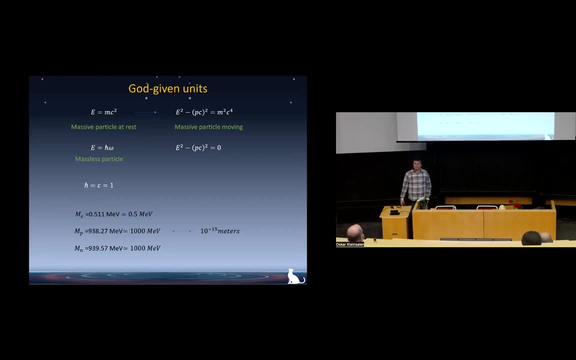 like taken with you for the whole of your life: H, bar and C everywhere in the place. it's just, it's coming. I don't know, not boring, but you are tired to do. it's becoming tiresome because well. 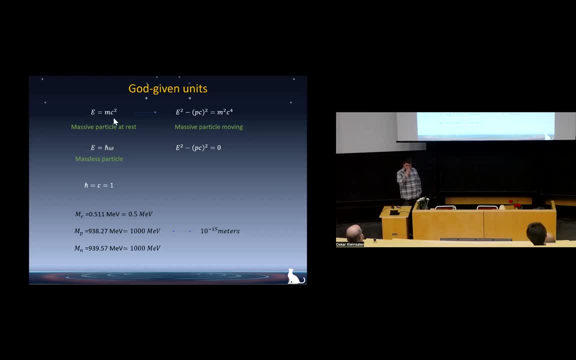 you just write equal, equal energy, equal to mass, And the moment you do this, you actually can measure masses of particles using energy units, and that's what is done in particle physics. You remember what is electron, What is electron? What is electron? 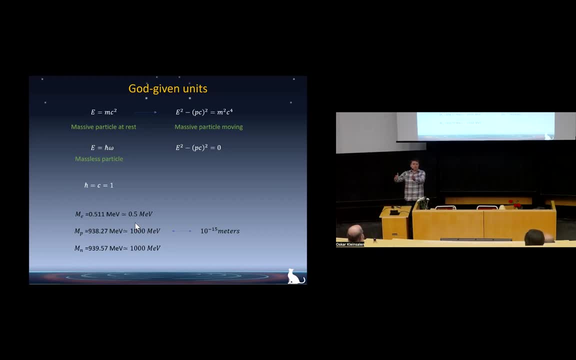 volt. i had this device here. so electron volt is energy that's achieved by electron, by bison, through potential. one volt now, because it puts equal to one energy, is also used to measure mass. so mass of electron is not one little point, it's electron voltage is a feature of charge. 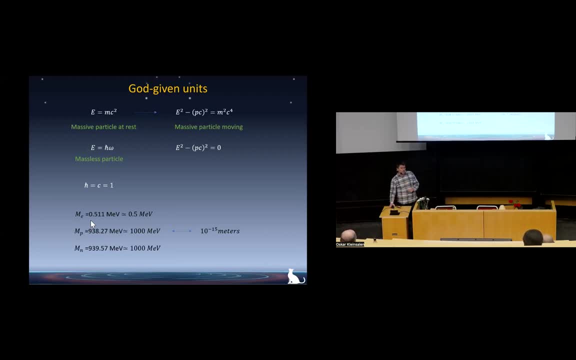 not of mass. mass of electron is actually 500, 000. it's quite a lot, but proton is still 2000 times harder and actually. but well, so frequency is one over second. so energy is inversely proportional to units of of time. but also when c is equal to one, one meter is the same as one unit of time. 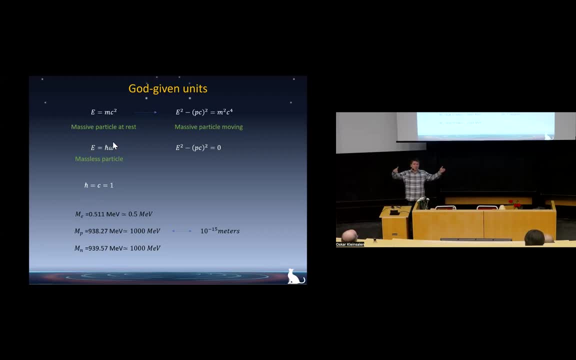 so energy and the and distances are inversely proportional to one another and and you can compute that uh, uh, related to this energy, you have size of 10 to the power minus 15 meters, which is topical size associated to prot. that's slightly more complicated. uh, i mean it's complete conclusion, reality more difficult, but 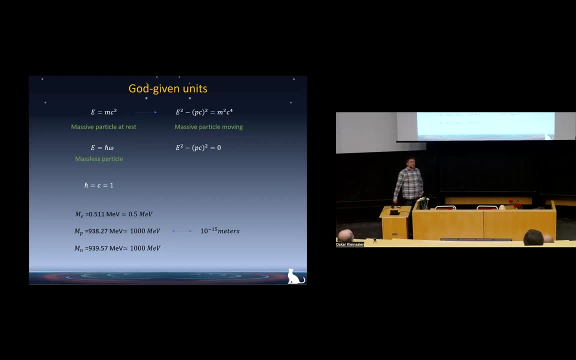 it actually works. i mean, for instance, you should not explain, uh anyway, so basically what you follow, now i will always write masses of particles using energy, select on voice. that's what is doing happening in, in, in, in Szene and outside accelerators. uh, right, right, which symmetry law did i forget? 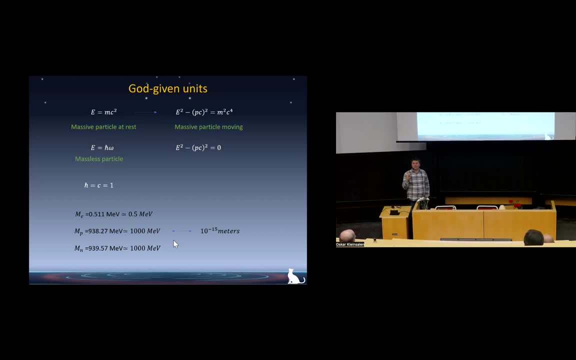 i did not use all symmetries. yeah, i did not use rotation. i use translation in space time and also boost change in in space time and also boost change in velocity. so boost gives me this formula, velocity. so boost gives me this formula. there's also rotation. 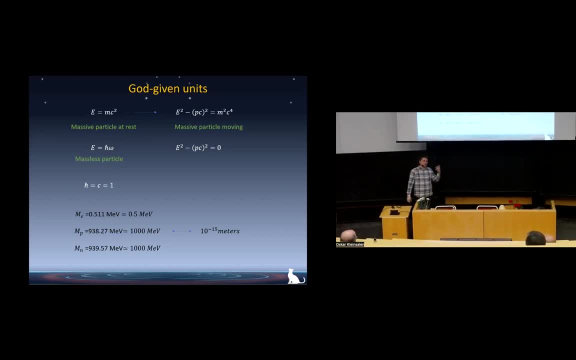 So particles are interesting because a priori particles do not have size, at least, I mean, if they're elementary they definitely don't have size. but if they're compound they can have size, but if they're elementary they don't. and rotating point-like particles is pointless, right? 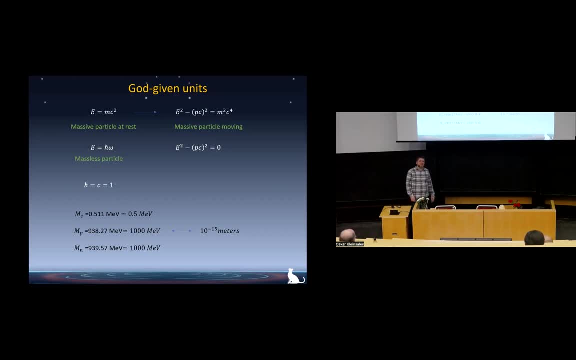 I mean, we cannot rotate the point. Nevertheless, particle can change under rotation and the way how it changes is called spin and it's a mathematical description. and so, in the case of massive particles, you have spin. in the case of massive particles, you have helicity. 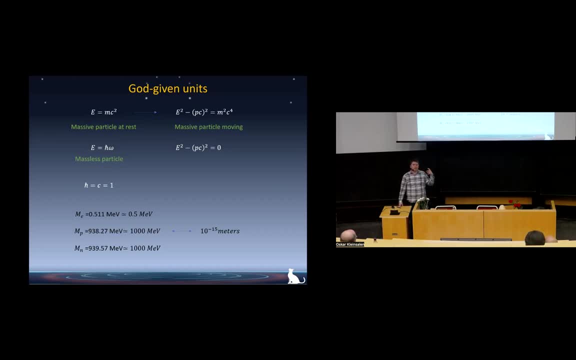 So let's speak about massive particles. So spin, it's fin, It's a picture of how particle changes when you rotate it. and there are two types of particles in the world: those who have even spin and reality. well, we have zero, one and two. 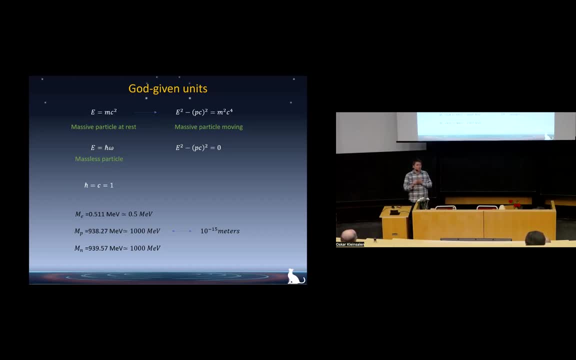 Zero is Higgs boson, one is photon, and also you'll see what else, and two is gravity. Sorry, I promised to speak about massive particles. Well, anyway, almost So. these particles are called, well, the integer spin particles. they're all together called bosons, and there are half-integer particles, which are quarks, actually proton, neutron as well, electrons, also neutrinos. 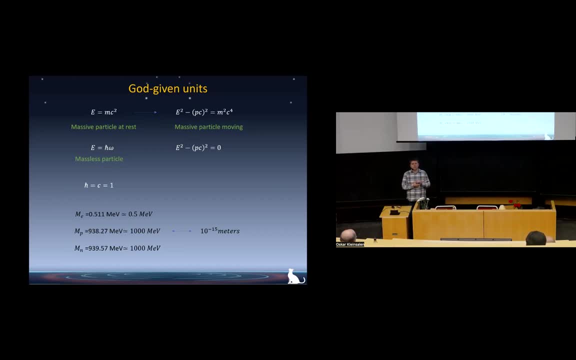 This example of half-integer particles- all they are named- actually have spin one-half. They are all called fermions. So what is important about bosons and fermions? So bosons, so in quantum world, particles, are indistinguishable. 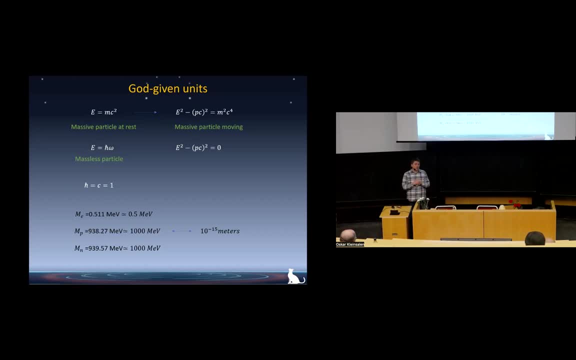 Bosons they like to. but the difference is a fun: that bosons like to be together in the same state and you can accumulate this number of bosons together in the same place And bosons will be the guys who transmit interactions. 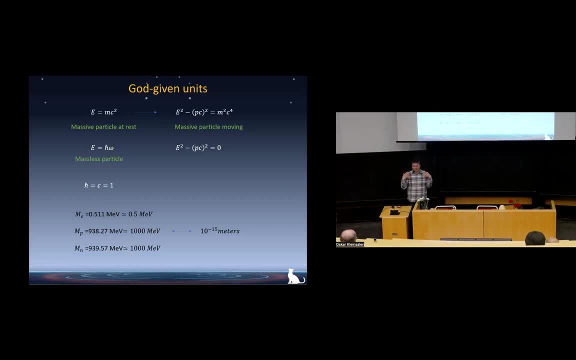 So you can actually can make it very strong flux of bosons and create quite strong interaction And electrons or fermions. these are particles that do not want to be in the same state. They always want to go by different states And this is very important to create better around us. 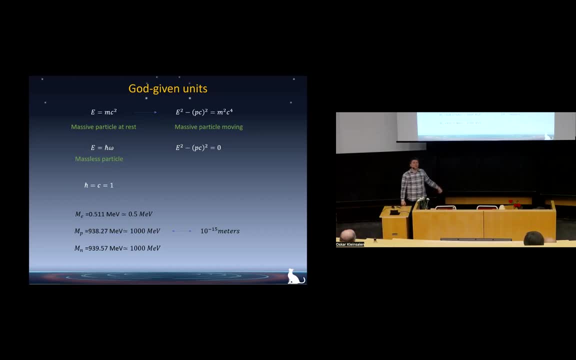 So I am not falling through this table, Or maybe I do, Because electrons from my hand do not want to be in the same state as electron in this table. So creation of massive matter- and not massive but like voluminous matter- is a fact that matter contains fermions. 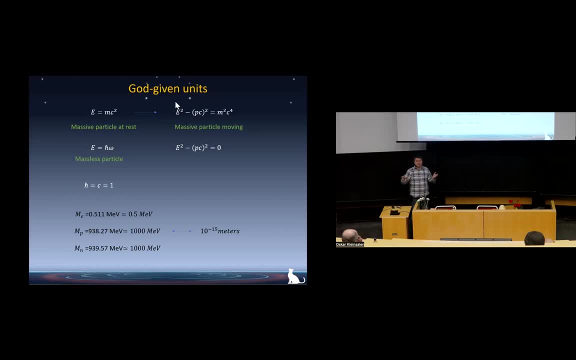 So we have two teams: Bosons spin zero-one particles and fermions spin, one-half elementary and three-half can be another spin. So this is what I call spin-statistic theorem. it's very important. So this was early, so I told you about early achievement of part of the theory. 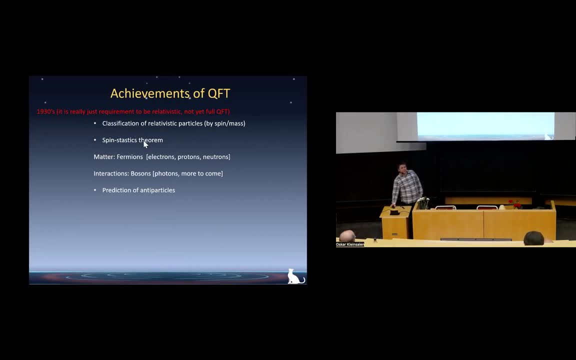 We got the idea about classification of relative particles. We split them into bosons and fermions. Fermions form matter and bosons form forces of interaction, And also a prediction of antiparticle happened. But this is actually was the easiest part. 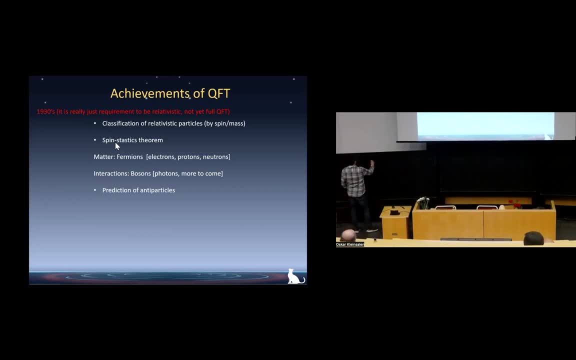 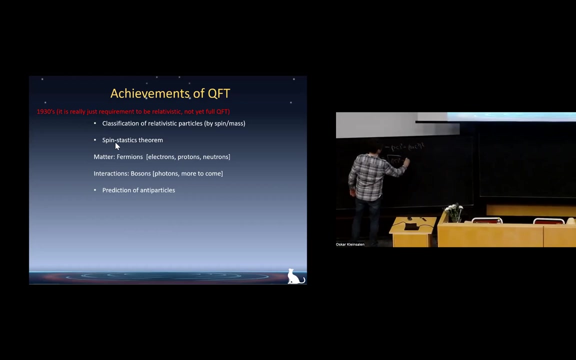 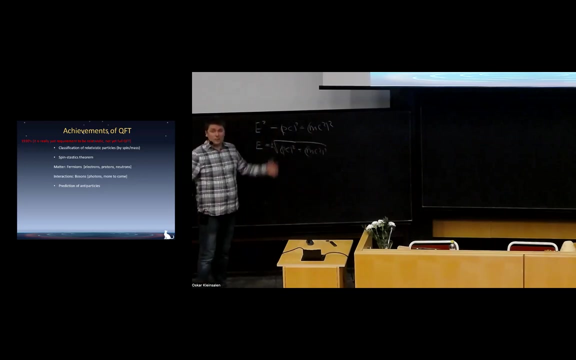 Because, as you say that when you write this formula you know, you probably know how to solve quadratic equation, You can have two signs and you have to do something with this, And so negative sign eventually can get interpretation of antiparticle. 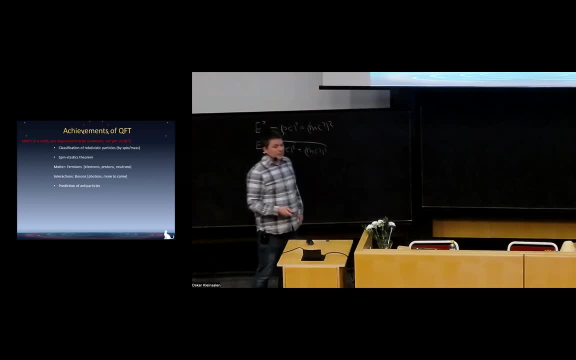 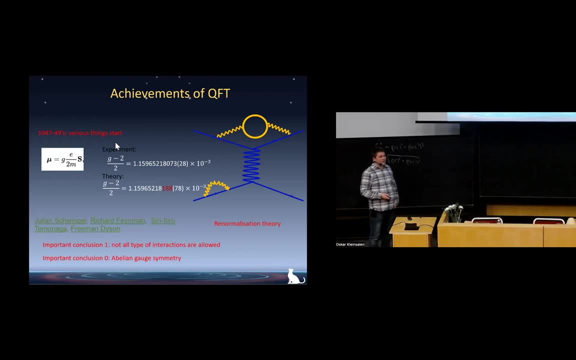 And so negative sign eventually can get interpretation of antiparticle, But I'm not going to go into details about this part. So this was the easy part actually of quantum field theory. The real stuff happened about ten years later. 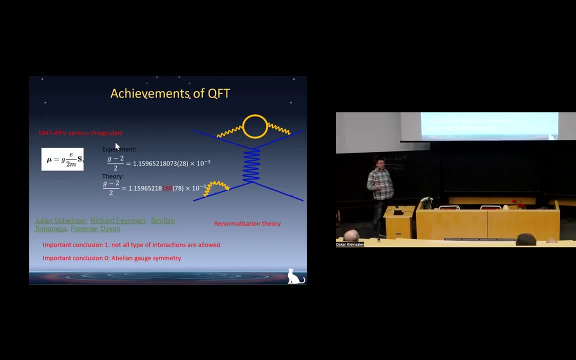 Because when I told you that you have to sum all overall possibilities, you actually really have to sum overall possibilities. And it's not only that electron flies emits photon and this photon is received by another electron. And it's not only that electron flies emits photon and this photon is received by the other electron. 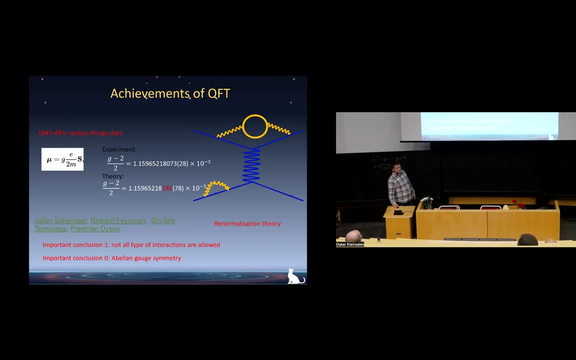 can emit another photon and this photon can emit electron and positron. electron positron pair a, which called vacuum polarization, electron, positron fly around, collide together, make another photon come back, or electron flies, emit photon and this photon comes back to the same electron. it's yeah, so uh, and there is thousands you can write i, i mean, thousand is not like. 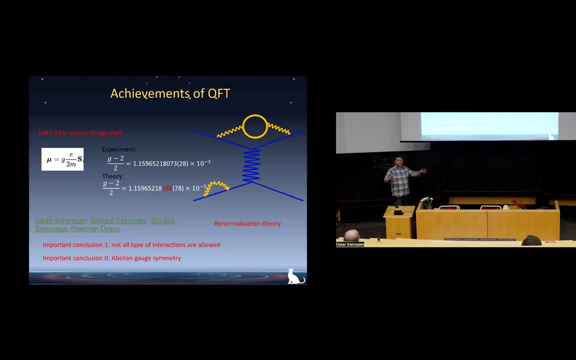 abstract, i mean it's combinatorially big number, and people who do these computations, they suffer from this. uh well, this one savior. every time you write this, uh, three particle place, you have another value of electric charge appearing, and two values of each other together called. 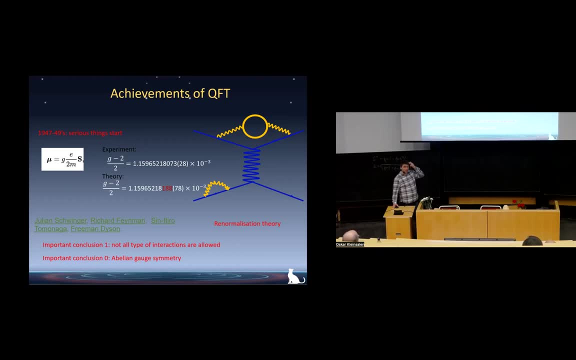 fine structure. it's one over 137, so every time becomes smaller and smaller. so writing two, two massive diagrams is uh, is becoming less and less correction. that's why we can make precise computation. but there is much bigger problem that if you sum overall possibilities here, i mean so here when this photon emits electron and positron. 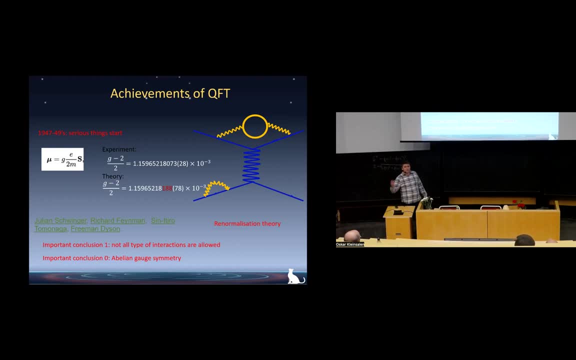 they can be of any momentum and if you integrate overall possible momentum you actually get infinity. there is infinitely many possibilities, so real computation will give you infinity and people struggled for many years to subtract two infinities together get finite number. this is called renormalization theory. so 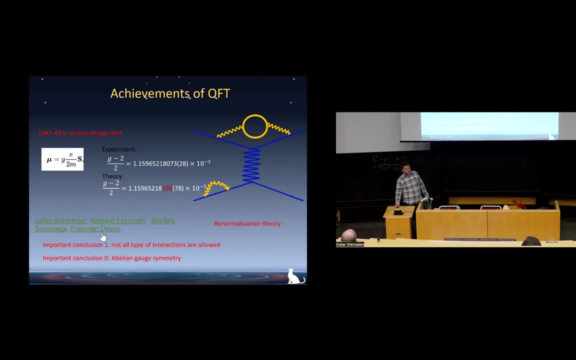 this gentleman did this job, famous finger to monogic. what noble price was this? and they explained how to subtract infinities. important thing to understand, to remember now that it's possible and there is some terms that it is possible- and after you did a lot of work, you can. 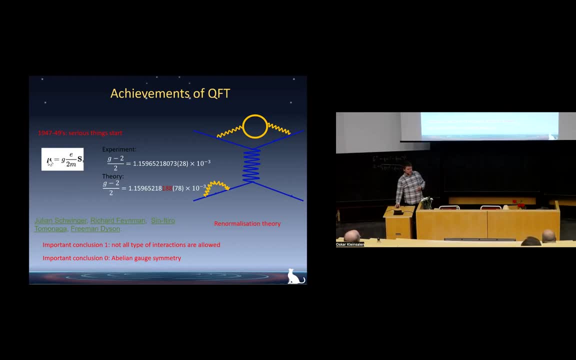 predict this number, whatever it is, is. it's a spin of a particle, this is magnetic moment. uh, so this is experimental value and and this is theoretical computation. so all these digits like one, two, three, four, five, six, seven, eight, nine digits, much so. quantum electrodynamics is actually the most precise. 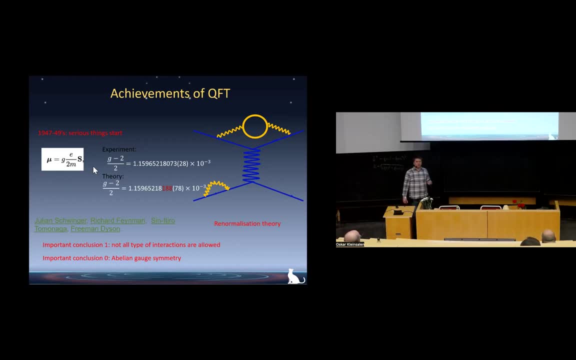 theory existing in nature. none of the theoretical computation can give you 90 to which 90 decision function and the more data you get, the more you can easily imagine this experiment. quantum electrodynamic does. this was really a huge achievement. all of the field and after you see this matching, you really believe that it is corex theory. 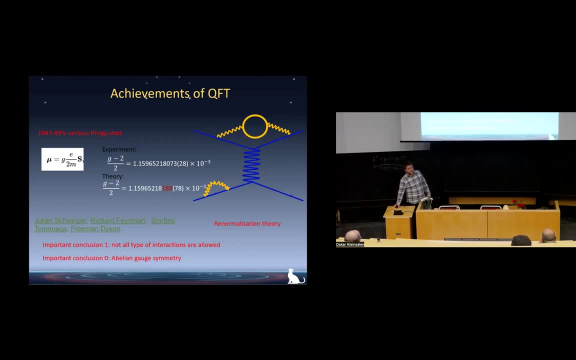 there are two important conclusions, uh, one conclusion is to get this uh secret word: normalization. not all interactions will be allowed. will allow myself not to explain what I'm not allowed, because I still have lecture in two weeks about grant unification and I will have chance to explain there because it will be appropriate. 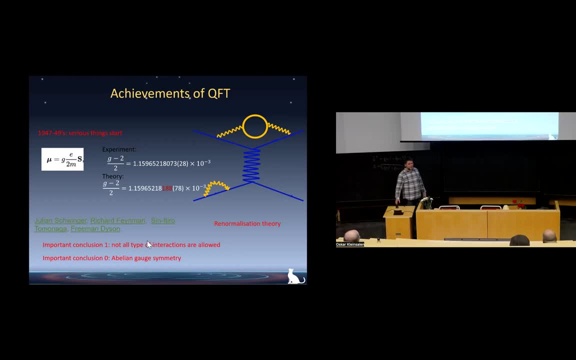 So but mind that not all of type of interaction allowed to get this important result: the normalization of the field. An important conclusion, number zero, that to achieve renormalizability you need to speak about gauge symmetry Again, I will speak about gauge symmetry seriously in two weeks. 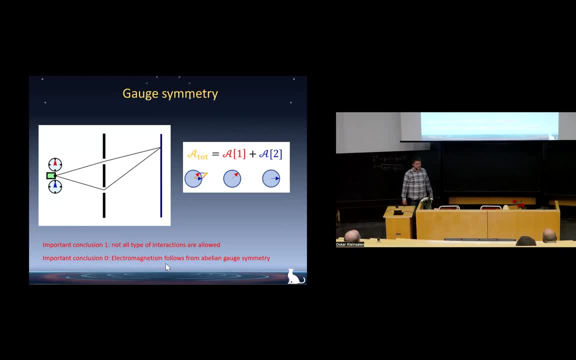 but I will give you just brief idea what it is. When I did this story about two complex number changing. so this is not the clock, it's not time, it's complex number change. I just draw clock because it's visually nice. There is no actually the ground understanding how fast the clock can change. 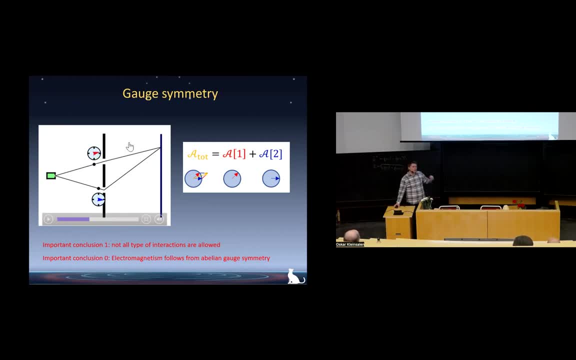 and in reality, there is something in the ground which tell you how fast it can change. There's something is called gauge field, and this gauge field is actually happens to be electromagnetic field. So electromagnetic field is about how this complex number will change fast. This is completely. 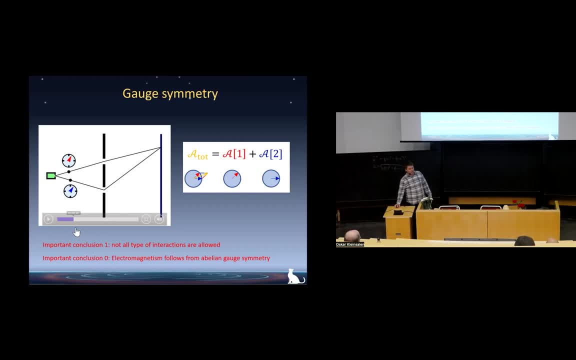 new understanding of electromagnetic field, and I will speak about this much more in two weeks. However, I also want to mention that next week we are going to have lecture about general relativity, about gravity, and there is another gauge, symmetry there, which is different reference places have different geometry and this is kind of the same idea. 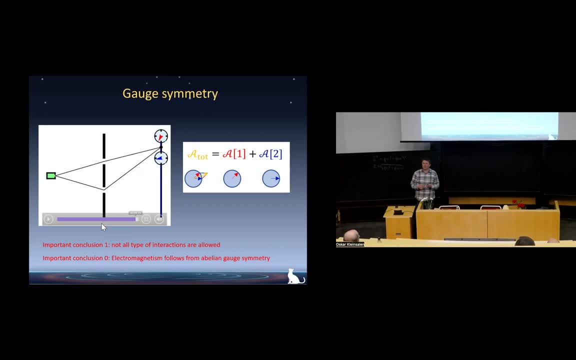 and maybe Sasha will speak about this. I don't know, but it's most likely will happen in some way. So for the moment, just keep this word in your head and wait. then it will become explain more in future events. Right, so this was our lessons from doing quantitative dynamics. 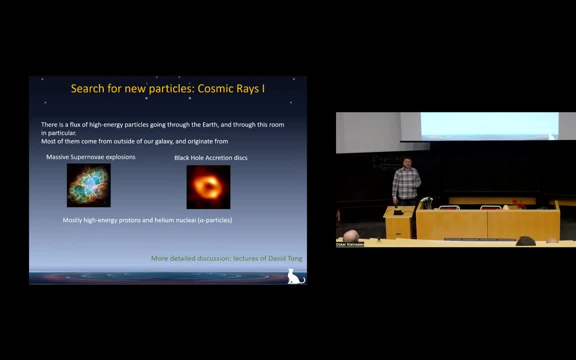 Okay, I finished with mass and now we come back to particle load. So where we stopped, We stopped with the nuclear decay and bombarding these alpha particles as a nucleus to produce even more decays. This is what experiment where I am doing, for instance, to 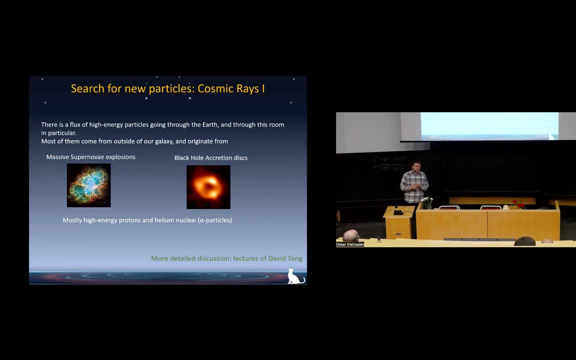 show that the neutron decomposes into proton and electron. But people understood that's super nice, we can get many results. Let's look for new sources of particles that we can collect. What people did next? they, they, they bought balloons and went to the atmosphere, because actually there are a lot. 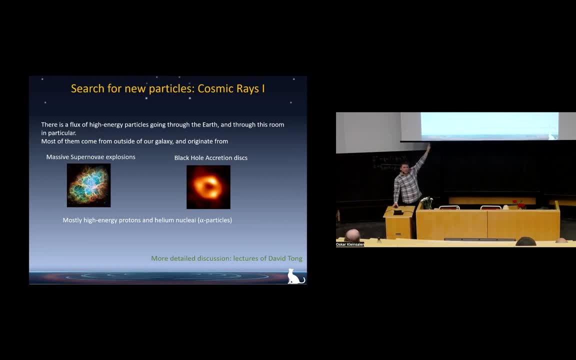 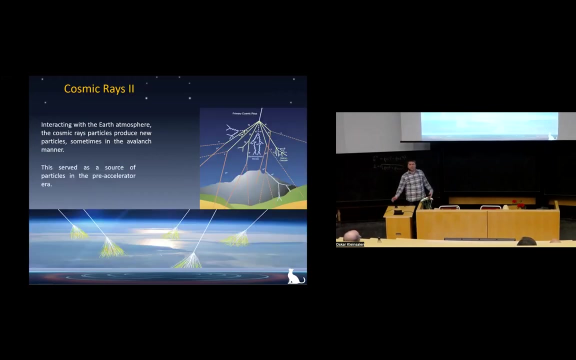 of particles which fly from the space so far away from our solar system. there are black holes and there are explosions of supernovas, of the stars. this is highly energetic events that create highly energetic particles, protons and alpha particles- and they fly through the space. space is reasonably empty. come to earth, come to atmosphere and atmosphere they start to. 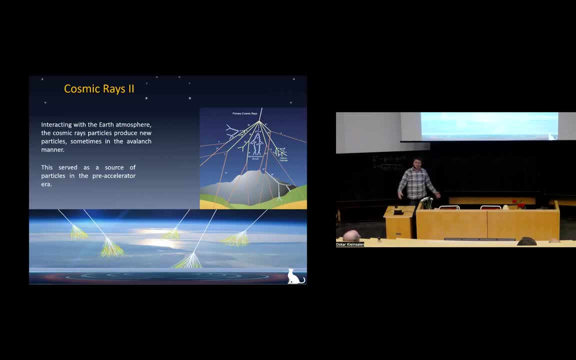 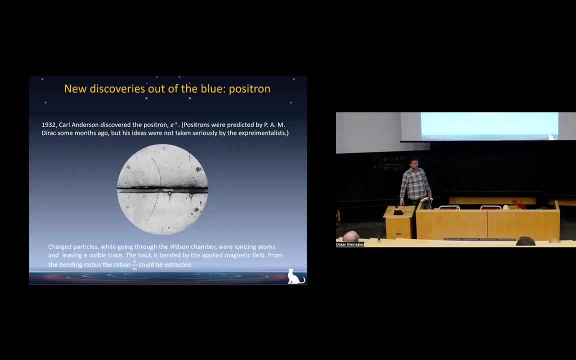 interact with atom atmosphere, producing avalanches of of different events, and the only thing you have to do you have to bring your. i mean this type of things, except they now look differently. they call tweets from chambers and measure the events. so this is exactly photos from wilson chambers. so, for instance, this is: 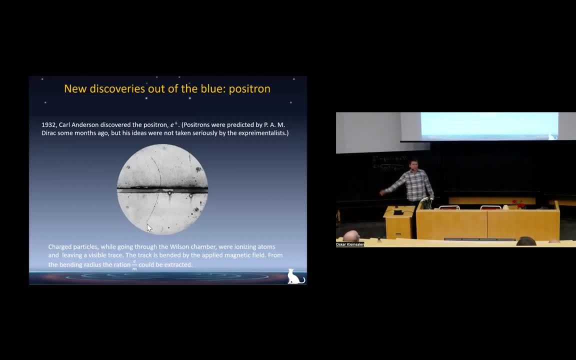 discovery of positron. so particle which flew from the sky passes through some medium which was invested into magnetic field, and this curving correspond to a charge mass ratio. the sample electron electron. but it was curved in opposite direction. so it's kind of the same as electron but has opposite charge. that's how positron was discovered. 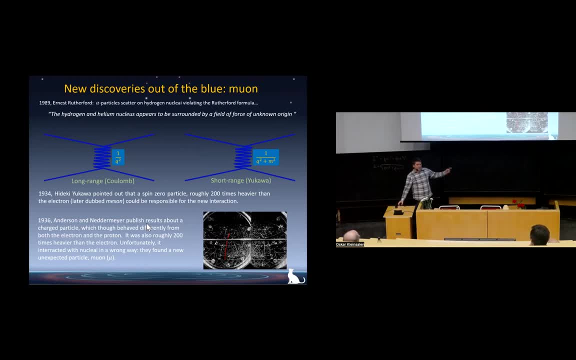 and later. okay, and then people also discovered muons and pines. and why this was? this is, i presume, it's discovery of muon. this is for you remember correctly. so why it was important. well, remember from diagrams: electron flies in its photon, and here another thing, and so this is when this is amplitude of probability of this photon. 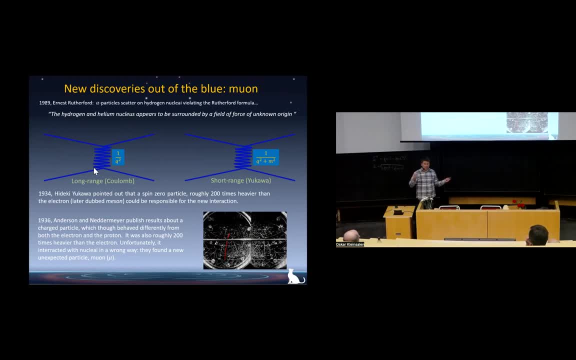 uh, then it gives you long range interaction, which is called bump interaction. then, uh, people understood that something is wrong with alpha particles scattering through hydrogen. when alpha particles come very close to hydrogen atom, uh, electric traction doesn't work to describe the spirit and there should be some new type of interaction which should be short range. 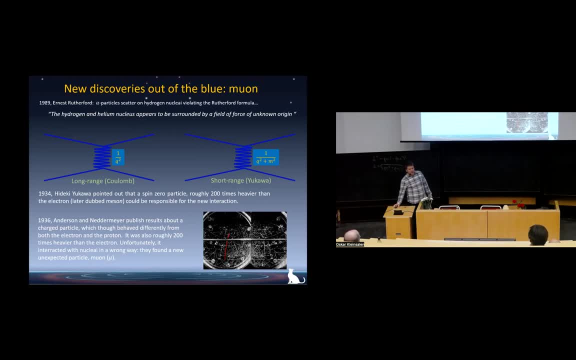 and hideki hideki ukava proposed that now amplitude probability of this guy is not one over q square, but changed, and this guy actually is massive. if it's massive, then actually this corresponds to the fact that the action will be short and well, eventually they found the particle which is called this day's 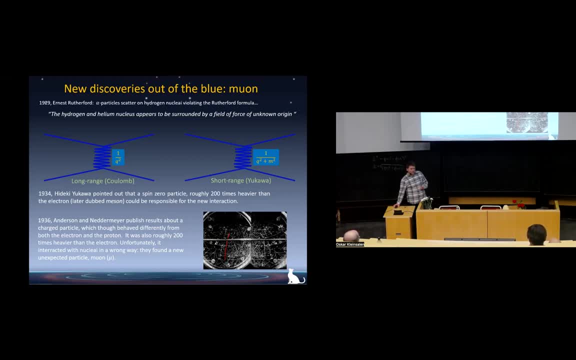 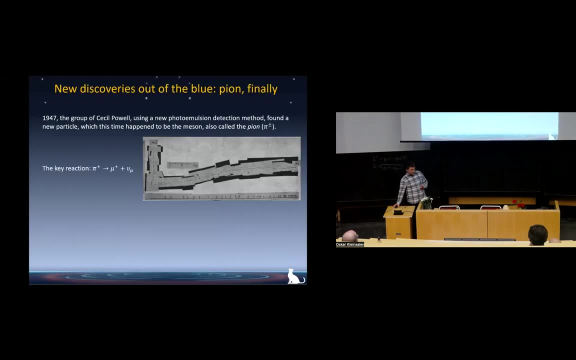 ion which correspond to this interaction. yeah, so this is how they found it. okay, so, but they did not only found muons, pines, positrons, they found thousands and hundreds of particles, and by the by 1950s, people already started to build big machines like almost modern accelerators, and they produce. 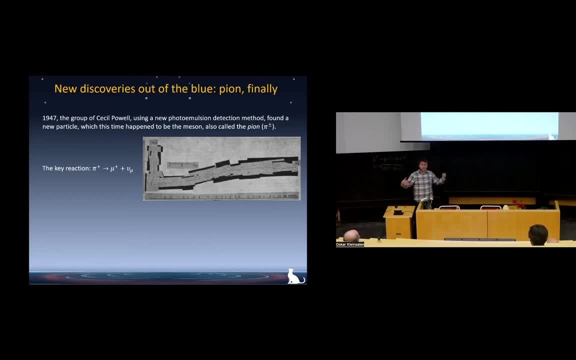 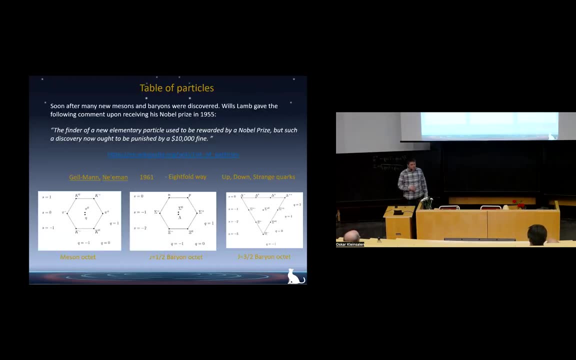 high energy rays in laboratory, and they're describing hundreds of thousands of particles and so so now become a problem. so will. slump received nobel prize, and he said in 1955: if before finding elementary particle used to be rewarded by a noble price, such a discovery now ought to be punished by a fine, if not by a prison. 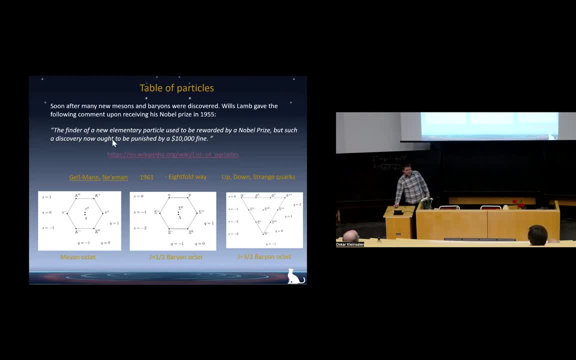 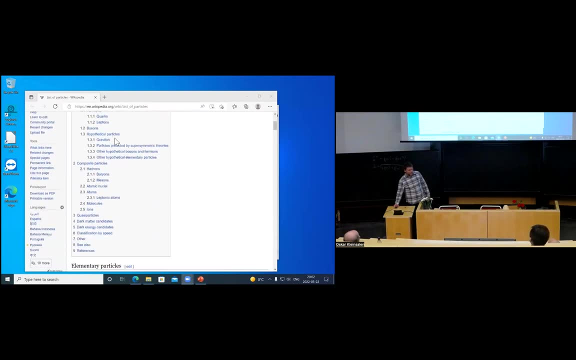 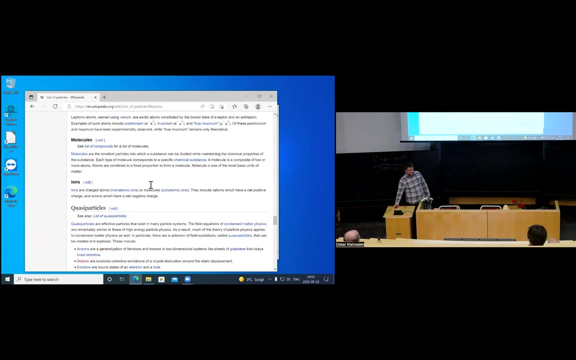 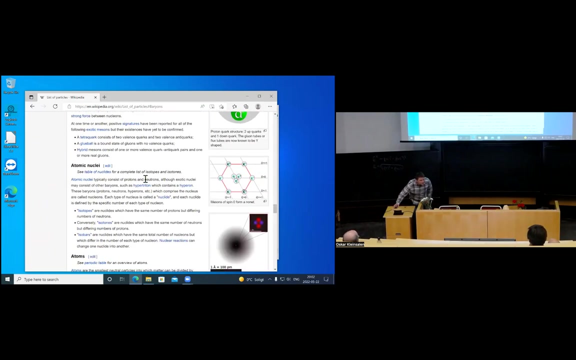 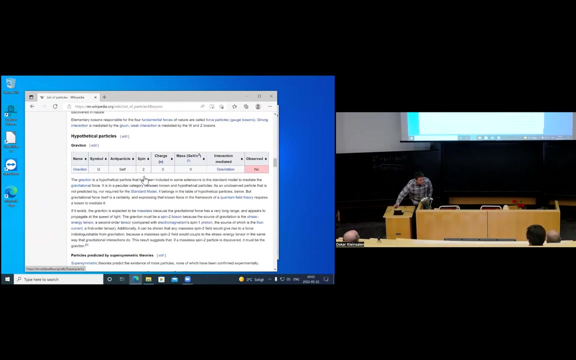 uh, because what we can do, we can go to wikipedia. let's try and just look on the class. so there is a class kept on this. let's go to biomes, is it correct one? uh, oh, yeah, okay, it's kind of here. uh, oh, i did, i miss it. 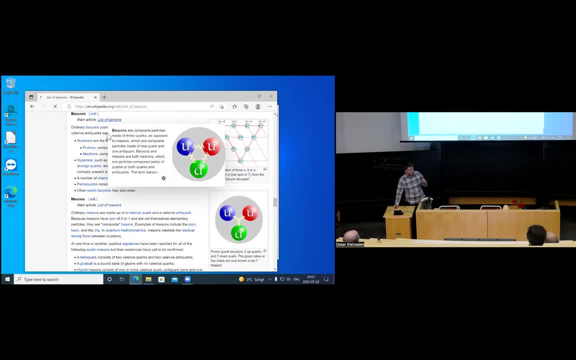 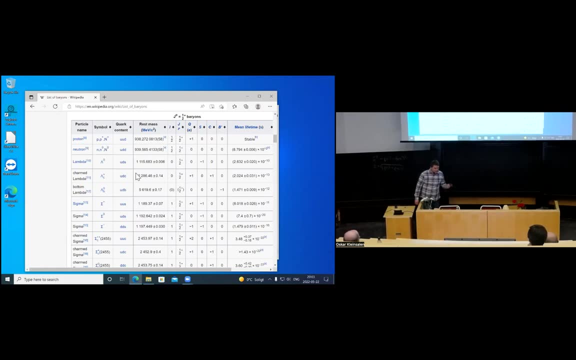 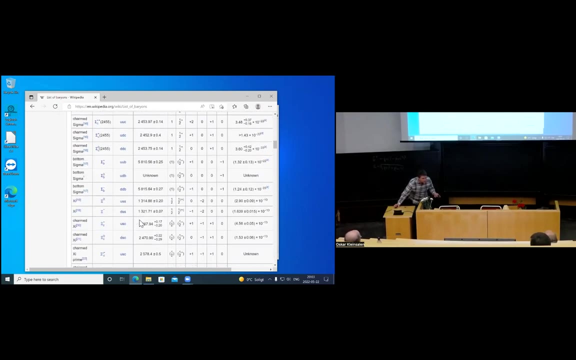 oh, yeah, yeah, this is what i wanted to look. yes, thank you. yes, list of variants. so there is proton, neutron: lambda chunk. lambda bottom lambda sigma. sigma plus is a sigma minus charm sigma. sigma plus zero bottom sigma bottom sigma one bottom sigma key key charm, key charm, charm, charm prime. 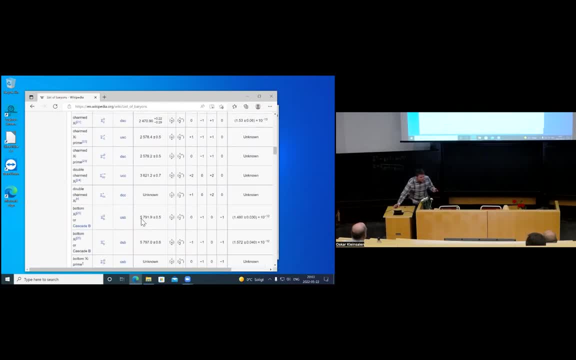 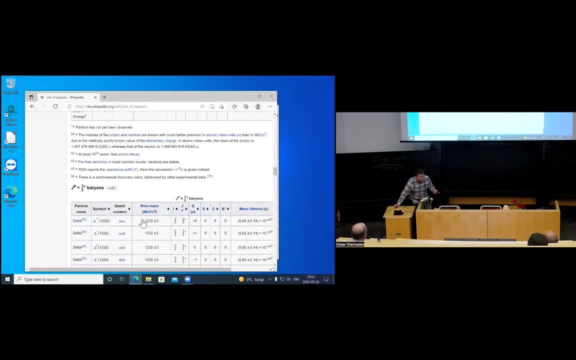 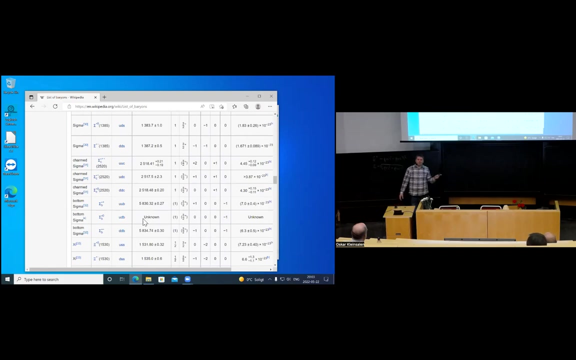 charm, key, prime, double chankey, double chankey, bottom k or cascade b, bottom k or cascade b, and yeah, it's just for spin one half. uh, then we start: delta, delta, zero data plus. okay, so do you get at the point this all the particles which you have discovered? and this is 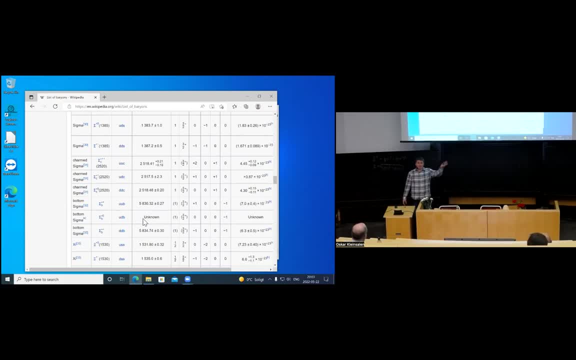 only baryons, because baryons the guys, this, uh sequence. inside they're also mesons, these two quarks, that's also decreased and there is other complicates. so it became a mess and everything was found in the lab, uh, or in the cosmic race, and something has to be done with it. 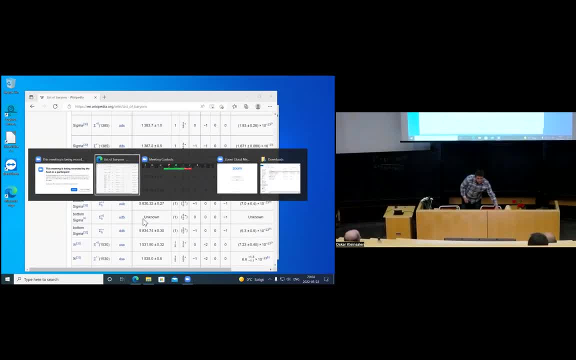 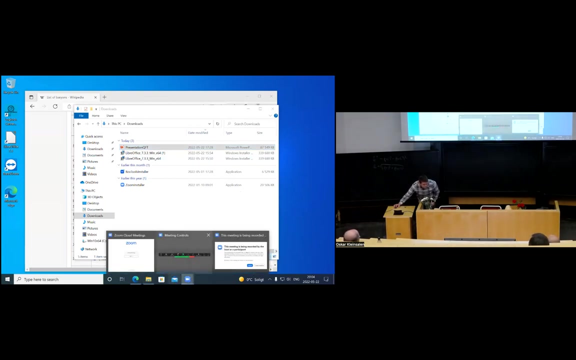 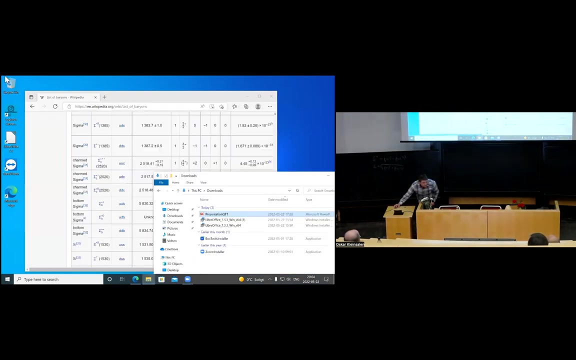 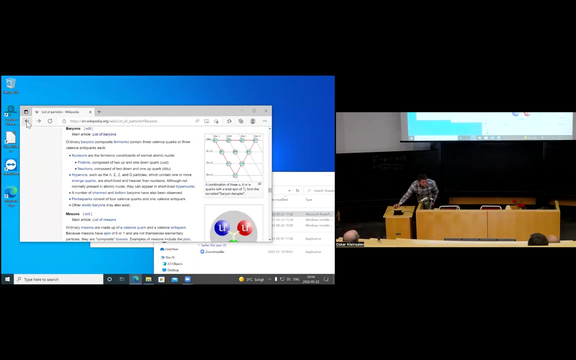 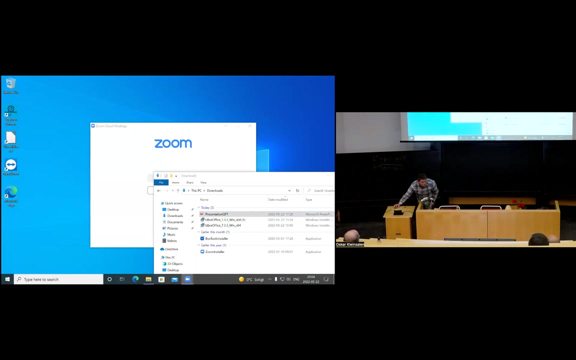 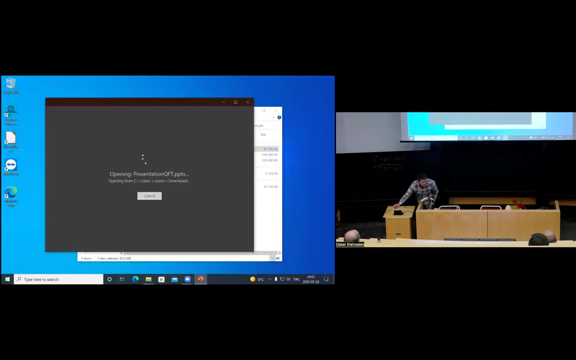 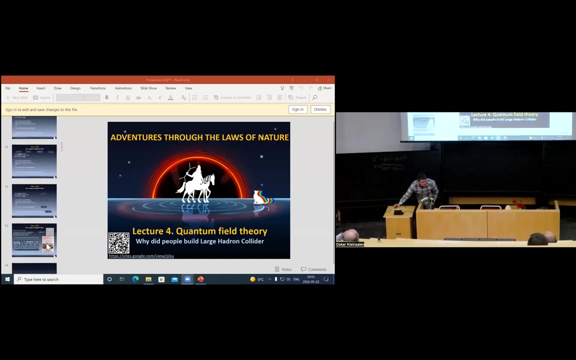 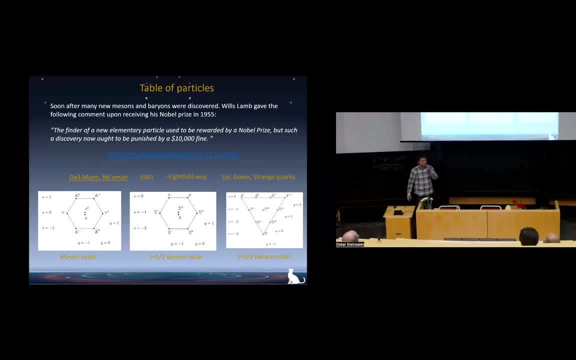 um, all right, so there was a big mess and people try to understand how to organize it. and uh, galman and neiman proposed the eight fold way to organize things. they actually understood that everything can be characterized by incomprehensible, whatever it is. and electric charge. 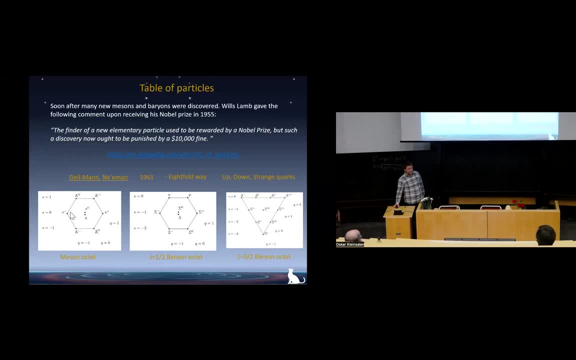 and so mesons, like certain type of mesons, it has this ion which is was discovered for explaining interaction of alpha particles, is proton- it's somewhere here- and also some single counts. they form together. it's six here and to here there is baryons. this is natron and proton actually here. 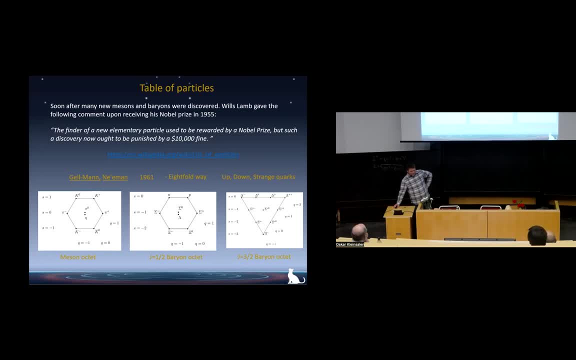 look there here and some other guys and they're like spin three half baryons. so things start to look nicely together and this was explained by existence of. so i mean, if you have all this mess, you probably don't believe this is elementary particles, right? you think they actually still? 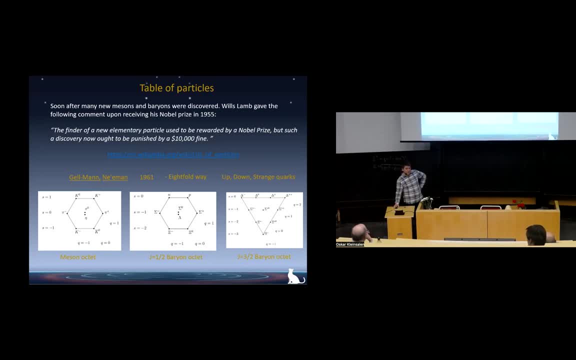 composed of something else, and so this gentleman proposed that there are three elementary things called quarks. there are three of them up, down, and strange. all together they make these nice patterns, and actually they use what is called in in mathematics representation theory of su3 group. for those who know, this is not su3 of qcd, it's a different one. 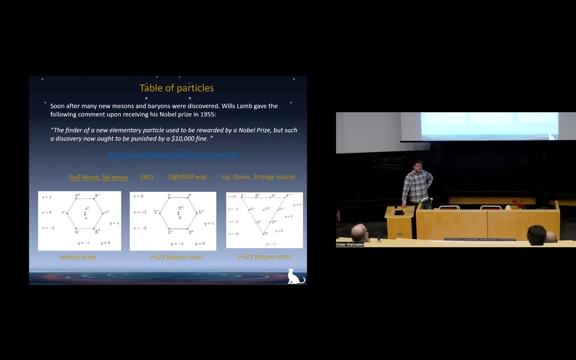 and next week in upsala, eduardo is speaking about symmetry, and probably he will speak a little bit about what this actually means anyway. so they said that these three guys can explain all this mess, and this is how idea of quarks appeared. and again i say: 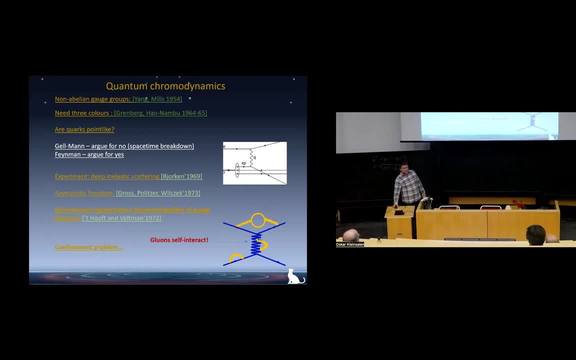 my safe uh for two weeks. in two weeks i will tell more, but briefly. so clouds should be described. so parts were proposed as new elementary particles, which so protons will consist of quarks. but behind this is our history, is history of quantum chromodynamics, so we had quantum. 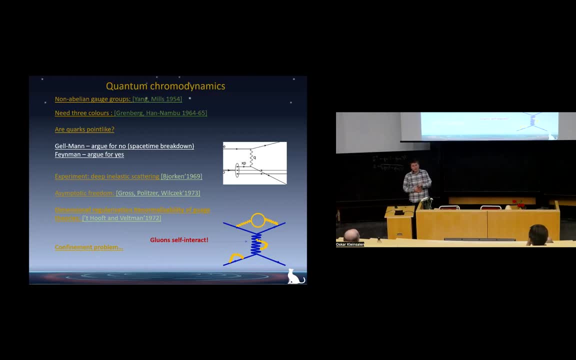 electrodynamics, this quantum theory of electromagnetism. so here we have chromomagnetism. well, chromodynamics, i don't know how to say uh and uh. so some some milestones of this. first, it was purely theoretical idea. uh, remember, this was gauge symmetry. gauge symmetry is about how you parameterize this moving, complex number. 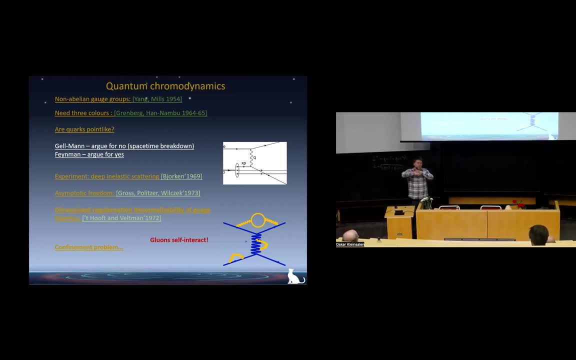 and again it's related to possibility, to uh. now let me tell at least geometry: uh, so this complex number moving around the circle, uh, but what if you replace the circle with another object? you can replace it with two-dimensional, uh, well, three-dimensional sphere and move a number in the sphere. this will be called su2, non-mobilian theory, or you can replace 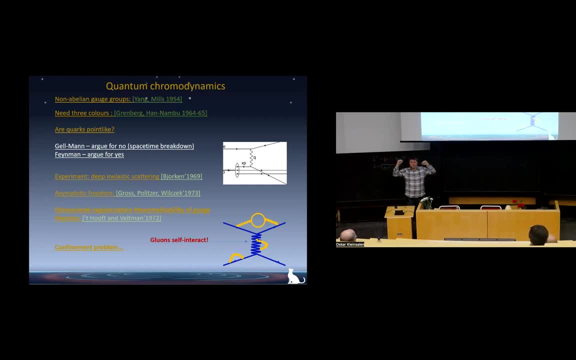 it with even eight-dimensional uh space and you replace the circle with a dimensional thing. it will be a gauge symmetry behind quantum chromodynamics and because it's eight-dimensional, you will have eight analogs of photons which are called gluons. so this first will propose uh. 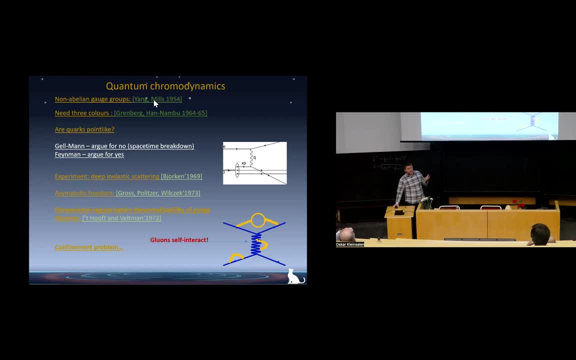 theoretically by young mills, uh, but it was not accepted because it wasn't physically very dense. um. so again, i hope to speak about this more in two weeks. now it's a little bit too unclear. what does this mean? then there was a problem. i told you that. 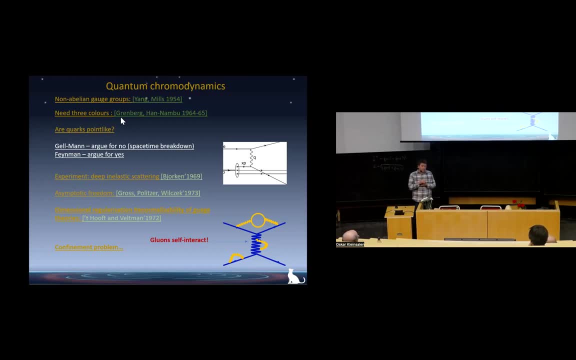 electrons, so fermions do not want to be together. electrons can be spin up, spin down and so, at least because they spin up down, two things can be together. but inside nucleus, inside of protons, there are three quarks, so spin up, spin down is not enough. 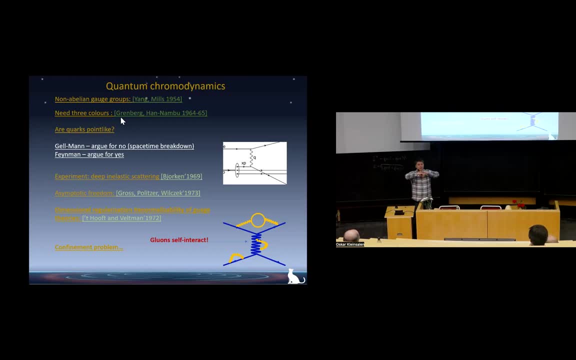 you need three different things to make them together, and that's why people suggested that quarks have three colors. uh, uh. then there was a question: okay, quarks is elementary particles as a point, like like collector, and people did not agree. first, galvan say: no, they're not, they're not. 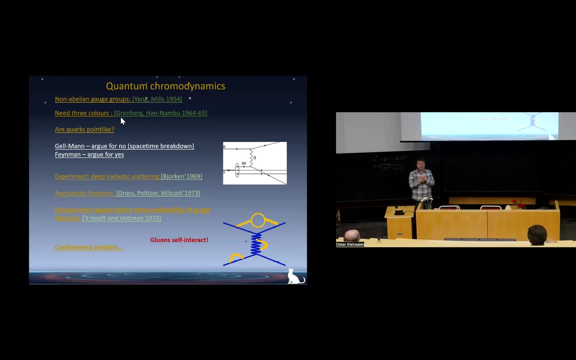 actually, because they're so small. at this small scale, they finally space-time breaks, it's no longer continuous and fermions say no, no, no, they're like electrons. and then it was deep analytics had an experiment- this is a picture of it- uh, which told you that actually, uh, they indeed point like: 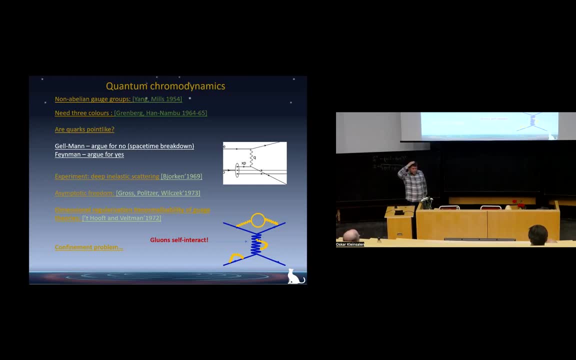 uh. then there was a story about asymptotic freedom- again, i'll speak about this in two weeks- seriously- and the proof of renormalizability, and hoffert might have got another way. a noble price so, and twice was, but uh, what i want to emphasize now is that gluons 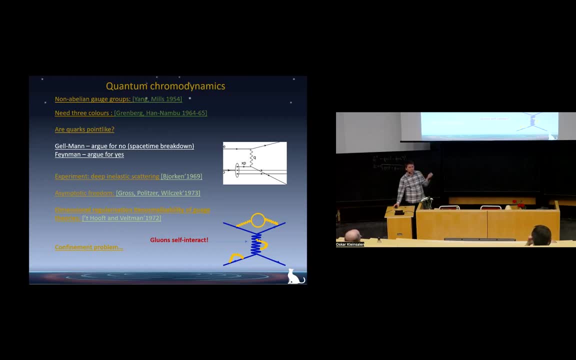 which analogs of photons, uh, do something new. they actually can self-interact. so gluon in frame and diagrams can emit a gluon which come back and this. so if this pair polarize your vacuum, gluon self-polarized vacuum, so it doesn't require any fermions to do. 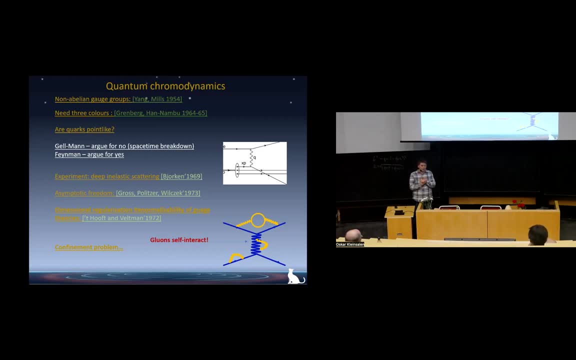 it and because of this you have a problem of confinement. so we say that, uh, natrons and protons consist of quarks. can we smash protons that hard to? to take quarks apart? like well, we were able to analyze atoms, we were able to split nucleus. let's 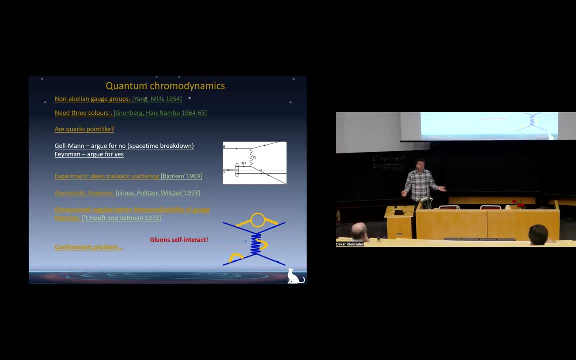 now split natron or proton. well, people tried, tried hard and they could not, and this is related a lot to self-polarization of gluing field. this is for confinement problem. it's still unsolved, normally like not proven rigorously, but there's a lot of numerical simulations and lattice. 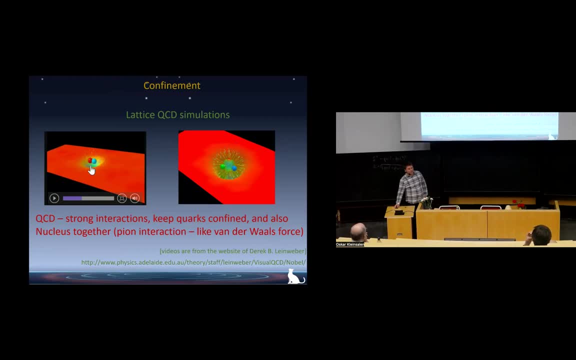 and so this is meson. it's a particle consistent of two quarks, and what happens? um so, uh, if you try to move quarks away, uh, then uh, gluon will self-polarize the vacuum and create what is called flux tube, uh, between two quarks, and it will increase in energy. so, pulling quarks apart, uh, will increase increase. 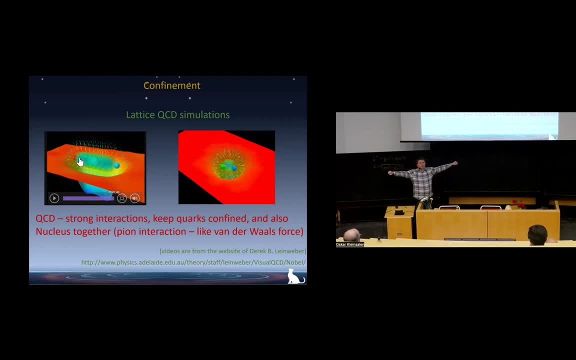 energy, and if you really try to put them too far apart, that will be so, so high that in between here, two new quarks will increase energy. and then you'll be so so high that in between here, two new quarks will emerge, and the only thing which will happen that your method will split into two new methods. 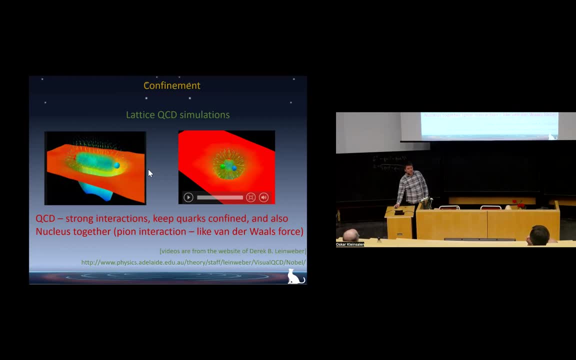 but parts will not be separated. and when you have three quarks, which is like natron or proton, there's eight. the same stuff happening: this flux tube polarizes vacuum and becomes like this. so, uh, we say these days that protons consist of of quarks. however, they cannot split proton. 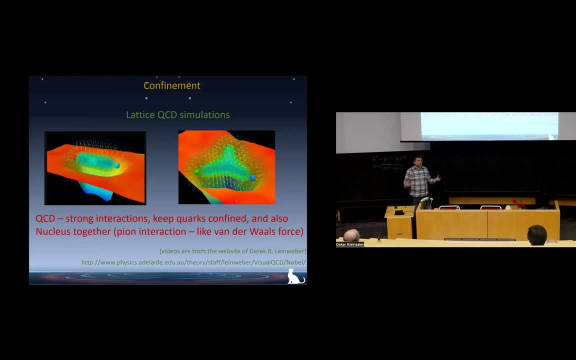 on, it still stays together, and this is a difference compared to our previous, because what is we're trying to do all the day? to split things together into smaller, smaller pieces. we reach the point, we know what is inside, but we cannot take it out, and quarks are considered as elementary particles. 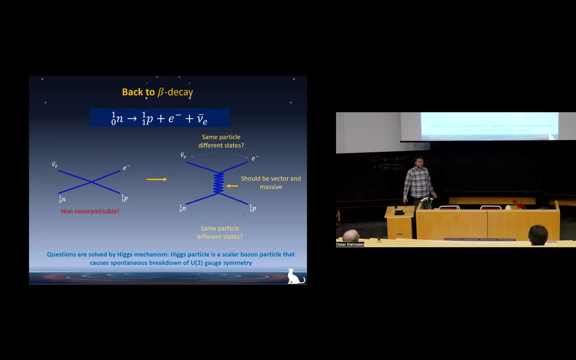 and finally. uh, so i told you a little bit about quarks and finally we come back to our story before the break. so we started from the story that natron transform into proton and electron. you see, that don't work. the word decay into proton electron, i will use the word transform. 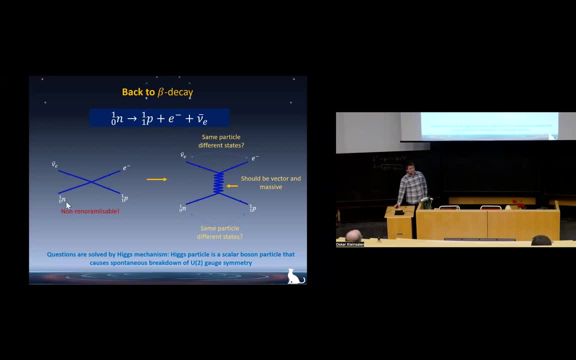 and also antineutrino from the. so if you seriously believe in this, in this diagram, in this process, you have to draw the full uh frame on diagram natron fly. So here will be destruction, operator of neutron and creation of operator for three other guys. 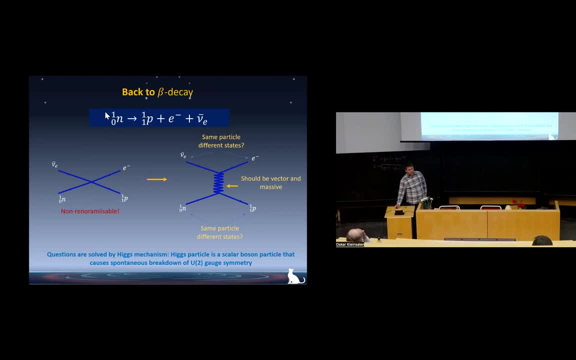 It is called four fermionic interaction, because all four guys here are fermions spin one half particles actually, And this secret word renormalizability. So this interaction is non-renormalized If you look in all our previous Riemann diagrams. 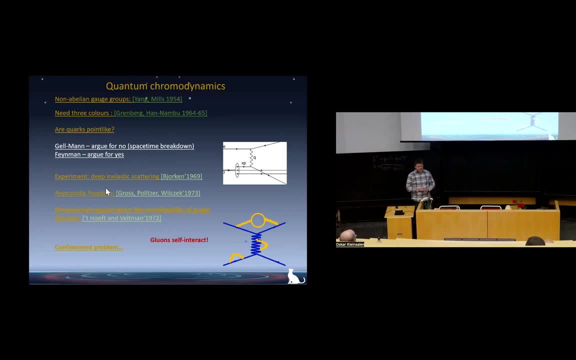 they were always the same type. It was: fermion flies emits boson as a photonogluon and another fermion receives it. It's also this type. It could be decorated all corrections in yellow, but it's just dressing for things. 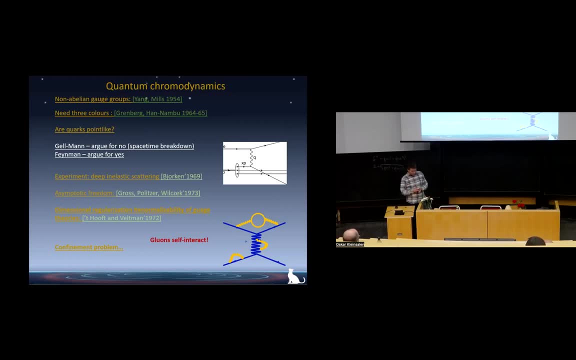 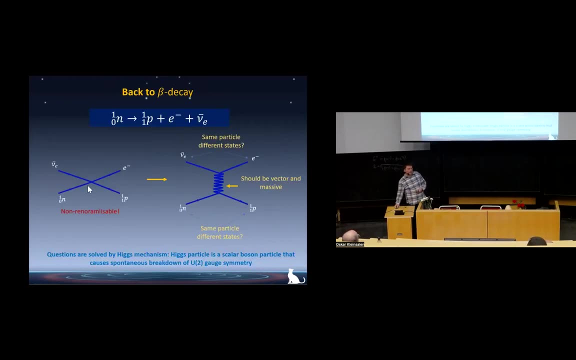 If the process is of this type, then theory end up being renormalized when things arise, So then it will be natural to expect that in reality this is not what is happening, That actually neutron flies, destroys, emits something and also proton is created. 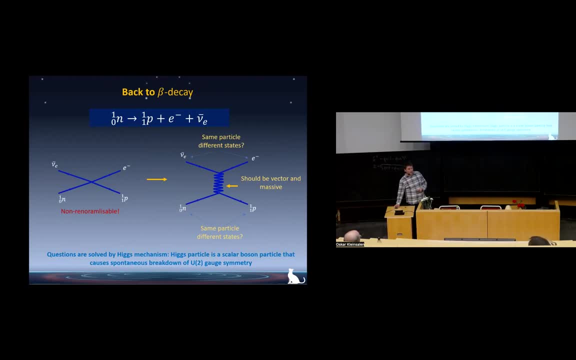 The something goes and interacts with antineutrino and electron, or let's say decomposes into. I mean in this case it decomposes into neutron and electron, antineutron and electron. So we would like to find this interaction field to make it. 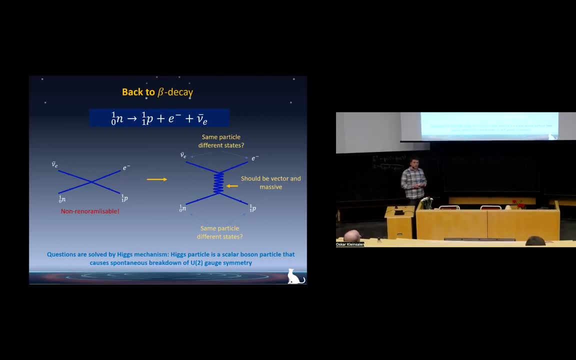 similar, and then we hope that it will be renormalizable and make sense in theory. But then the problem comes that experience shows that this interaction is short range and this vector here could be. So first of all, they should be vector field and that should be massive. 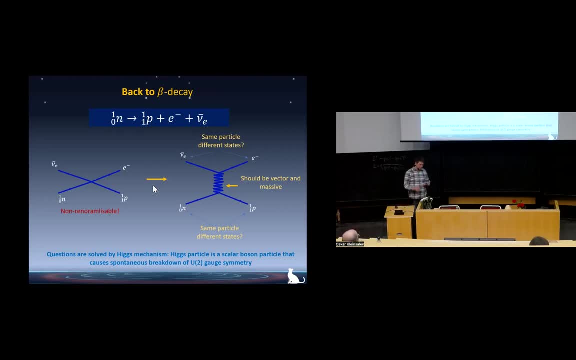 And if it's massive and just random vector field, which is massive, you can have a problem with this. You can have the problem with this, But that's not a University theory: renormalizability. this is problem number one and problem number two, uh, that it's kind of. 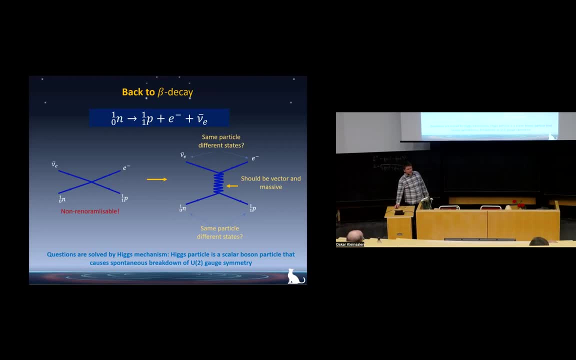 kind of suggests that this happens, suggests that natrium and proton actually, uh, somehow relate, and so also for an integral electron, is it like the same particle but different states? so this is a question. uh, this is. it is a little bit philosophical, but this is important. 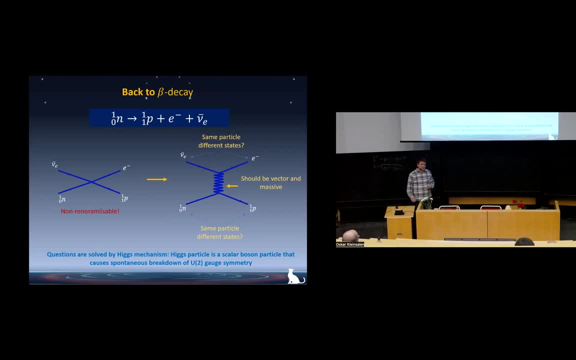 if you have vector particle which is massive, you again have problem with renormalizability. and to solve this problem people suggested higgs mechanism. so finally i came to higgs mechanism. higgs particle is actually was proposed as a scalar boson which, for the moment, i just say. 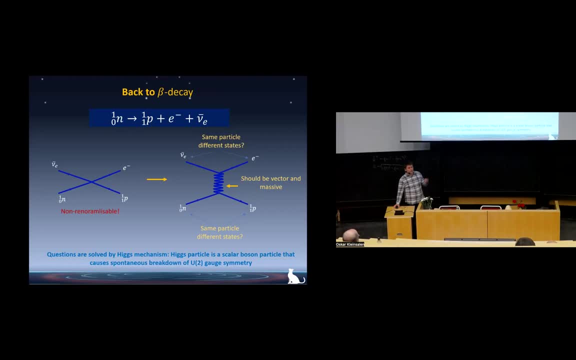 spontaneous breakdown of two gauge symmetry and in two weeks i spent half of the time explaining what does this mean? so higgs boson was proposed to resolve this problem. this was bad. something should exist here, but something should be massive. But if it's massive. 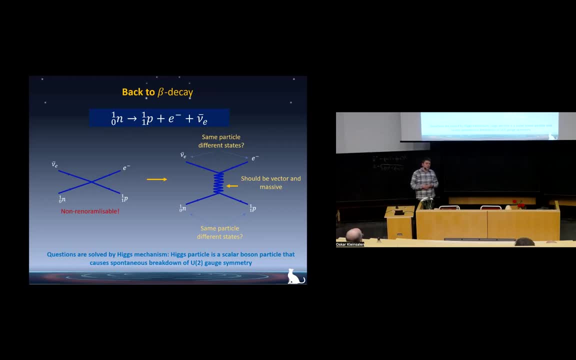 theory of mathematics is still inconsistent And there should be a mechanism to make it massive, and Higgs boson was proposed for this mechanism And it was, to my knowledge, the only reasonable proposal. I'm sure there were other ones, but others didn't survive for one another reason. 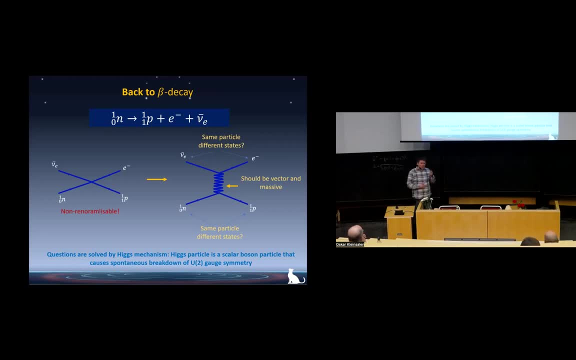 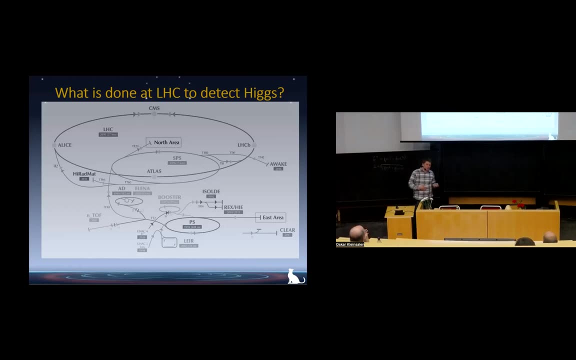 and people were looking for Higgs bosons seriously, And so, finally, one of the reasons to build large Carnot-Lupin-Reil collider was to detect Higgs bosons, because if we found it, then everything we said about particle physics started to make sense. 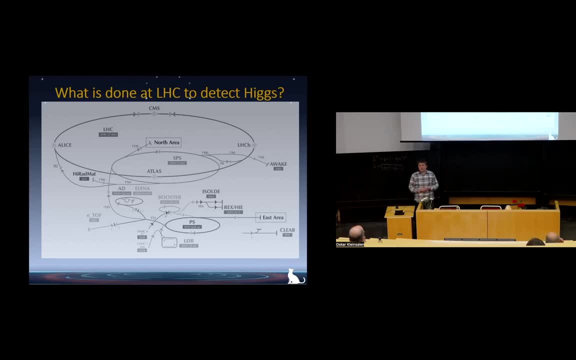 And okay, they built it, but what are they doing with the experiment? Okay, so actually it's not just one circle, it's quite a bit of things around. First of all, there is this part here: creation of a beam. So there is one accelerator which created to first energy level. there is a 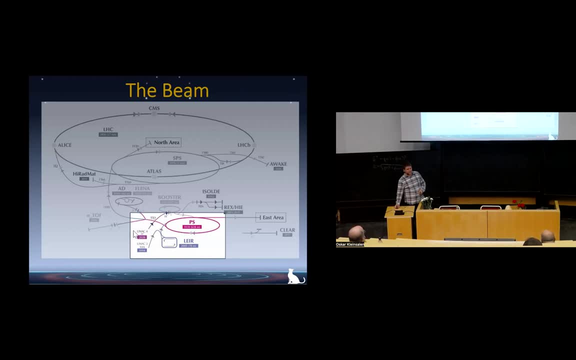 smaller cyclic one, accelerate again. after that it brings it here, accelerate one more time and after that it goes to the big circle. So it's actually in several different iterations actually it reaches the big machine. So what are actually people accelerating? You want to go in circles because you want to accelerate for quite a while. If it will be a linear accelerator, then it will be too super long to achieve necessary energies. So that's why people do it in circles, so it can go many times until it's accelerated. 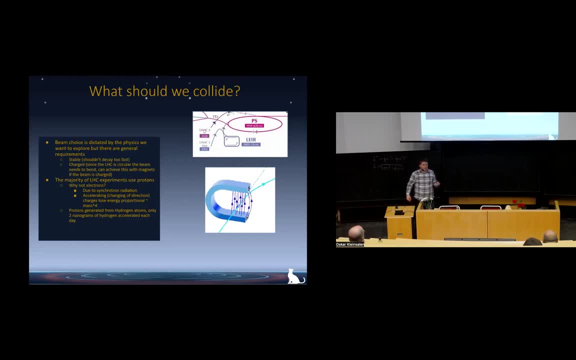 So you want the particle inside this table. it should be charged because the only way to make it in circle is to put it into a magnetic field. But remember this device here put magnet to bend it. So they actually also put a magnet to bend particles here. 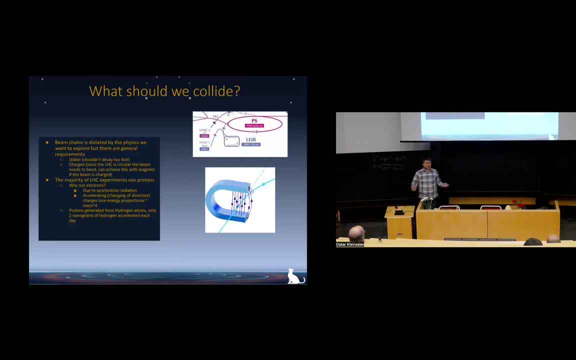 Right. and then there's also the problem with synchrotron radiation. every time you expand it it shouldn't lose too much energy, so it should be charged stable and do not lose much energy by synchronization, which makes, say, we are going to use proton, so they are going to accelerate proton. 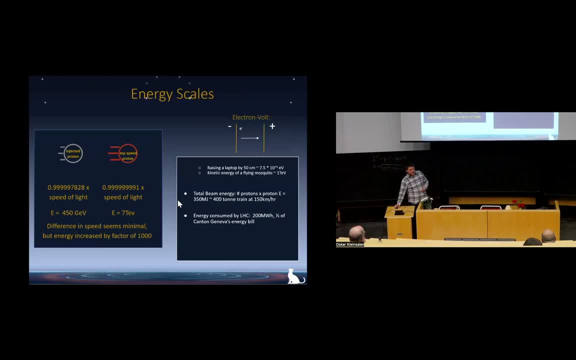 so they accelerated to very high speeds, and let us just recall to which, to which energies they have been accelerated. this is definition of electron. volt is energy of electron which passes potential one volt. so uh uh, injected proton to the big circle is 450 ego electron volt. 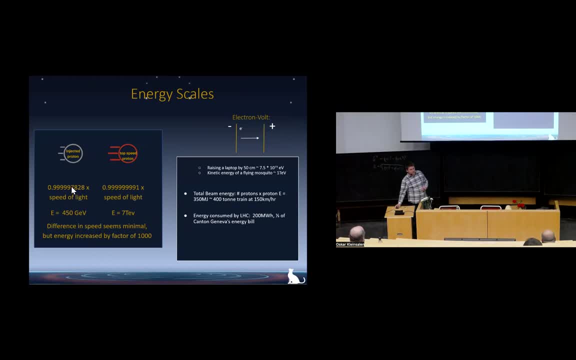 it's already a lot, and this is its speed, so it's almost bit of light. so first five digits is nines and then becomes not nice, but it's still not enough to get higgs. they still accelerate it to that many nights of speed of light. 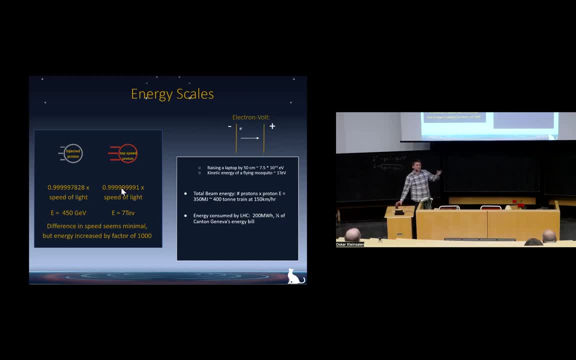 so it looks like almost nothing, but because of florence contraction, this is a huge difference in energy. so this is uh total energy cell. i think it's uh. when two particles collide, this is uh uh. you know, it's not one proton, but two of them collide. as far, remember, it's seven till it, till the electron volt, so it's one thousand. 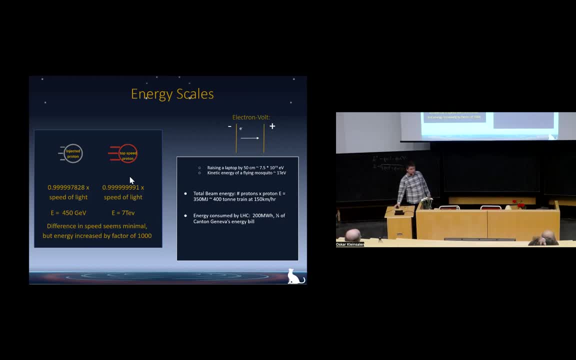 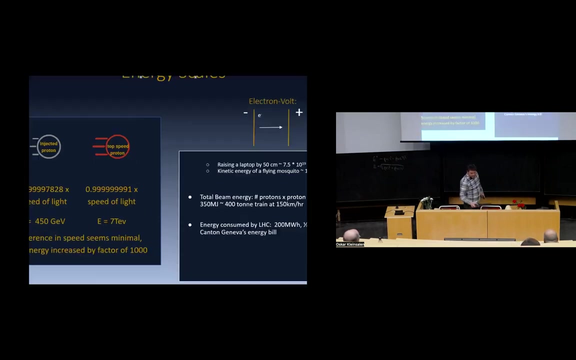 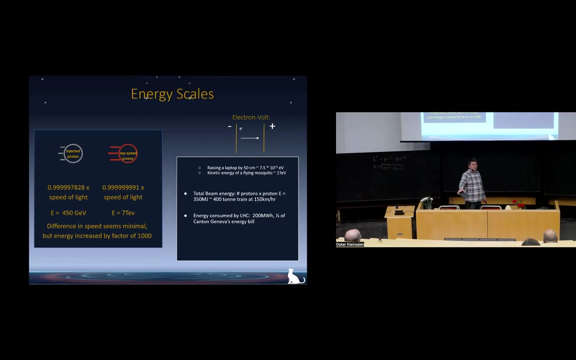 times higher energy. uh, that is achieved. it needed for this acceleration, so is it? is it a lot so, uh, if, if i just take this keyboard and try that here, i will spend much, much, much more energy than energy consisted in one proton moving at this almost bit of light speed. 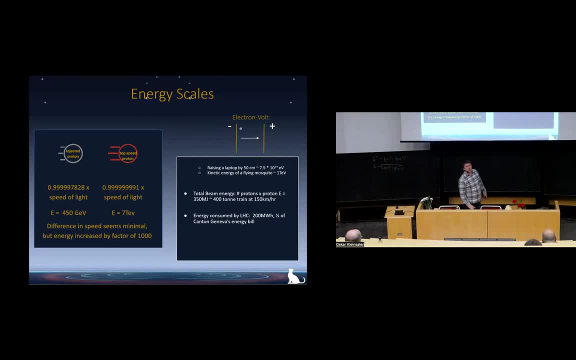 actually, one battery can change, charge millions of protons, in theory, up to these energies. the trick that you want to channel all this energy to one given particle, whereas statistical physics says that you cannot uh, force, uh to be all energy to one place. it always will be distributed because 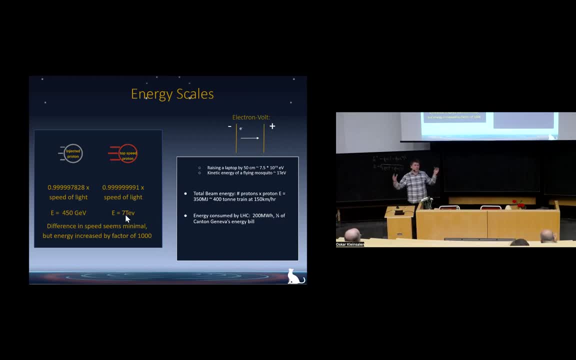 of chaos and in reality you will have a lot of protons, because also you want to have luminosity in your accelerator. you have many products and now it's come more serious. uh, actually, if you multiply number of protons each proton has, for particle is a huge energy. 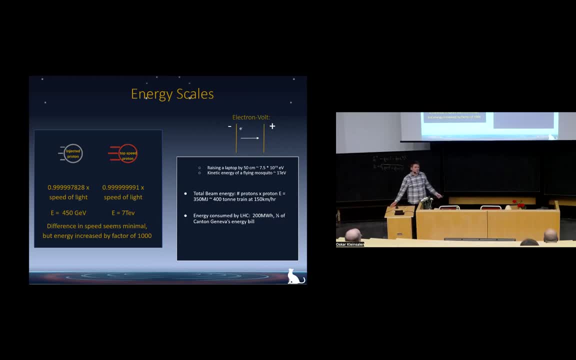 but it's less than energy of mosquito. mosquito is millions of 20 particles or even more uh. so if you multiply number of protons- but actually uh proton energy- by number of protons, so the total energy here is okay. this is what is suggested for 100 ton train at 150 kilometer per. 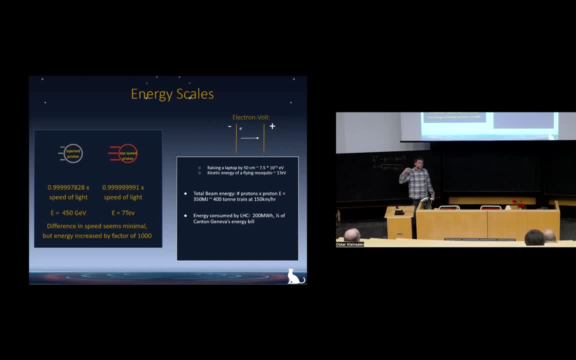 hour. so this, all this energy of it train is concentrated in the proton beam of accelerator and when this happens, that what i told you, when, when actually lhc is running, it's one third, not of geneva, but of geneva canton, which is like a region, not on only the city. okay, so this is how energetically think. 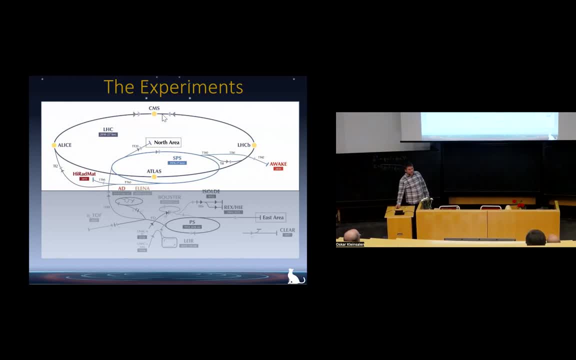 so it's runs here. they're actually several detectives, at least cms, lhcb and atlas, and i don't remember, uh, if i were experimentally speaking, but i don't remember, uh, if i were experimentally i would know it for sure, but uh, it's, i know that not only one detector, but several different. 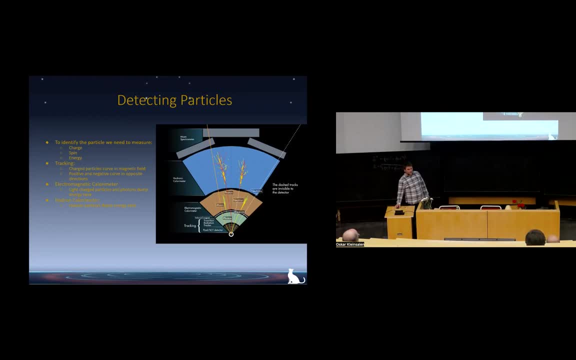 boson, but here is a picture for cms. so here collision happens. so two proton beams collide. when they collide at very high energies, they create a lot of particles and and there are many detectors, this whole type of uh, this photo multipliers, and these chambers and whatever they also use. so this is modern version of everything i told you. 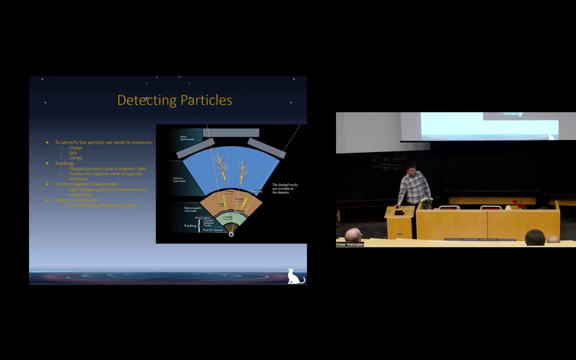 showed it before, on like in historical scale. so they will register photons, electrons. i mean most of the things will be photons, electrons, neurons, neutrons, all. so this will be like 99 percent should go out. but they want very special events, so very many events happening. this is this picture. this is what i what called before. 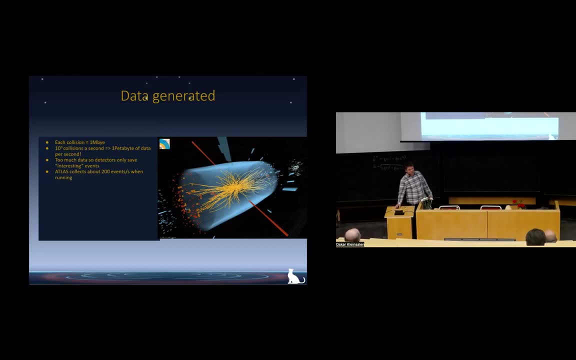 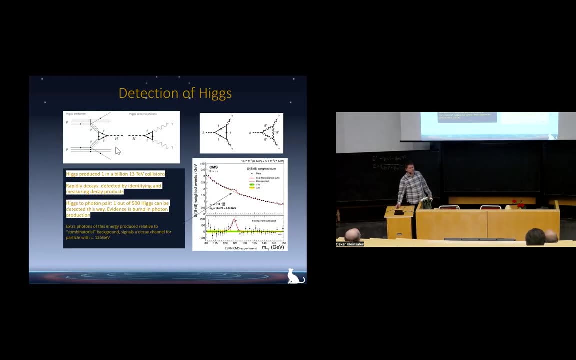 actually you need to find it about a letter coming, you just need to filter it out. and this is actually the process in which higgs boson participate. so you have proton, which consists of three quarks. one quark emits gluen. uh, the exchange has supposed to quark. 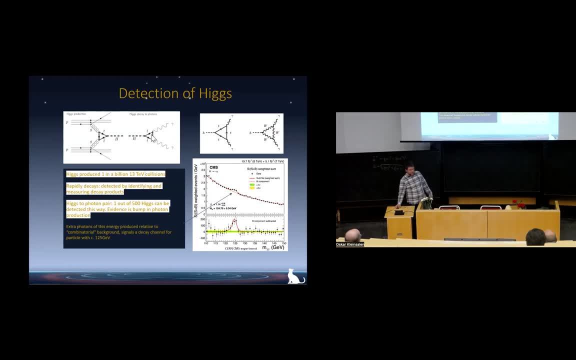 uh, produces higgs boson and then it is decreasing into photons. it's, there are two channels of decay, also through w boson, which this massive particles, uh, uh, explaining decay of natron, and so these two things, uh, it's a main channel, decay of higgs. and so this is, uh, what you see. and this bump, discovery of this bump. 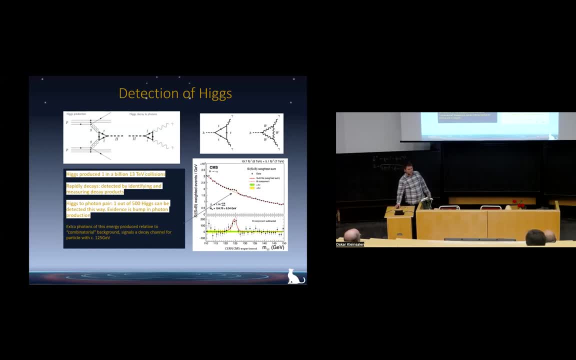 was discovery of higgs boson. when you subtract this curve you get much more clear bump. okay, so here it's 125 peak, and this is peak of higgs boson. so what it's actually, the synergy is südner ke Trent on the it, just gamma radiation, just before it says the combined energy 125. 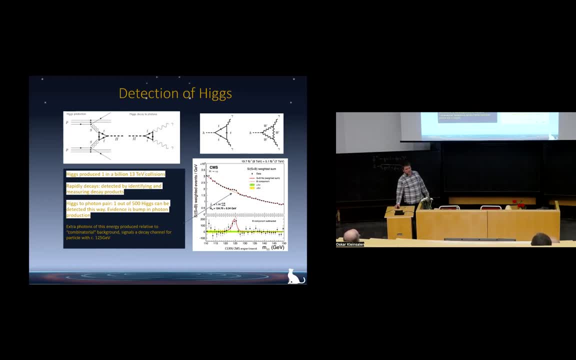 jv and this means that have an obtained from the destruction of one's boson. so hix produce one in a billion 13 electron volt collision. so i said it's seven is both. no, it's only one direction. this other issue together is certain okay. 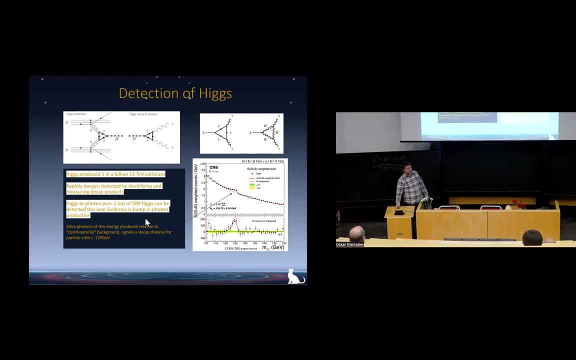 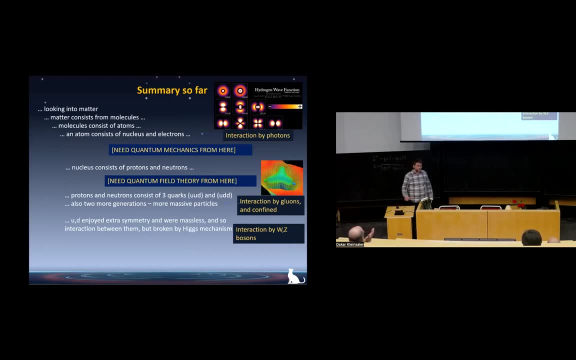 so he's produced. one in a billion and one in 500 can be detected. but well, people get it, and so they confirm a standard model, uh, so let's make a summary. so until electrons was nice, uh, but when we split electrons and nucleus, we need quantum mechanics to explain, uh, how atoms are made. then what we learned now that nucleus consists of. 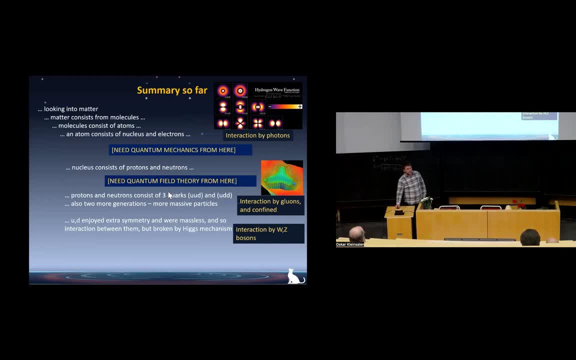 proton and neutrons- uh, to describe this, we already need quantum field theory. uh, and proton- neutrons consists of three quarks, and to do this we need to introduce a new type of quantum field theory, which is called quantum chromodynamics. uh, so we need to give an example of quantum field theory. so proton and neutrons are made up of. 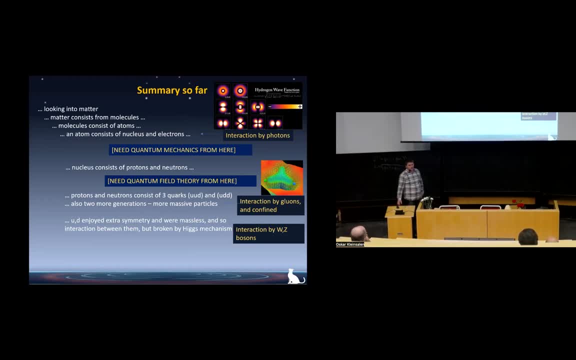 three quarks uh matter on this in this theory. and gluons, there are eight of them uh replacing photons. so they have issue of confinement. so proton consists of three quarks, but it cannot take them apart and, moreover, we have many particles that require other quarks. so early, early experiments. 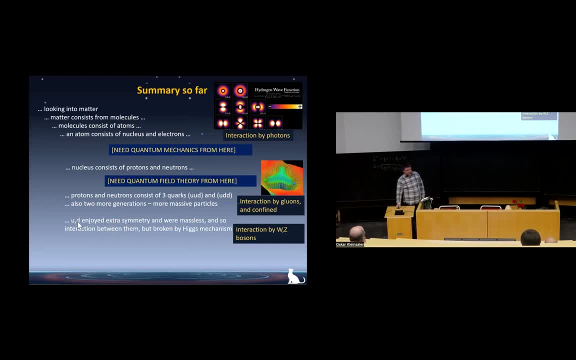 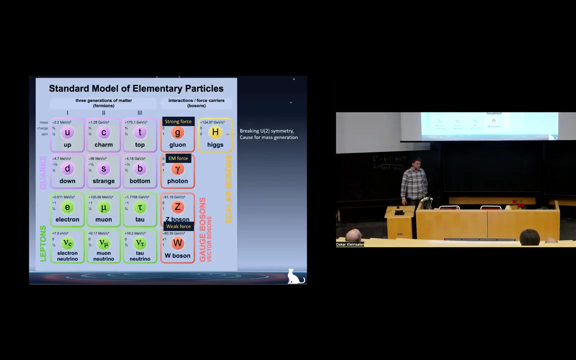 had this strange quark and, uh, there was another problem that, uh, this problem of decay of neutron should have been explained, and to explain it, people have to introduce uh hicks mechanism to explain everything together. and so, combined together, we have standard model, so, uh, so now, 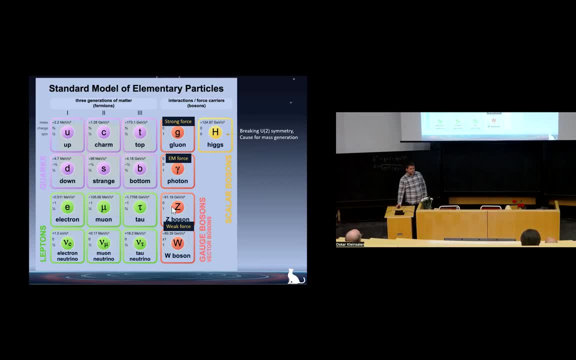 this is how we understand nature, like on the elementary scales. we have fermions, uh, so we have a heavy part of fermions which are clarks. we have three generations up and down, uh, making normal matter. but there is also this charm and strange top and bottom there is much more heavier, you see. 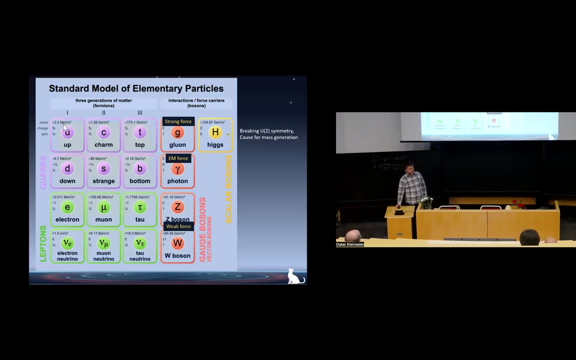 this is their masses, uh, so it's like thousand times more, hundred times more on top uh, and they're also light, uh, fermions, massive uh, electron and the other generation partners. and there is also these guys, uh, well in in canonical standard models. they're massless. 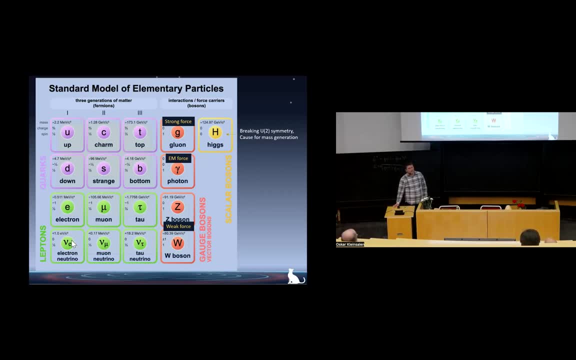 but people discovered, uh, neutrino oscillations, and now we know they are not. and this actually seems to say that this, this what we hear already, is incomplete and it should be updated. so but so, but like, at least you know their muscles. very good approximation, uh, and this is what constitutes 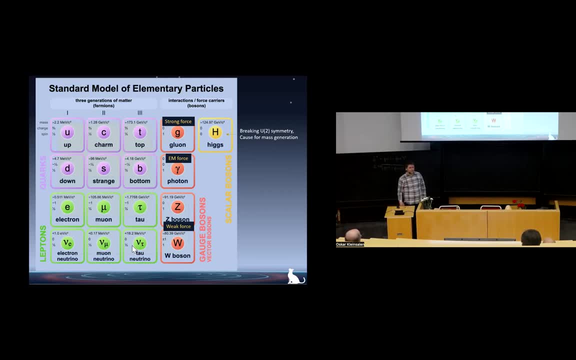 matter of, of everything what we see, uh, and this matter interacts through bosons, and so the most known to us is photon. it's electromagnetic radiation. there are eight gluons. which strong force? strong force, it's interaction between quarks that keeps them together, but also it actually keeps neutron. 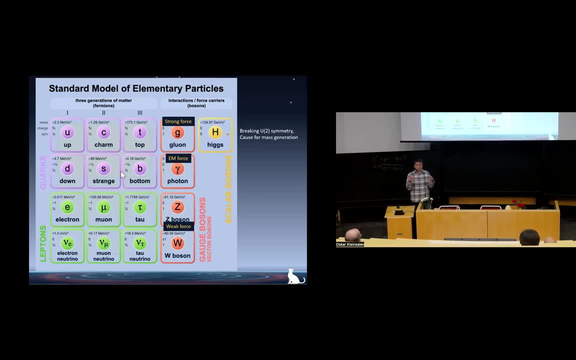 proton together in the nucleus. we actually never discuss this part, why they do not fall apart. actually, interaction of the proton is like underwise interaction on the level of elementary particles, using, again, eventually, gluons. so effectively gluons combine together to form this. well, uh well, okay, uh well, this is probably okay then. um, and finally we have 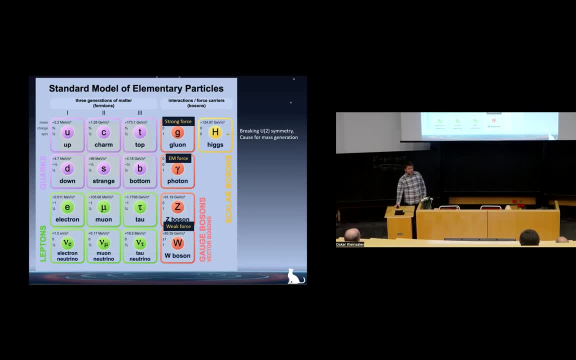 weak force which explained decay of neutron, and originally there were three guys, uh, but higgs broke the symmetry and there were two guys which called w boson and one guy who is called z boson. they have different masses now. originally there was three to the same, three of the same mass, equal to zero, but higgs- 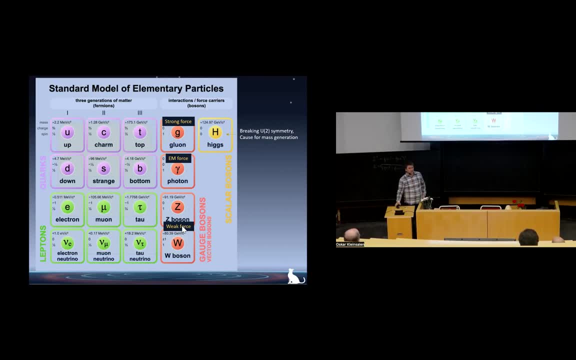 mechanism makes a massive and short interact, short, short-lived interaction. and to explore, to make all the synchronization and explain many symmetries present we need with higgs and it was discovered. so this looks happy end, but there are loose ends and where there are loose ends new physics starts. 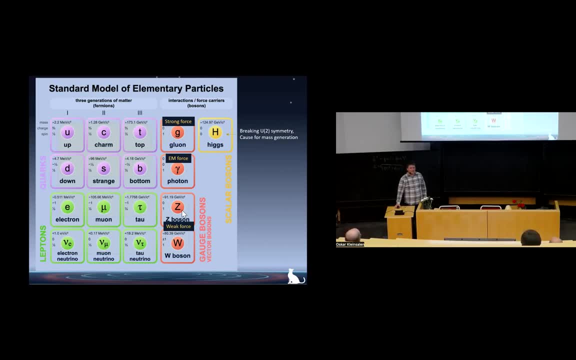 and in two weeks. so one loose ends and some gravity, which we discussed next week, and another looks and- and it's also in gravity, but for in different sense, if you so- loose hands is going to be discussed in two weeks. uh, what's beyond this and uh, what people are looking for these days? 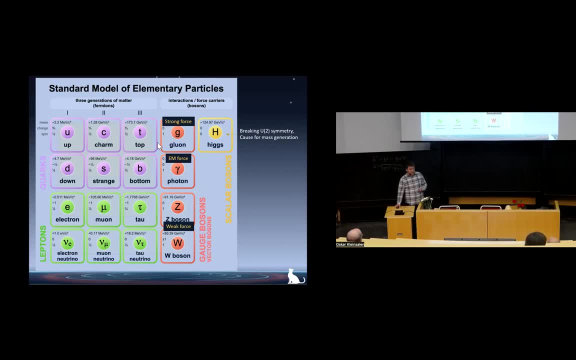 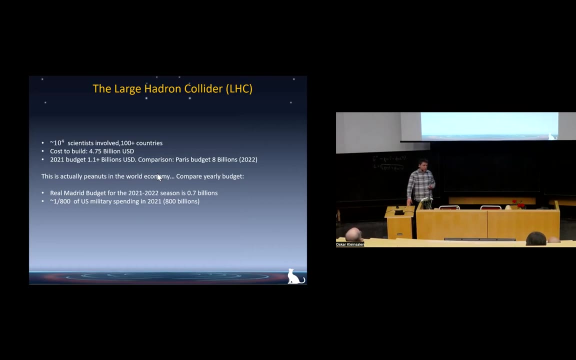 so this explains why people did build lhc to like. well, there are many other reasons, not only this, but this is the one which is easy to well like, easier than other to explain. uh, and now i want to come to the question of budget. uh, because we say that one billion? 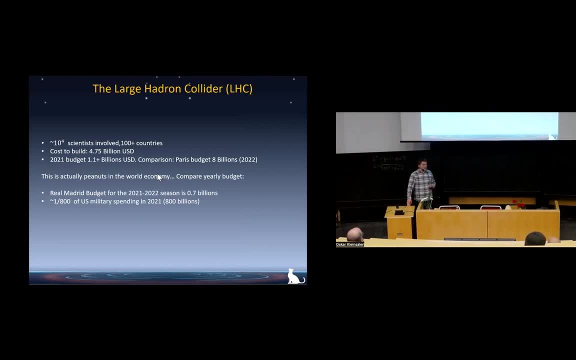 career is a lot, but in reality, is compatible with the budget of real madrid, madrid football club, uh, so let's, let's make it again so: scientific experiment, because plant, uh, the nature of the most fundamental scales, is worth for humanity as much as one football club per year, uh, and, moreover, humanity spends almost thousand times more for defending. against each other, whereas science offers much better ways. I mean what does define against each other? It's fight for resources, eventually, or who will be in control. Science offer much better ways to use resources. It gives us orders of magnitude better ways to use what we have, Yet we spent most of the money to defend against another. 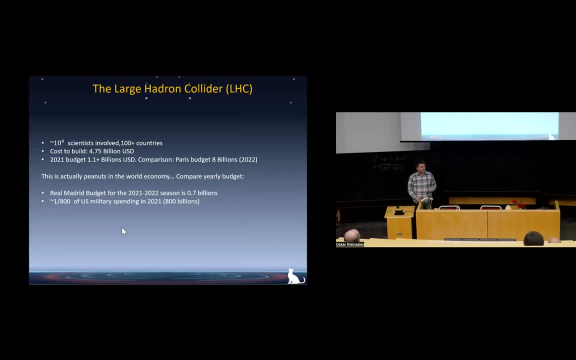 instead of investing to improve everybody's wealth. basically And well, if you look at these numbers, I found once I was modern. well, you may think for yourself. This accomplishes my lecture and I would like to thank for everybody who helped me today. 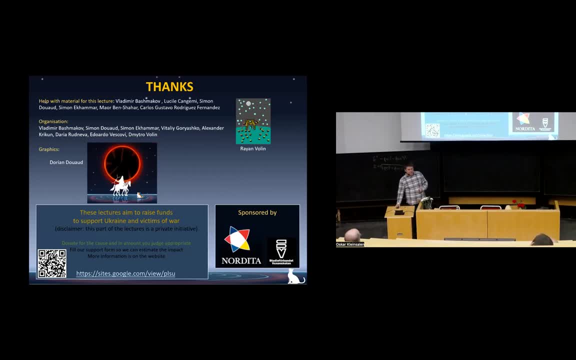 To prepare it. So this one says about this picture. So this actually pixel art picture and this a small ants who are doing observatory. So there are many people who helped me to create these slides. Thank you to all of them. And likewise, thousands of people were building LHC. 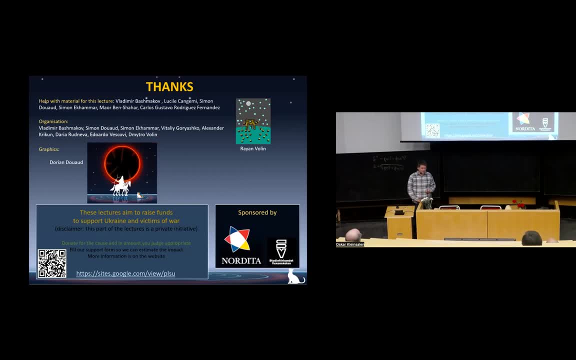 to achieve the heat that we have today. And the last thing- there was a reason behind this lecture is: we aim to raise funds, So please consider doing this and look at our website. We have information about this. Thank you, It's no good time for questions. 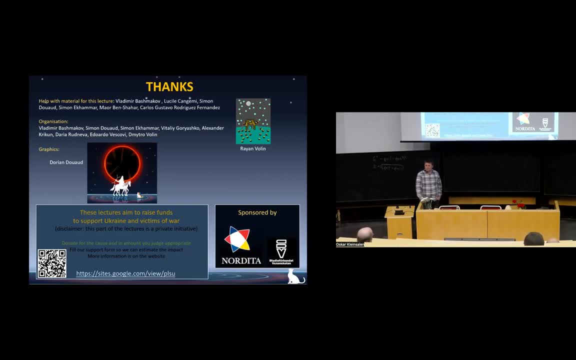 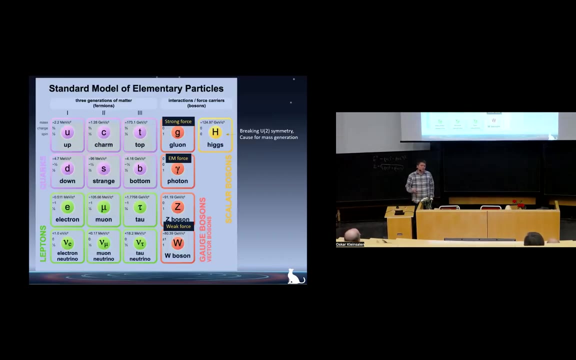 Or we have another question: The web is still closed. Well, To make it short, for this means that at least told them: have us. So you have to update this model. So one was камера proposal. is some lives Close? 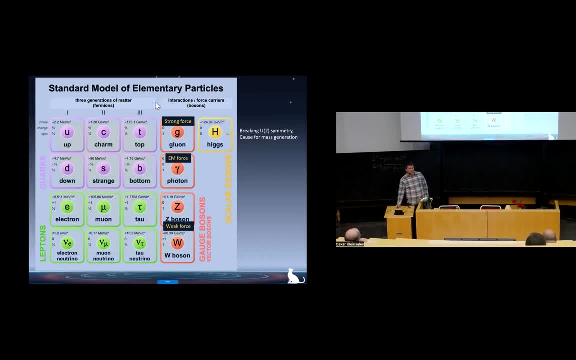 outside of this table there is a force, very, very heavy neutrino or something like this, and it's slightly mixed with these three guys which make this light mixture. it's massive. well, i mean, yeah, we need to make small update of the table, but i suppose people write articles about this but there is no like standard. 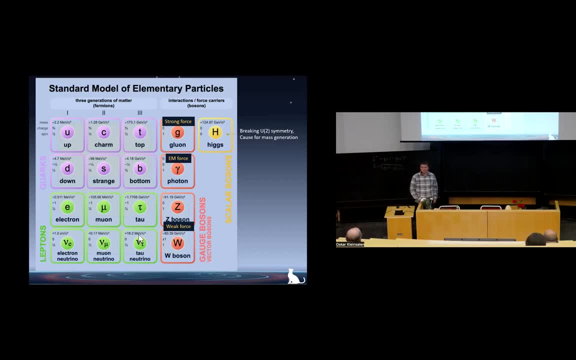 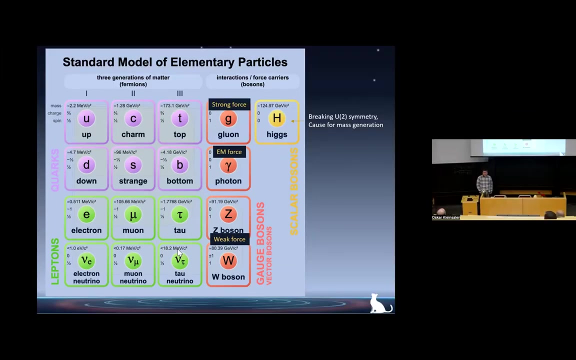 uh, think about this yet, otherwise you will know it about it, but we don't. so i would suggest a homework exercise. given this number of quarks, try to calculate the number of baryons which you can make out of them. so i would suggest a homework exercise. given this number of quarks, try to calculate the. 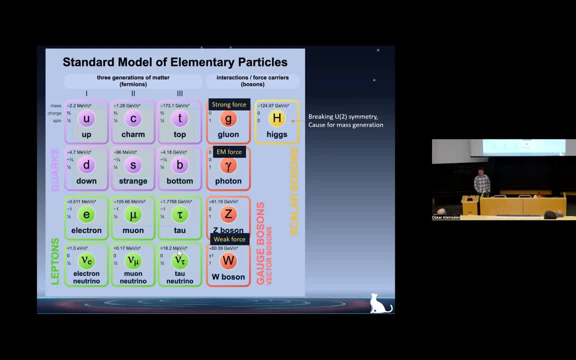 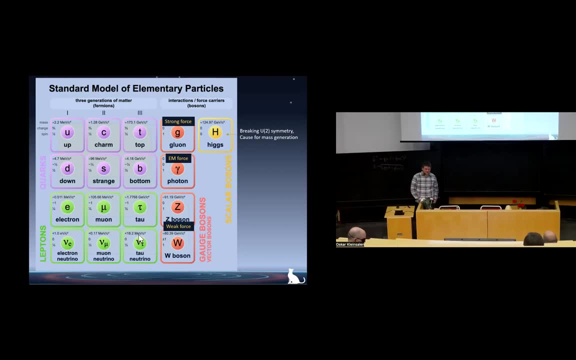 number of baryons which you can make out of them. so i would suggest a homework exercise. given this number of quarks, try to calculate the number of baryons which you can make out of them and check how many baryons have not been discovered yet. 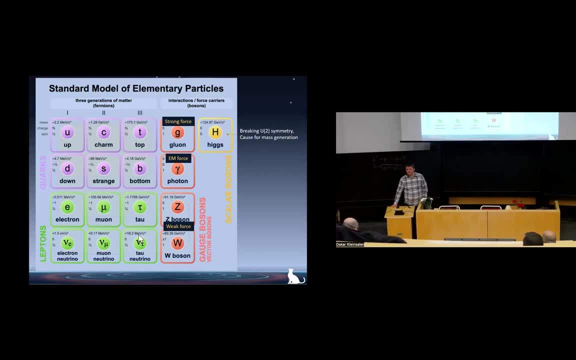 we have some of you might be probably right in the chat. we have some of you might be probably right in the chat. we have some of you might be probably right in the chat. yeah, there are no questions. yeah, there are no questions. yeah, there are no questions. oh, 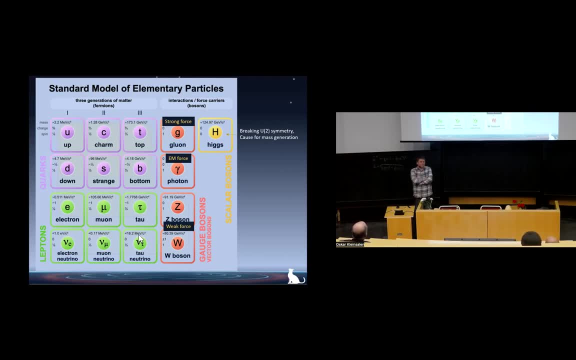 i wonder actually, before i forgot i can switch on machine. before i forgot i can switch on machine. before i forgot i can switch on machine if you want to look, if you want to look, if you want to look. electron emission. i did not notice that electron emission. i did not notice that. 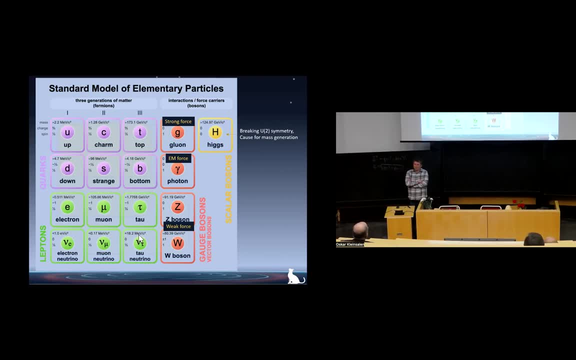 electron emission. i did not notice that it's already very late. Last time I looked, the clock was still before 8.. Yeah, we have raised hands in Zoom, but I don't know how to make Zoom participants speak now. No, let me try.